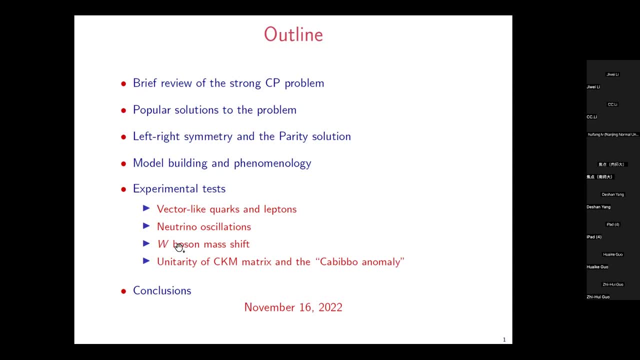 that are around these days, such as the W boson mass shift and that is measured by the CDF collaboration recently, and the potential non-unitarity of the Kobayashi-Maskawa matrix, sometimes called the Khabibov anomaly. This setup is rather constrained. One cannot take the model and solve the strong CP. 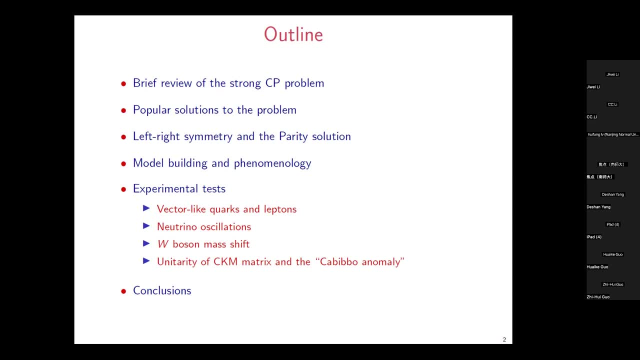 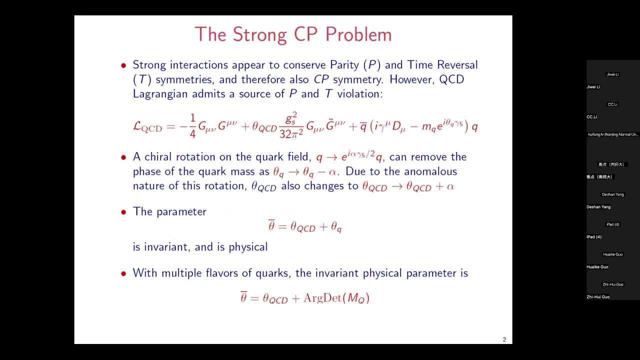 problem and also explain various other anomalies. I will explain why some of the other anomalies cannot be explained within the context. but these two fit very well with the idea of left-right symmetry and solution to the strong CP problem. Then I will conclude: Okay, so here is a very brief summary of what the strong CP problem is. 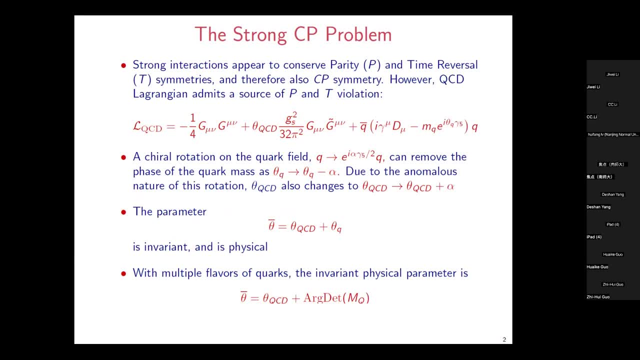 The strong interactions appear to conserve parity symmetry as well as time reversal symmetry. This is unlike weak interaction which breaks both parity symmetry and time reversal symmetry If both P and T. if time reversal symmetry is broken, then because of conservation of CPT, CP symmetry would be also broken. But in the strong interaction, 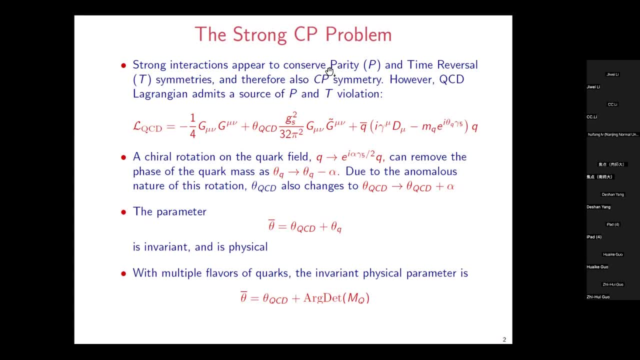 CP symmetry seems to be well preserved. However, if you look at the QCD Lagrangian, there is a source of violation of parity symmetry, as well as time reversal symmetry or, equivalently, CP symmetry. So here is the QCD Lagrangian with one flavor of quark. 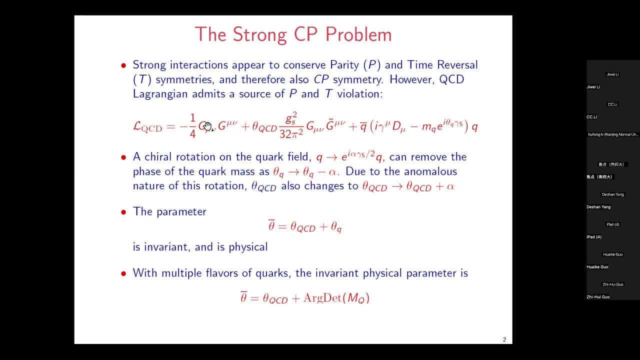 So here is the field strength. This is a gluon field strength. So the kinetic energy of the gluon is the first term And this term here, theta QCD times gluon field, times the dual gluon field. this is a term which would, if it remains in the Lagrangian, it will, violate parity symmetry. 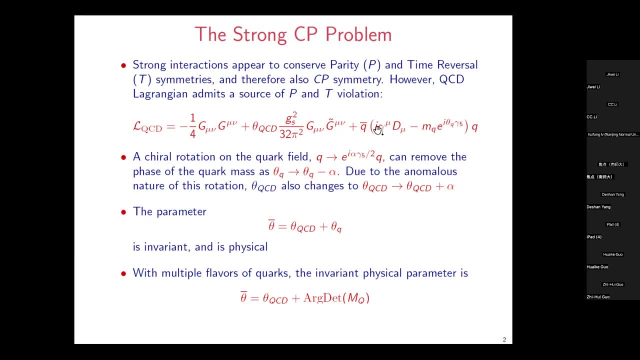 It will also violate CP symmetry. And then we have the gauge interactor kinetic term for the quark field and a mass term for the quark field. And the mass term here has been written. it is in general complex, So that can be written in this fashion: a phase E to the i, theta, Q times gamma phi. 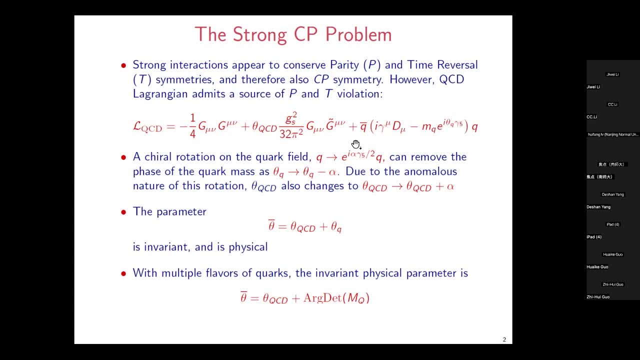 Now, if you look at this, we can get rid of the. Whenever there is a space in the Lagrangian, that is some signature of CP violation. But the phases don't always always remain after field redefinition. the phase in the quark mass term can be absorbed. 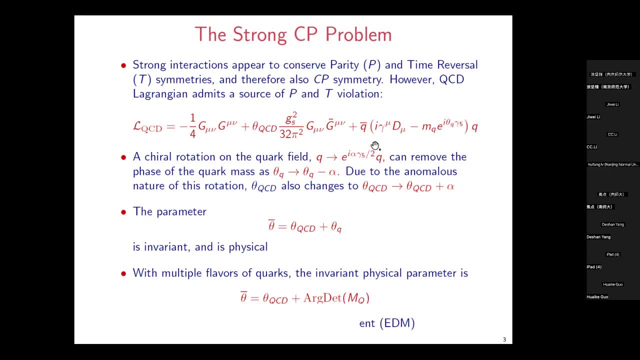 by a field rotation e to the i- this is a chiral rotation of the quark field and with this by e to the i alpha gamma 5 over 2 times the quark field and one can if we do that. 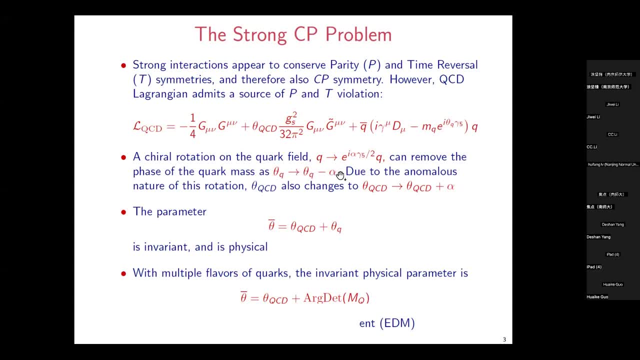 the theta q will go to theta q minus alpha, And one can choose alpha appropriately to get rid of the quark mass phase if needed. However, the rotation that is needed to get rid of this is a chiral rotation. It has an anomaly associated with it And this term 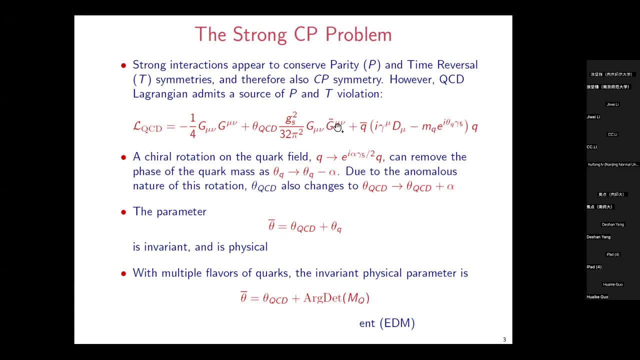 here the second term, g times g dual, is actually something related to the anomaly coefficient. So when you get rid of the phase of the quark mass term, it will appear in the theta qcd term. What happens is that theta qcd is not an anomaly, it is an anomaly. So when you get rid of the 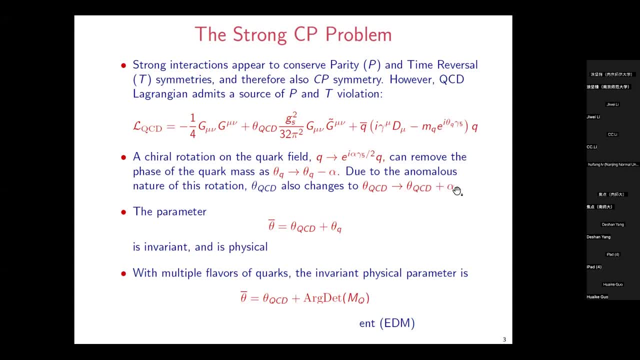 QCD will go to theta QCD plus alpha in such a way that this combination, theta QCD plus the phase of the quark mass term. it does not, it is invariant And this turns out to be a physical parameter. So there is therefore a physical parameter in the QCD Lagrangian. 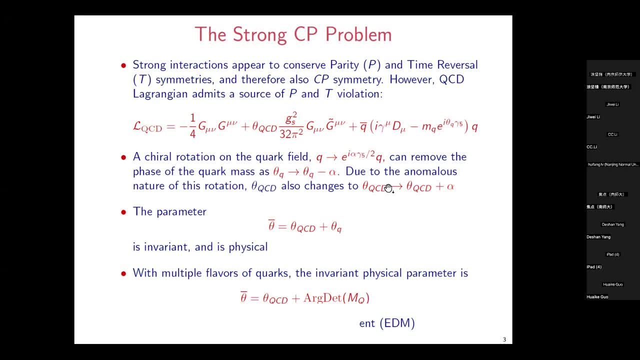 that violates time reversal symmetry as well as parity symmetry. If you look at multiple, this was for the case of a single flavor of quark field. one can generalize this to multiple quark fields And if you do that, what happens is that the theta bar becomes the QCD part. 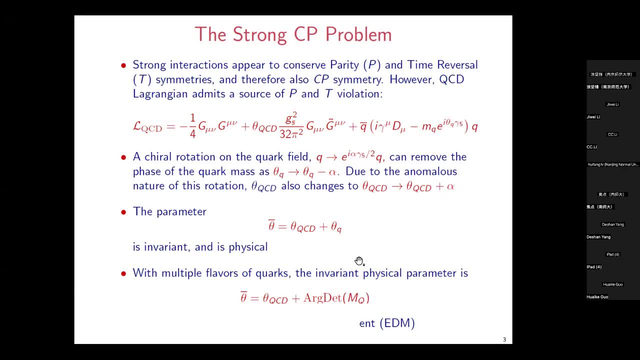 plus the argument of the determinant of the quark mass matrix. Okay, So this theta Q becomes right, The phase of the determinant of the quark mass matrix. Let me see This: if the QCD Lagrangian has this physical parameter, theta bar, 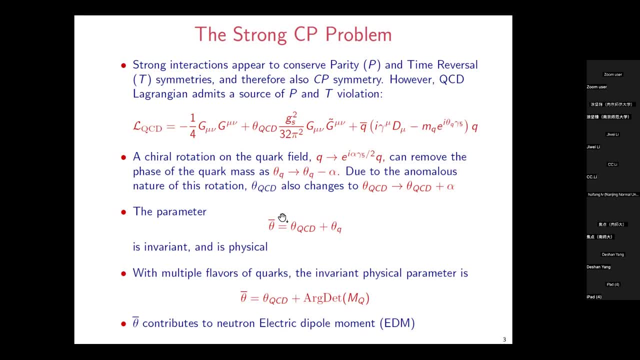 it would contribute to the electric dipole moment of the neutron. As you all know, the permanent electric dipole moment of elementary particles is a signal of CP or time reversal violation, And the neutron does not seem to have any electric dipole moment There are. 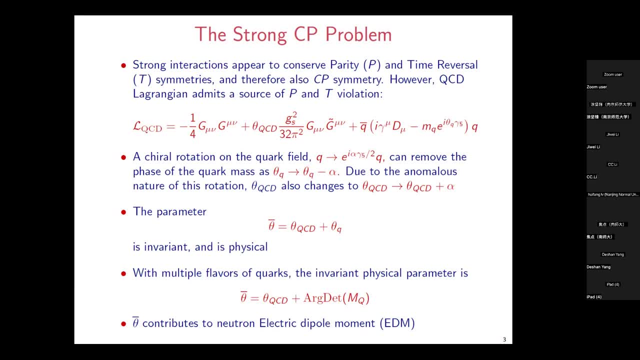 there have been concentrated experimental efforts to measure the electron, the neutron electric dipole moment. It has not seen anything. This is a strong indication that the strong interactions are conserving time: reversal and CP symmetries. So how does that neutron electric dipole moment? 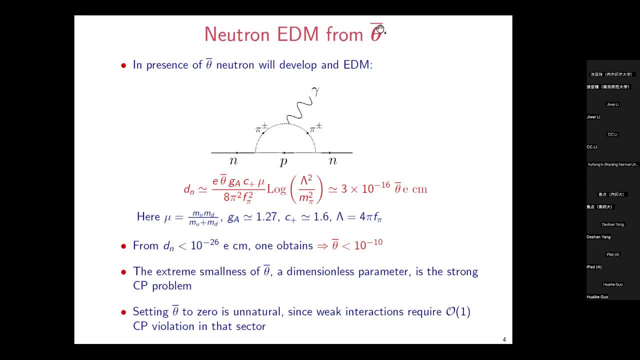 arise. We must be careful that at this constant variation we do not cost rotation the irreversible Dirichlet of Karlsruhe. allest in the pos registered Los Angeles research that neutron is the洗 siglycott Okay of the neutron, and it is estimated in chiral perturbation theory to be the expression given. 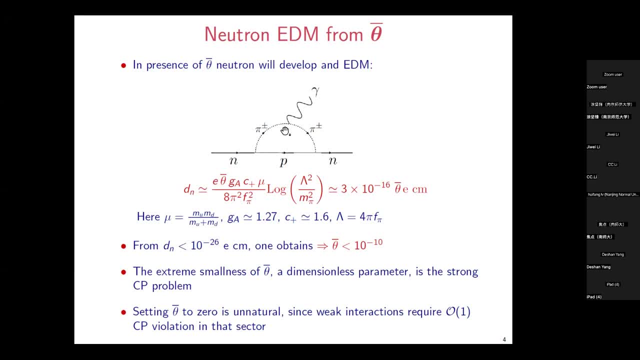 here. It is proportional to the electric charge, It is proportional to theta bar, because that's the source of CP violation. GA is the axial vector coupling of the nucleon and C plus is some order one coefficient which is obtained from chiral perturbation theory, and F pi is a pi. 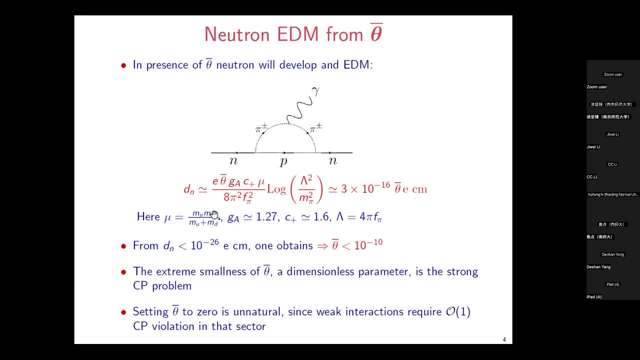 constant. It is also proportional to a parameter, mu, which is this quantity mu md divided by mu plus md, and the cutoff scale here is provided by the QCD scale for pi times m pi. If you put in all these numbers, we see that neutron would have an electric dipole moment of order 10 to the minus. 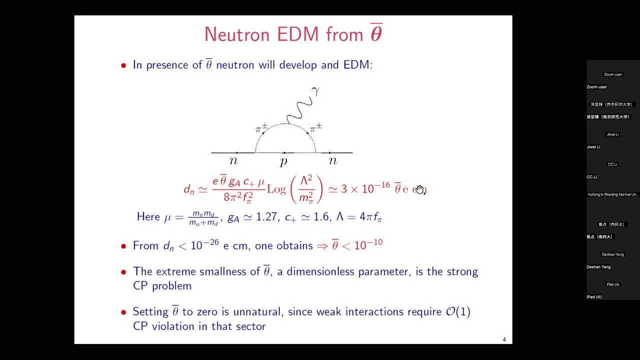 16 times this theta bar in units of e centimeter. Now neutron electric dipole moment. there is an experimental limit on the neutron electric dipole moment which is 10 to the minus 26 e centimeter. When you compare these two, 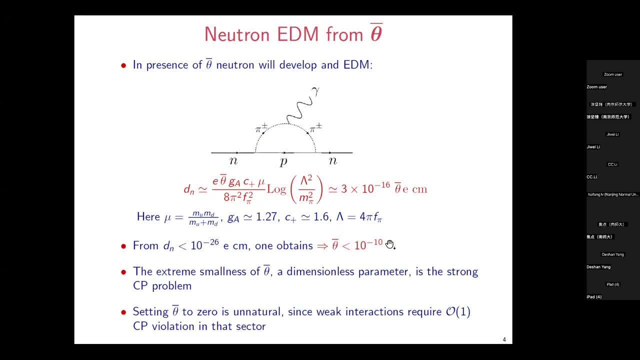 we see that theta bar has to be less than 10 to the minus 10.. Now this causes a problem. Theta bar is a dimensionless parameter in the QCD Lagrangian, and the puzzle is: why is it that a dimensionless parameter in the Lagrangian is so tiny? 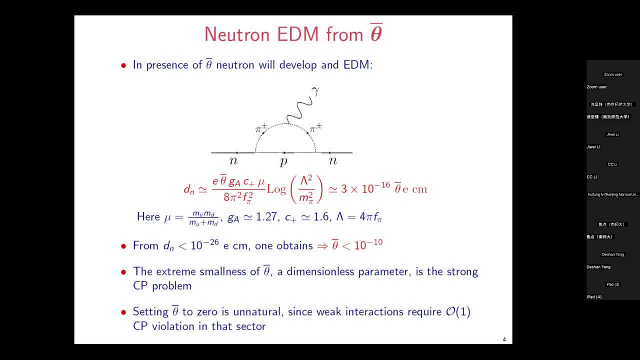 That is the strong CP problem. Another way of stating is that: why is QCD CP conserving? Why is the neutron electric dipole moment so tiny? These are all related questions. One might consider putting theta bar to zero just to, because it breaks a certain symmetry. So 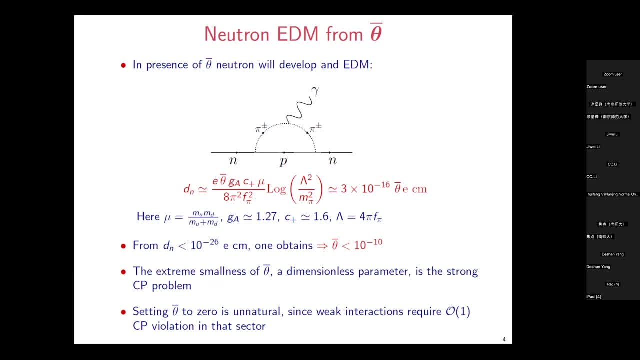 if the symmetry of the Lagrangian is enhanced by setting certain parameter to zero, that is a good explanation. But that is that is not a good explanation. So if the symmetry of the Lagrangian, in this context it is not a good explanation because we have one Lagrangian, the standard. 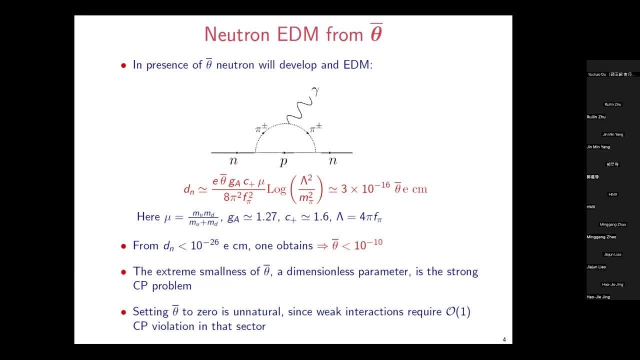 model Lagrangian, which has weak interactions as well as strong interaction, And we know for sure that the weak interaction break the CP symmetry in some last way. The Kobayashi-Maskawa phase in the CKM matrix is of order pi over three or something. So on the one hand you have an order. 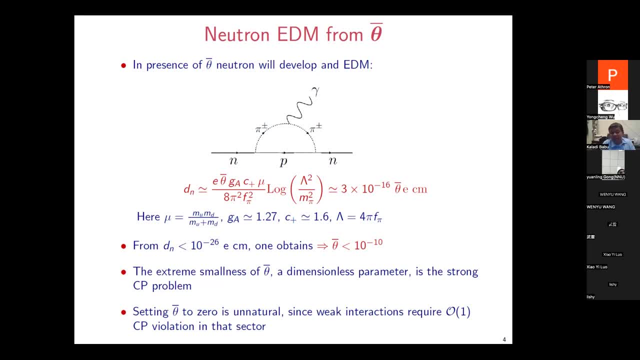 one CP violation and then in weak interaction and the CP violation in strong interaction is allowed to be theta bar, to be a four or one. That would have been the most natural scenario, But we know experimentally that it has to be less than 10 to the minus 10.. 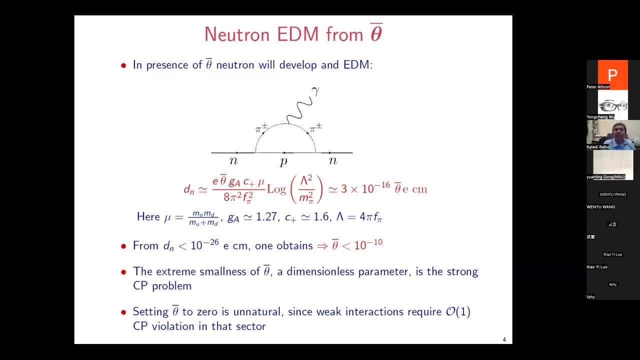 So that neutron limit on the neutron electric dipole moment provides a well-defined problem of the standard model Lagrangian, which is the strong CP. Okay, If there are any any questions, I welcome interruptions and I will be happy to address it as we go along. 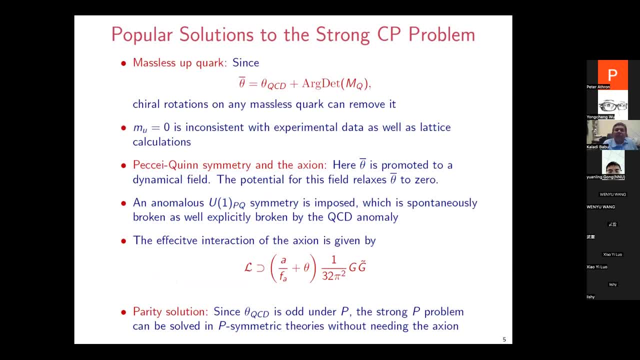 Okay, Let me move on. This is a summary of popular solutions to the strong CP problem. I have listed three solutions here. One is the idea that one of the quarks is. the mass of one of the quarks is zero And the leading candidate is the lightest of all the quarks, which is the 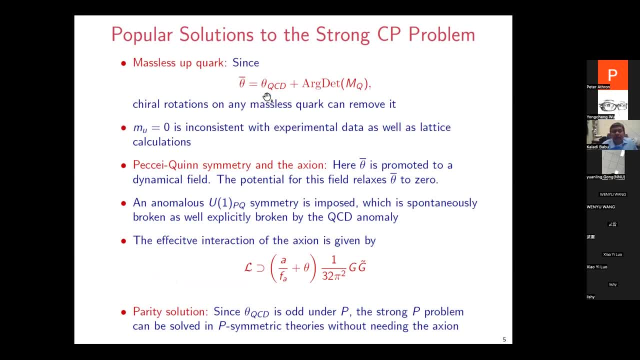 up quark, Since theta bar is equal to theta QCD. plus this argument determinant of the quark mass matrix, one can, if one of the quark masses is zero, one can make a chiral rotation to remove, remove theta bar entirely from the Lagrangian. So if, experimentally it were, 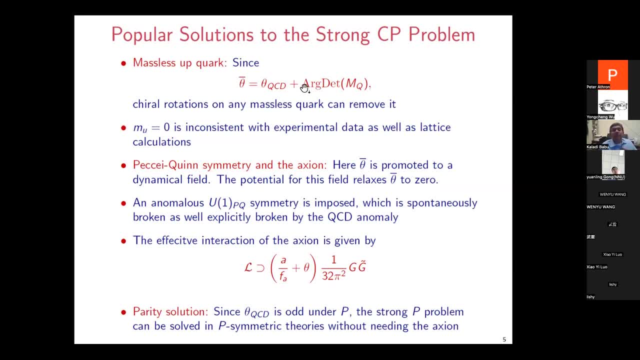 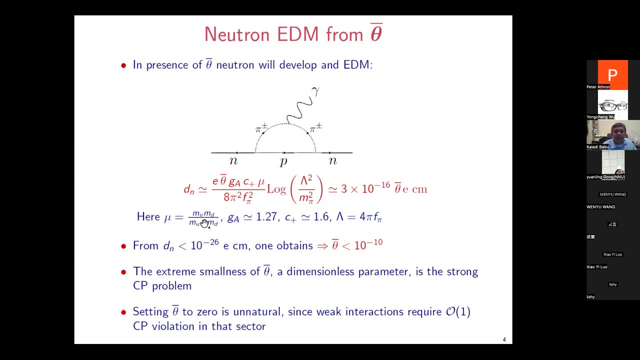 consistent that the up quark mass is zero, then there would not have been a strong CP problem. Okay, And you can also see that from the previous slide. see the mu parameter in the estimate of neutron electric dipole moment. it is proportional to the light quark mass If up quark mass is set. 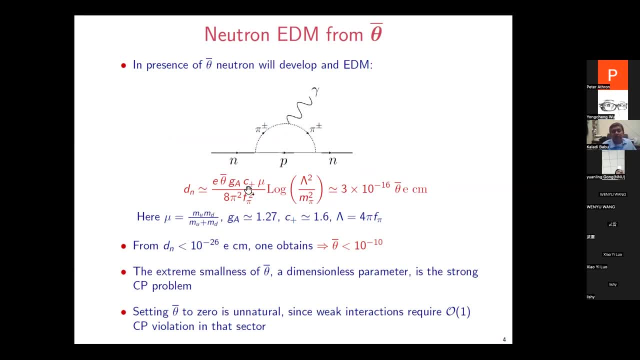 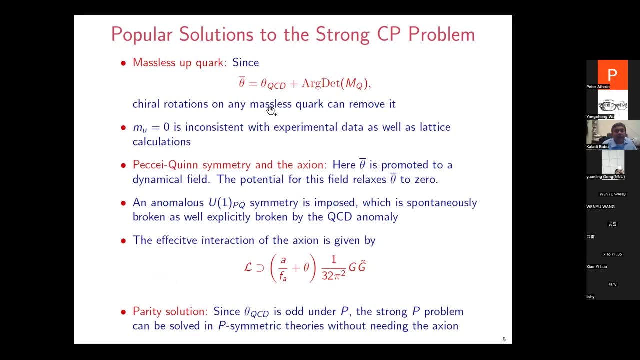 to zero. there is no electric dipole moment. So it is manifestly shown in this chiral perturbation theory estimate of neutron EDS. Okay, But there is an unfortunate inconsistency with experimental data. Up quark mass is not zero. It is measured to some value, a few MeV, And this is confirmed by 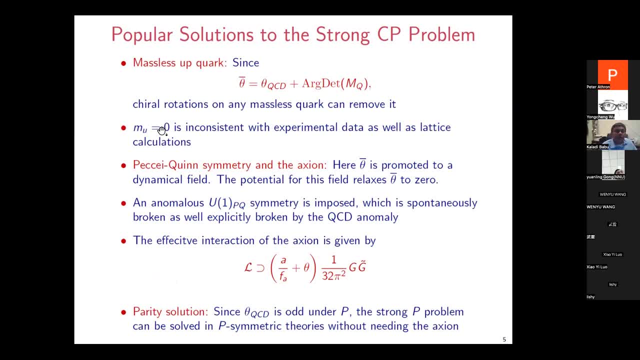 precision lattice computation. So this solution, although theoretically would have been an acceptable solution, it is not realized in nature. Okay, The most popular solution to the strong CP problem is the pitch-eye quincemetry and the resulting axion. What happens here is that this theta 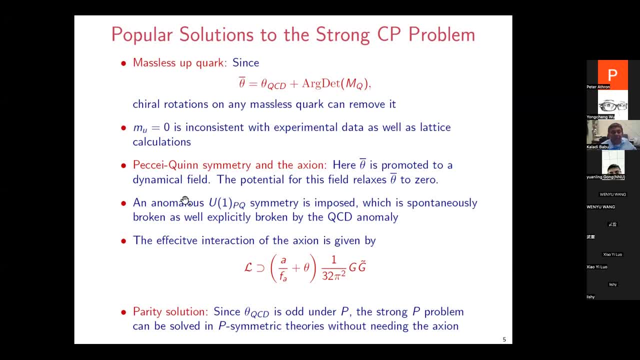 bar parameter is promoted to a dynamical field. So this dynamical field, which is a scalar field, has a potential And when we minimize the potential, theta bar would be relaxed to zero in the ground state. That's the basic idea of the pitch-eye quincemetry, solving the strong CP. 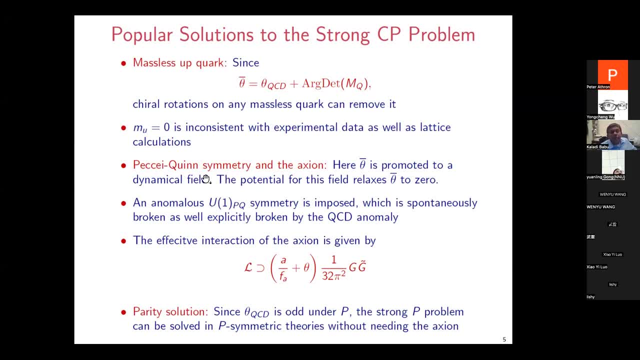 problem. So here, what one does is we assume a global symmetry called U1 pitch-eye quincemetry on the Lagrangian. This global symmetry is a global symmetry on the Lagrangian. This global symmetry is good everywhere except for one thing: It has a QCD anomaly. So the anomaly of the QCD interactions. 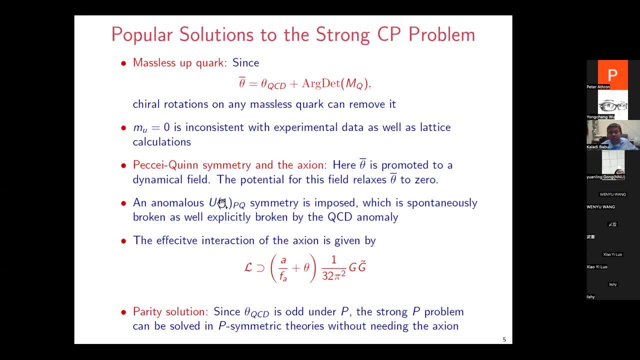 breaks the symmetry explicitly, but otherwise it is only spontaneously broken by the scalar field, acquiring vacuum expectation value. Now, if the only source of breaking is the spontaneous breaking, there would be a Goldstone boson, a Nambu Goldstone boson associated with the U1 symmetry breaking. 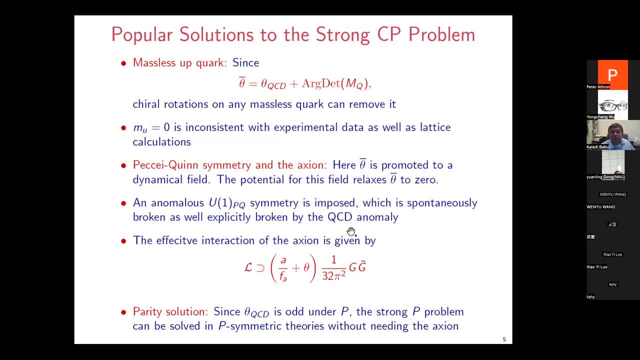 And that would be exactly massless. But in fact, the U1 symmetry breaking would be exactly massless. However, the QCD anomaly actually means that the symmetry is not exact. Through the QCD anomaly, the axion will pick up a mass And all its interactions can be. 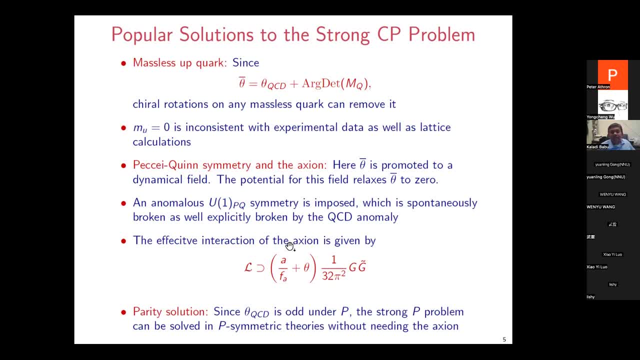 expressed in terms of this effective Lagrangian A. here is the axion field and the associated decay constant. This is F. A is the associated axion decay constant, which is typically of order 10 to the power of 1.. And this is the associated decay constant, which is typically of order 10 to the power of 1.. 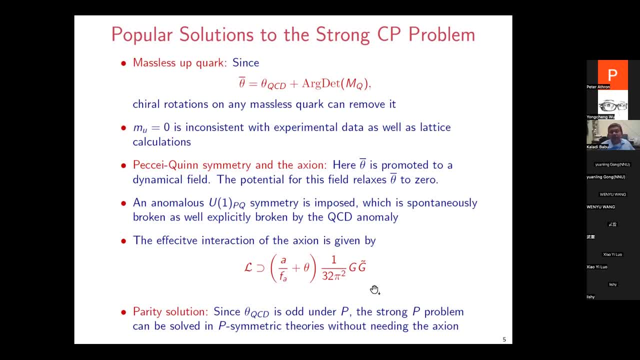 And this here is a class of 2.. Indeed, 1 to the power of 1 is green, But after the offers that QCD scenario in aquarius, the actual position of a mass of give zero non- Stick Sugar actually is equal toelles. So we could, but we're essentially using the distribution system. at the log. and so this is how the axion coupled to the gloom fields. So this is led to a lot of interesting research in especially looking for a light particle. the mass of the axion would be of order milli electron volts, or even smaller. They could potentially be a dark matter candidate, but there are many interesting things that goes with the axion solution to the strong, marvelous culprit picture. AsAM plant cannot reproduceWell, which is seeing Después19.5.1.3.. And therefore that is important to note, that the small CPM process is not biodegradable. You could not use the small swarm — we said 4.. 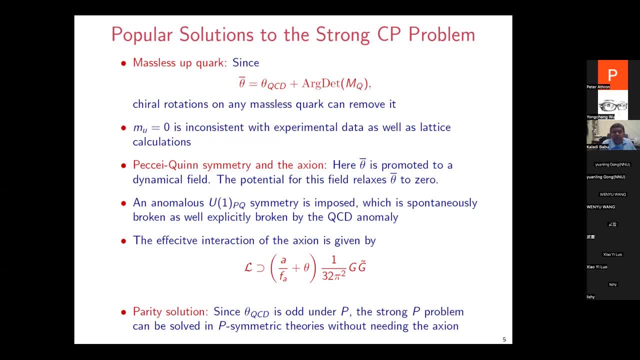 Axion has not been observed. There are also issues about having global symmetries, such as the Pichetkin symmetries, because quantum gravity is expected to break all global symmetries explicitly, And this goes by the name axion quality problem. The axions suffer something. 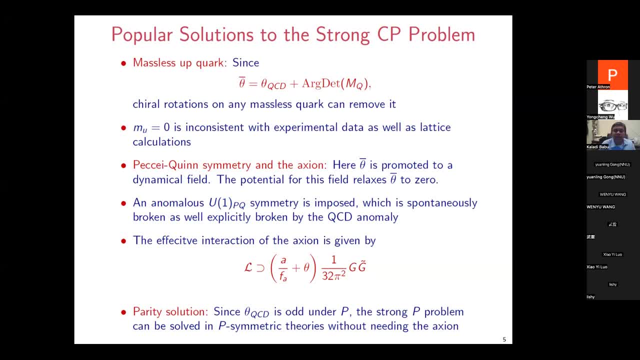 called axion quality problem. In order for axion to be a good solution, the Planck suppressed or gravity-induced breaking of the Pichetkin symmetry should be rather weak. Anyway, apart from that, this is a very interesting solution. A lot has been done in the search for axion. 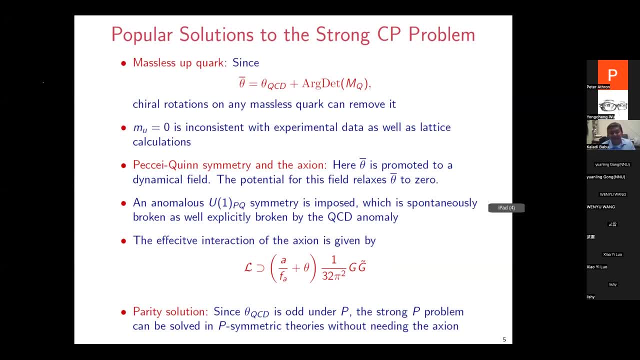 studying the properties of the axion and so on. That's not the focus of my talk. My focus is the third solution, which is the parity solution. I believe it is somewhat underappreciated solution to the strong CP problem. If you look at it theoretically, it is on similar 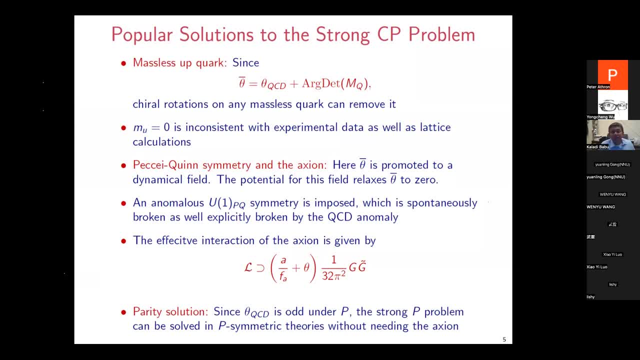 footing as the axion solution. The idea is that since Theta QCD is a parity odd operator, if one can somehow impose parity on the whole Lagrangian and break it spontaneously, then that could potentially solve the strong CP problem without having the axion, So that 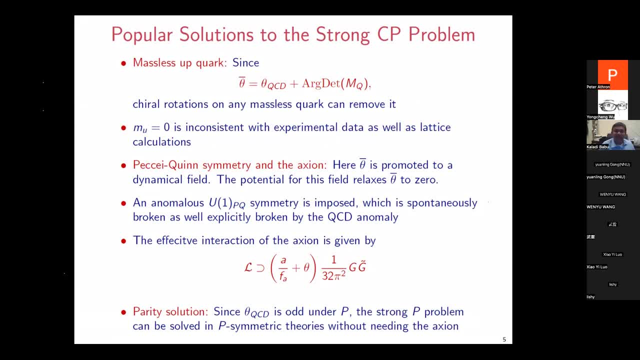 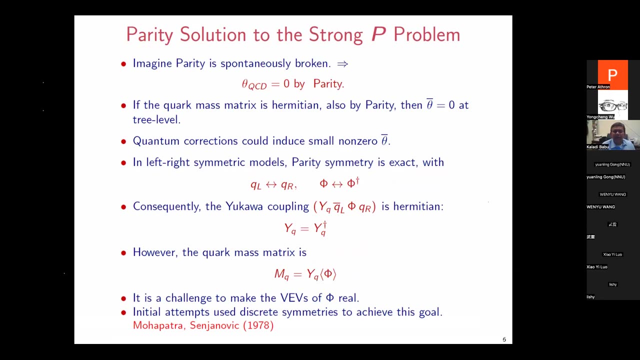 is the remainder of today's talk, Motivation for doing that and some of the models that are built to explain this and some of the experimental parts. Okay, so here is a broad brush outline of the parity solution to the strong CP problem. Imagine you have some underlying theory which is some beyond. 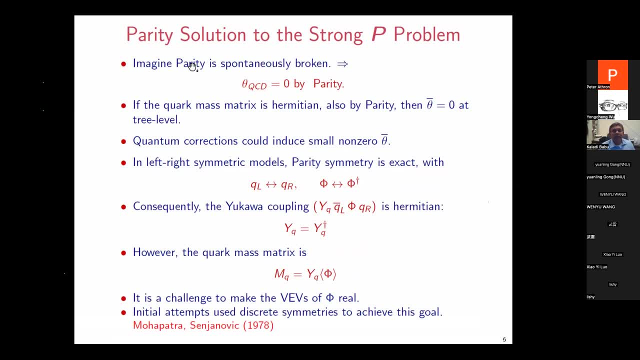 the standard model theory. In that theory parity is a good symmetry and it is spontaneously broken. So because of parity symmetry the Theta QCD should be zero, because it is a parity odd operator. The Theta QCD is the coefficient of the g-g dual term. Let me show that again. 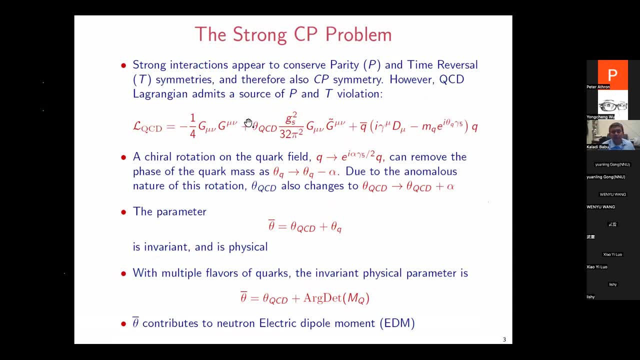 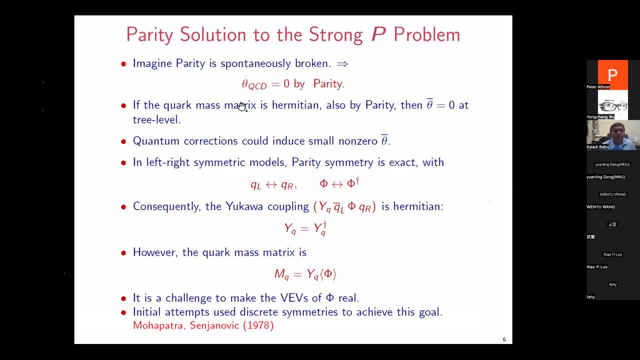 Theta QCD is the coefficient of the g-g dual term, which is parity odd. So, because the theory is assumed to have exact parity symmetry, Theta QCD would be zero. Okay, that's the first condition. Now imagine also that the Quark mass matrix is Hermitian. 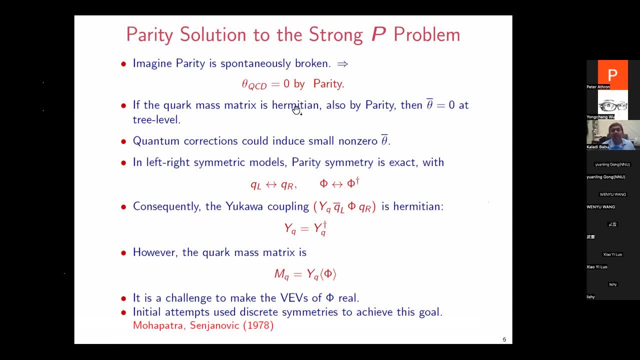 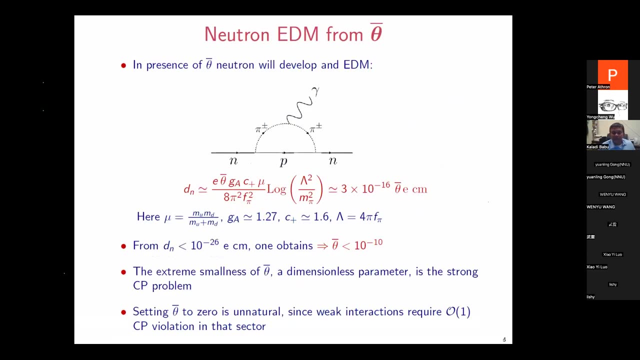 This could be achieved and I will show this in more detail. if it is Hermitian, also by parity symmetry, then Theta bar is zero, because Theta bar is a combination of Theta QCD and argument determinant of the Quark mass matrix. Where is that? Yeah, Theta bar is Theta QCD. 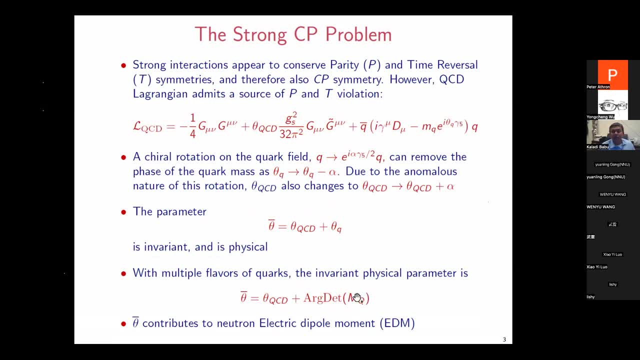 plus argument: determinant of the Quark mass matrix. What is that? Yeah, so this is the determinant of the quark mass matrix. If quark mass matrix is Hermitian, the determinant will be real and therefore the argument determinant will be zero. 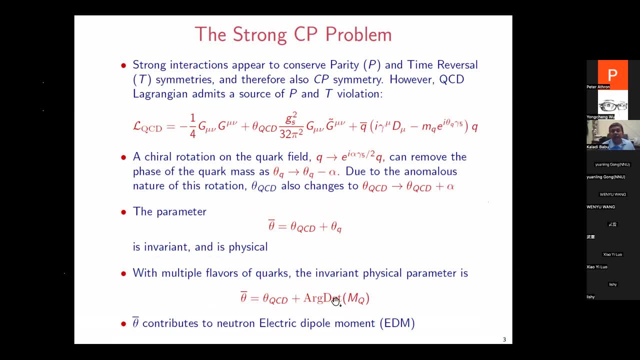 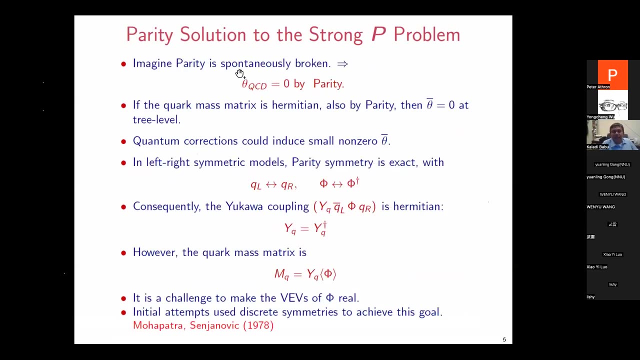 Therefore, theta QCD is zero by parity symmetry. Argument determinant of the quark mass matrix is also zero because the mass matrix is Hermitian, again due to parity symmetry. Okay, back to this. So this is the broad brush outline of the parity solution. 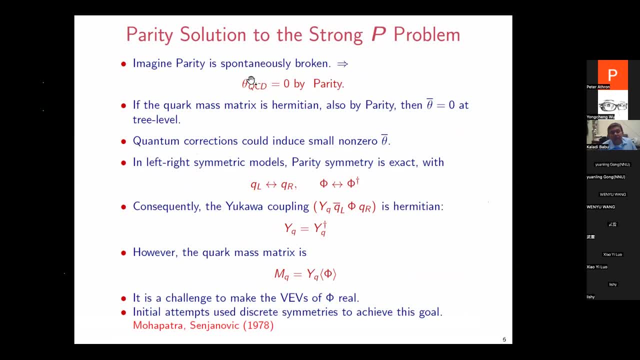 Now. so what this guarantees is that theta bar is zero at tree level. It does not guarantee, because parity symmetry is not a good symmetry. It has to be spontaneously broken, So through quantum corrections, theta bar will be induced. Now, potentially, this quantum corrections? 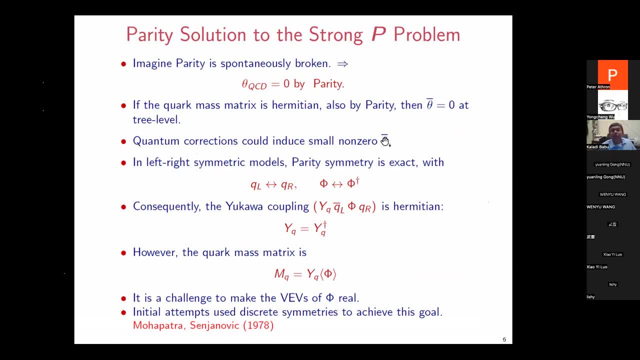 would be small enough so that this induced value of theta bar is consistent with that constraint that arises from neutron electric diagram. Okay, so that's a general idea. So in order to impose parity as a good symmetry, we have to modify the standard model. 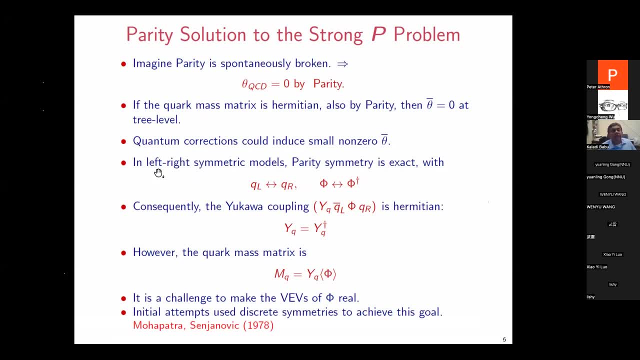 so that parity can be well-defined, And the leading candidate for that are these left-right symmetric models. I will explain that in more detail. In these models, parity symmetry is exact, As the name suggests, under left-right symmetry or under left-right parity symmetry. 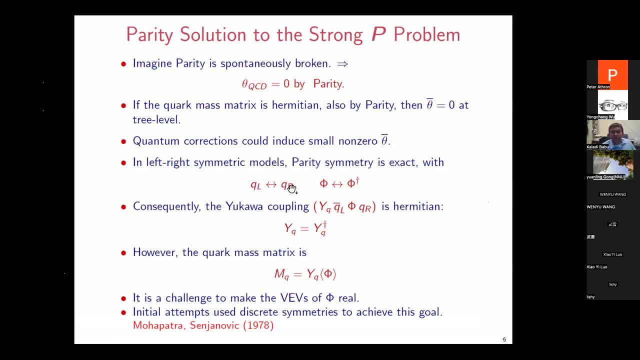 the left-handed quark fields. the left-handed quark fields transform into right-handed quark fields And the field. there is also a scalar field, denoted here as phi, which generates the mass matrix for the quark field And under parity symmetry. 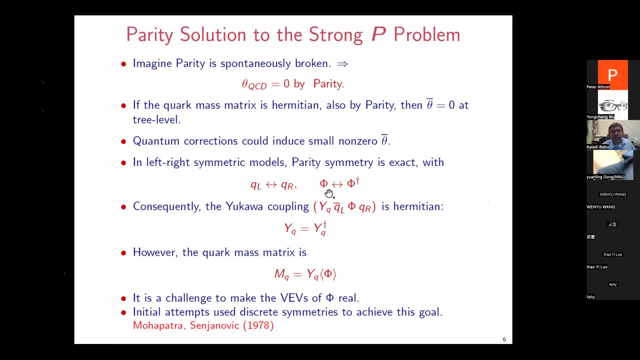 this phi goes to its Hermitian conjunct. As a result, the Yukawa interactions, which is written here: QL, bar, phi, QR, with a Yukawa matrix, y quark. if you impose parity symmetry, then it requires the yq to be Hermitian. 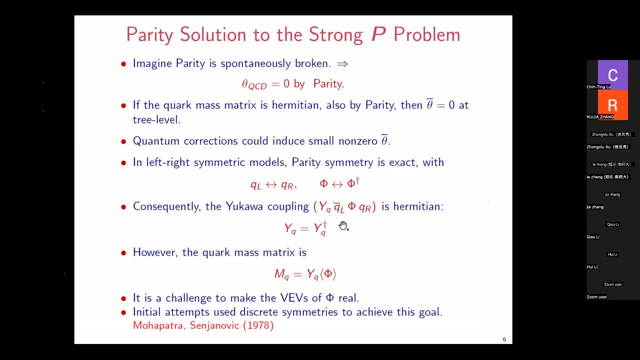 yq equal to yq dagger. I should point out that this is something that, in order to impose this condition, you have to go beyond the standard model. In the standard model, there is no way to impose the Yukawa coupling matrices of the quarks to be Hermitian. 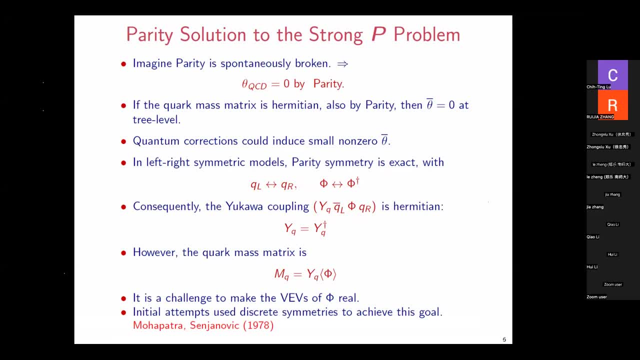 Even if we imposed it to be Hermitian at some level, at some scale, it is not going to be stable. It is going to be stable under renormalization because parity is explicitly broken in the standard model But in this left-right symmetric models. 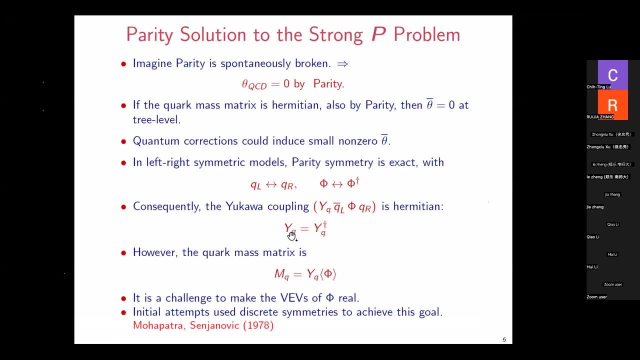 where parity can be defined. this is what you get. The quark Yukawa matrix is Hermitian. Now, that is not the condition that is needed. We need the quark mass matrix to be Hermitian in order to set the Rabat to build. 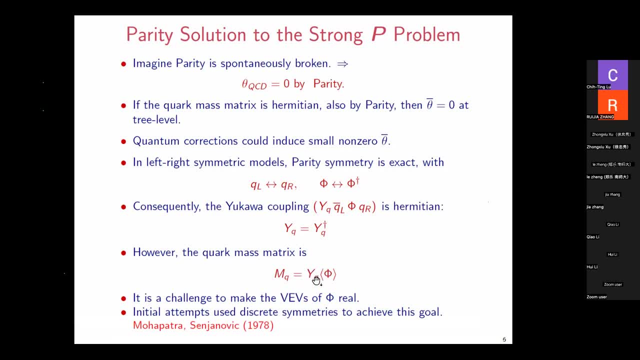 The mass matrix of the quark is given by Yukawa matrix times the vacuum expectation, The vacuum expectation value of the field, which is the equivalent of the it contains the standard model Riggs field. It turns out, and I will again explain this, 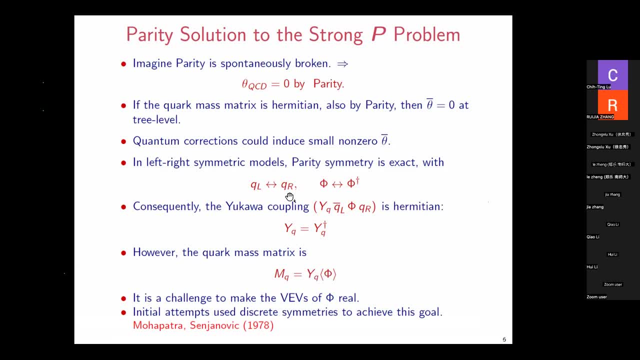 in a bit more detail, it turns out that the parity symmetry makes the Yukawa coupling Hermitian, but it is not enough to make the vacuum expectation value to be real. What is needed to make the Hermitian quark mass matrix is to have 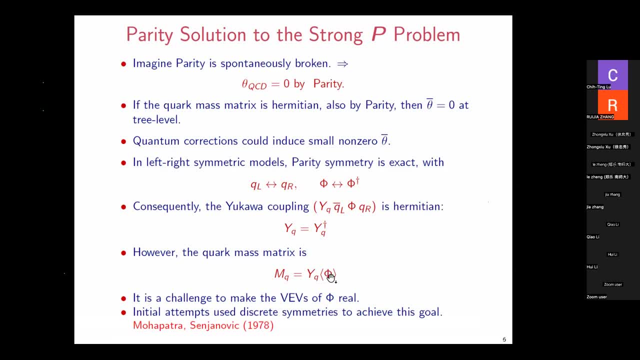 Hermitian Yukawa matrix and real vacuum expectation value. This real vacuum expectation value is a challenge. So initial attempts. for example, this idea was initially. this has a long history: Mohapatra and Sanyana, which is a 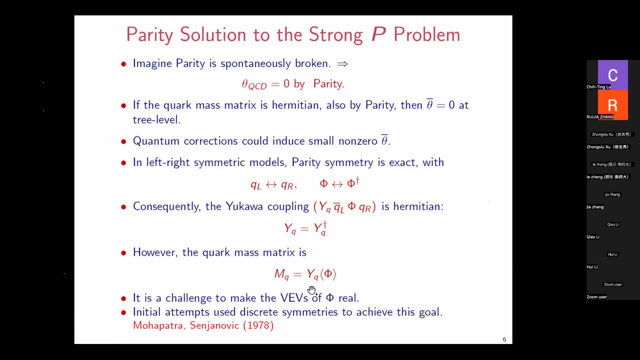 tried to solve it this way, using parity symmetry, And they've realized that because of this issue that the vacuum expectation value tend to be complex, It was sorted to additional symmetry outside of parity with a goal of making the vacuum expectation value real And there were some somewhat of a successful attempt. 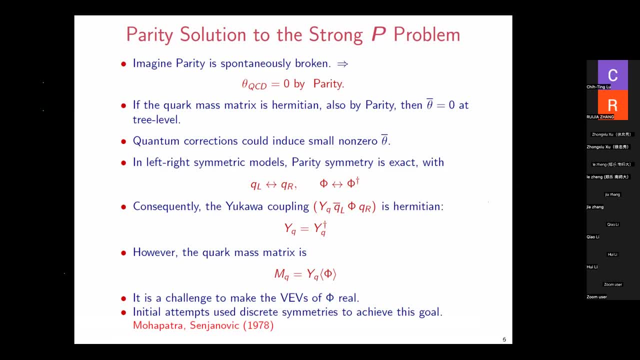 but not completely satisfactory. So it was a parity plus something else. But if you look at the theta bar term, it's really it's a parity odd operator. It would be nice to have parity alone as the solution to the strong CP problem. 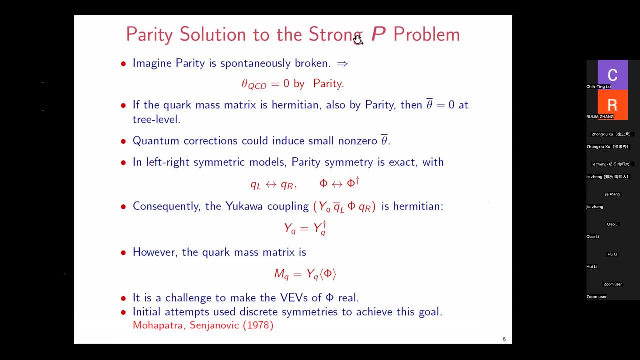 By the way, I should also say that my call here strong parity problem. It is just a historical coincidence that we call it strong CP problem, because in the standard model parity is kind of a maximally broken symmetry. CP is at least in the development of the standard model. 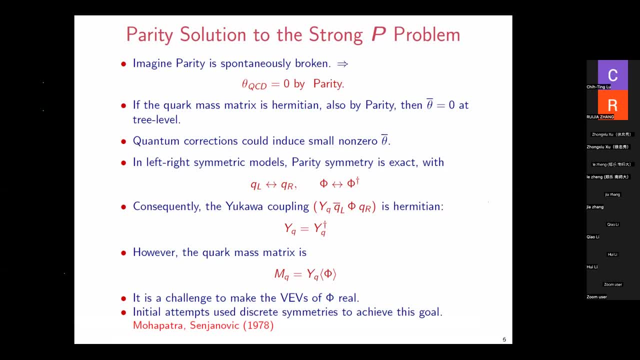 initially CP was thought to be a good symmetry. So there is some intrinsic thinking that it is really a violation of CP symmetry. That is a problem? Obviously that is a problem, But since the theta bar breaks parity, I could have also called it the strong parity problem. 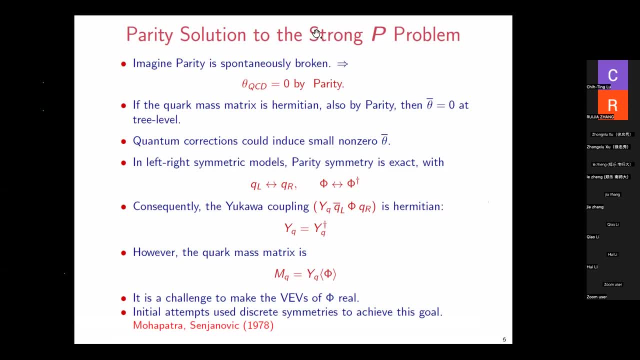 So in some of my slides, instead of calling it strong parity, strong CP problem, I will indicate it as strong parity. That's what I have noted there. Okay, Hello, sorry. Yeah, Professor Babu, yeah, I have a question. 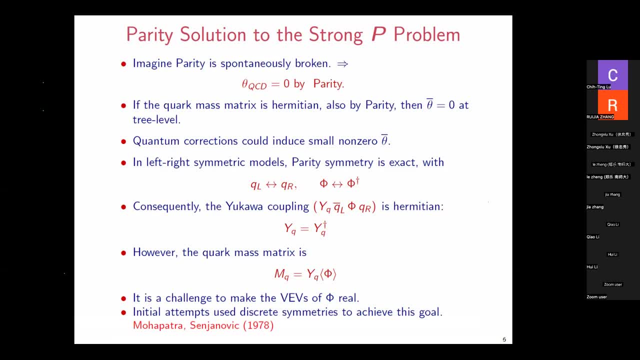 And so in the left-right symmetry model the W on mass is much heavier. It's much heavier than WL, And how does this affect the parity symmetry here? Yeah, this is a very good question. I will actually come back to that specifically. 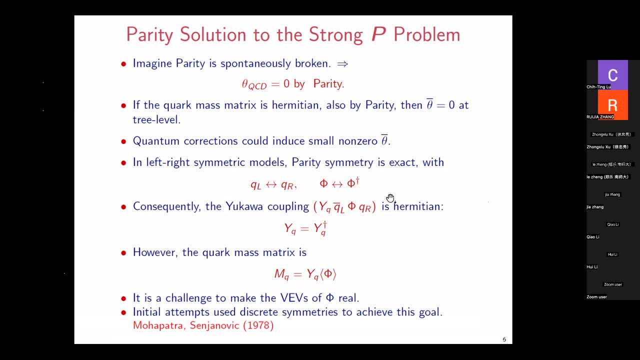 I will have more detailed discussion of left-right symmetry, But you're right that in nature we know parity is broken, right? So this means that in left-right symmetry theory there are additional gauge bosons And at a parity symmetry the usual W boson, the left-handed W, would be. 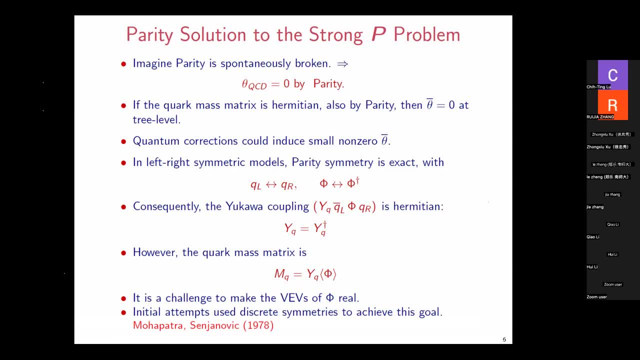 taken to right-handed W. But because parity is broken in nature, the mass of the right-handed W have to be rather heavy, much heavier than the mass of left-handed W, so that weak interactions are maximally parity violating And also there are direct limits from LHC experiments. 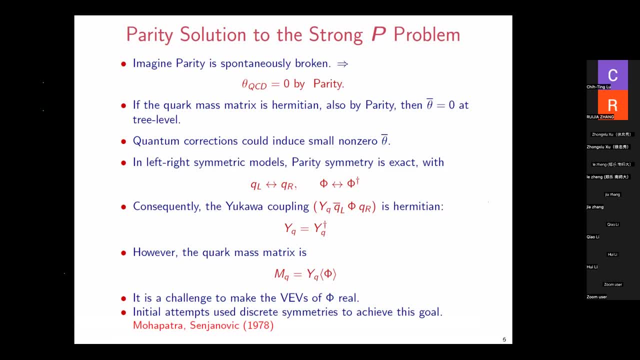 The right-handed W of the standard left-right symmetric models have to be greater than about 40 EV from LHC data. Now this is. this has some effect on this part on the quantum corrections in the induced value of theta bar, But it does not. 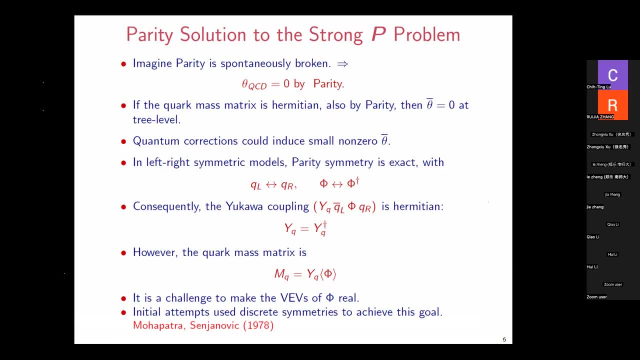 one can still define. because parity is broken spontaneously, one can still define. the whole Lagrangian has this parity symmetry. So one can still solve even though the right-handed W bosons don't have the same mass as the left-handed W boson. 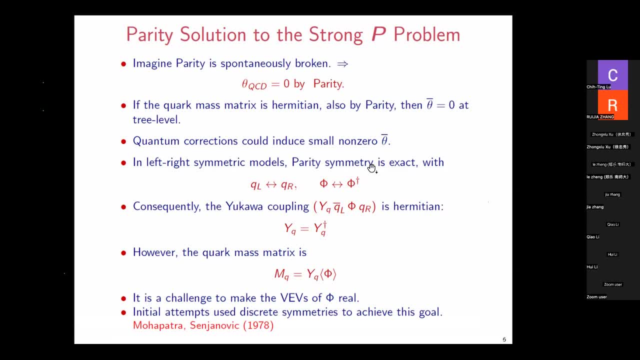 Well, one can define this symmetry. The crucial point is to be able to define the symmetry. Then, if this symmetries are defined, theta QCD is zero, right, Because that is a parity or operate, And the right-handed W will acquire a mass. 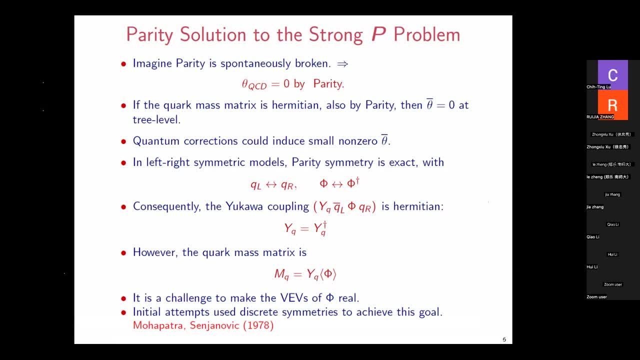 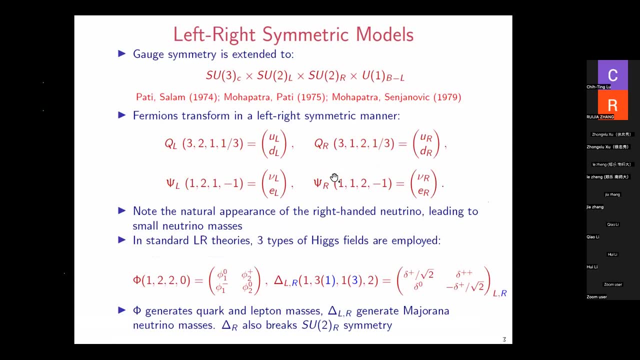 which is very different from the left-handed W, but that doesn't spoil this solution And I will show this explicitly. Okay, I think, yeah, So this is. I'm giving a little bit more detail now. This is, this is the elementary introduction. 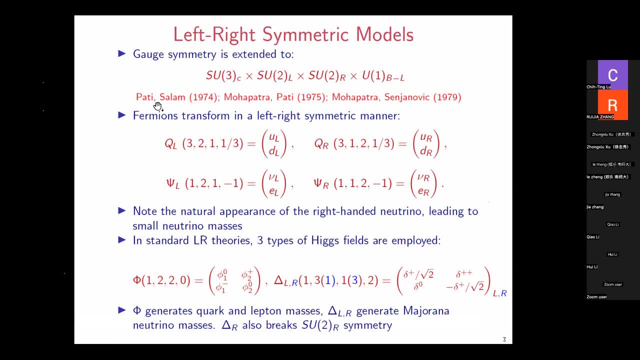 to the left-hand symmetric models. This is the. this was not proposed to solve the strong CP problem. This is, you know when, in the foundational paper by Lee and Yan, which proposed that weak interaction may be parity violating. they already were somewhat. 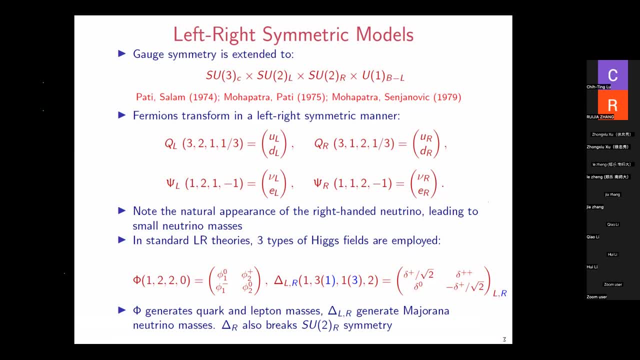 the authors were already somewhat uncomfortable with the fact that we take look at the mirror reflection of our universe. It is different. That's what parity violation is It's telling us. So in the Lee-Yan paper they already proposed the idea that maybe there is some parity. 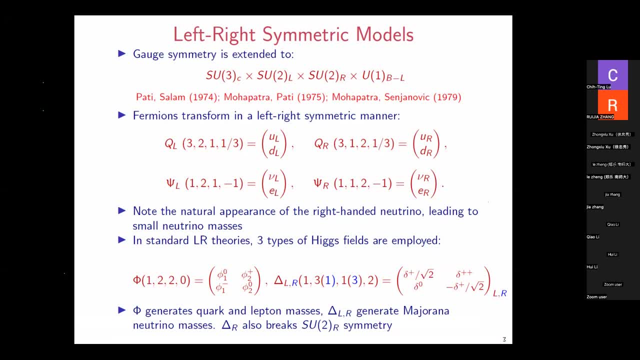 is not really a broken symmetry. Their idea, in modern language, their idea- was to postulate mirror particles. So for proton there will be a mirror proton, for neutron there will be a mirror neutron. And if, if the world is duplicated. 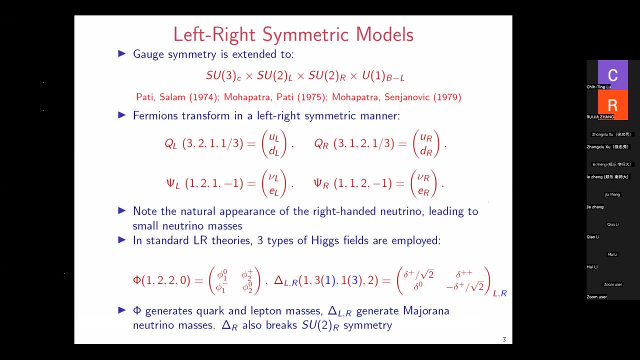 and there is a mirror replica of the world, then one can still, you know, define parity symmetry. This was their idea to reconcile the, the feeling that if you look in the mirror we should do something completely different. These are very uncomfortable to the 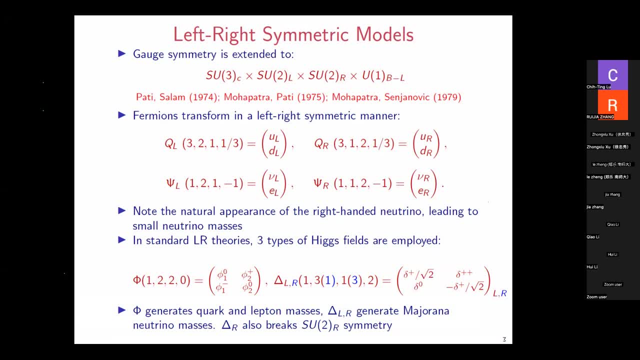 to Lee and Yan. They proposed it And it turns out that that would require a doubling of all the particles that we know. It is an interesting idea. I will not be discussing much about that idea at all. That is a different way of recovering parity symmetry. 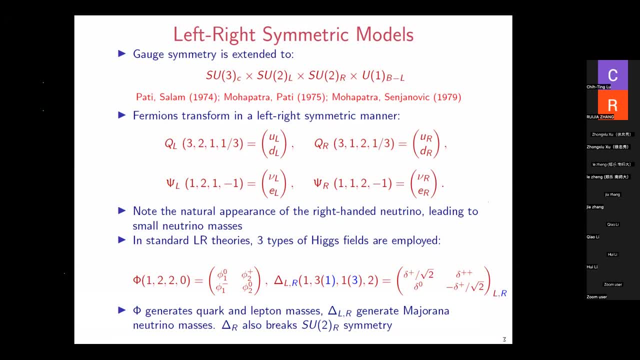 And as far as I know, that does not solve the strong CP property, because there will be a different color SU3 color gauge interaction for the mirror universe, But rather, if you look at this structure, it is only the weak interaction has been extended. 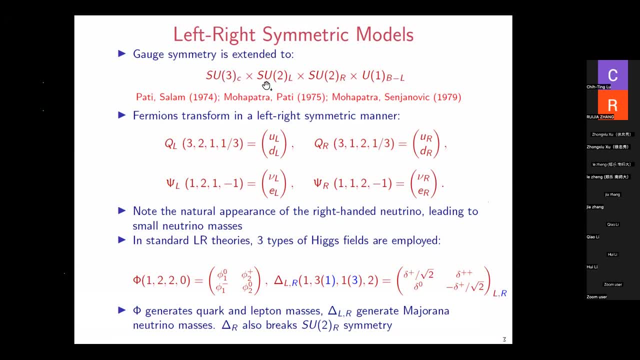 Color is SU3 color of the standard model, but the weak interaction sector is now SU2 left, cross, SU2 right And the U1,. instead of hypercharge, it is now identified as barrier number minus laptop number. So these are the. 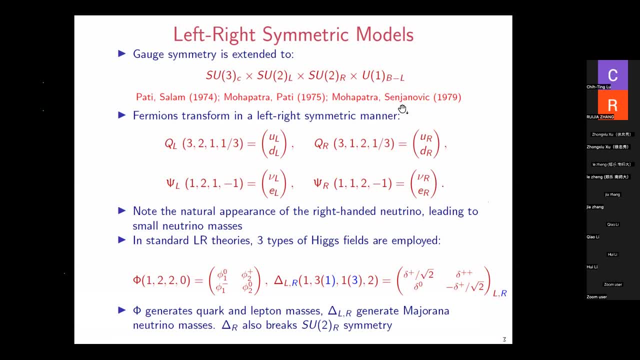 the Pachy Salaam, Mohapatra Pathy and Mohapatra Sanyana, which they they developed this idea, And the idea is that, well, it's much more minimal compared to the, the Lee-Yang idea of a mirror universe. 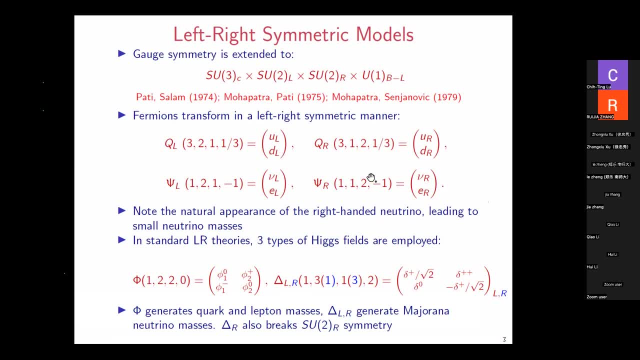 to recover parity invariance. Well, if you look at the particle content, the only new, one new particle is introduced, which is the right-handed neutrino. All of the particles are, say, right-handed quarks, are doublets of SU2 right. 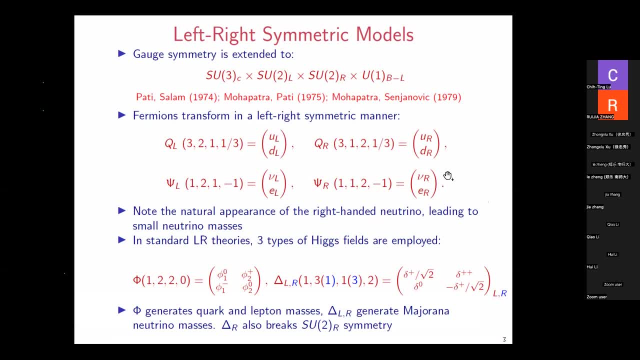 Left-handed quarks are doublets of SU2 left And same with laptop. So they were forced to introduce the right-handed neutrino, which is actually a nice thing. It naturally leads to small neutrino masses through the SISO mechanism, Of course, initially. 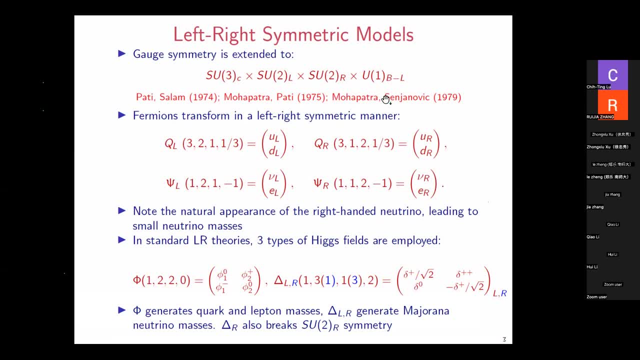 they were not aware of the SISO mechanism, but this paper of Mohapatra Sanyana, which actually showed that it is a natural framework to explain smallness of neutrino mass, because it contains in it right-handed quarks. Because it contains in it right-handed quarks. 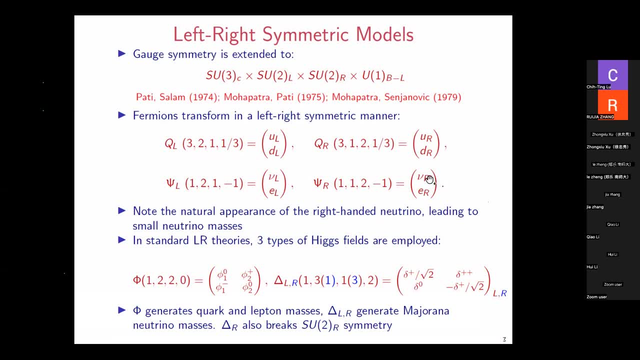 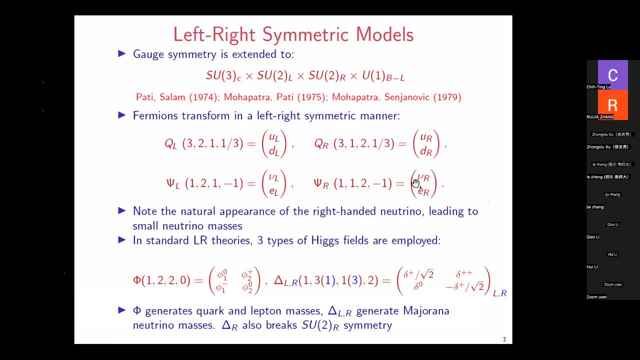 if you have a new L, you must have a new R, So they were forced to have the right-handed neutrino. So, then, neutrino mass is not an optional thing. So well before neutrino masses were discovered, these theories predicted neutrino. 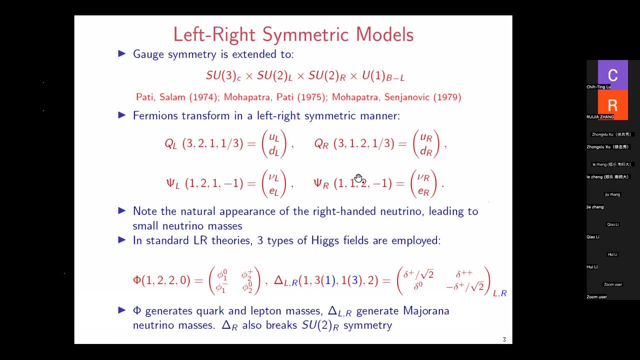 to have finite, non-zero mass. Okay, This is in the so-called standard left-right theories, Two types of Higgs fields are used. This phi field is the one that will generate quark masses and also charged electron masses, QL, bar, QR, phi- that type of interaction. 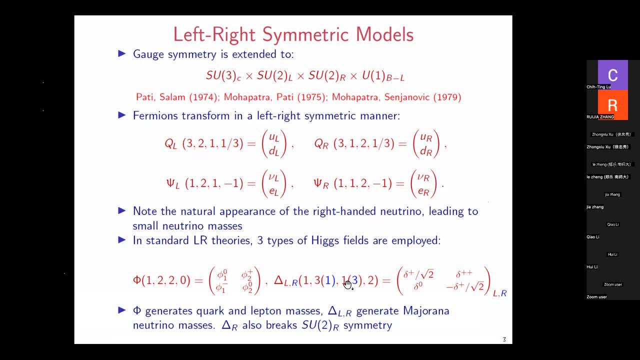 And this delta fields. they generate Majorana mass to the neutrino, both to the right-handed neutrino and the left-handed. There are- I put it in a compact form- There is a right-handed triplet and a left-handed triplet. The left-handed triplet can lead. 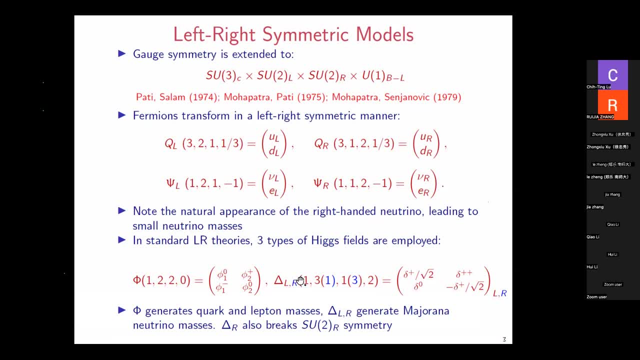 to what is called type two seesaw mechanism. The right-handed triplet generates the right-handed neutrino Majorana mass, which is much higher compared to the usual neutrino. So this theory contains the type one seesaw embedded in it, as well as a combination of our type two seesaw. 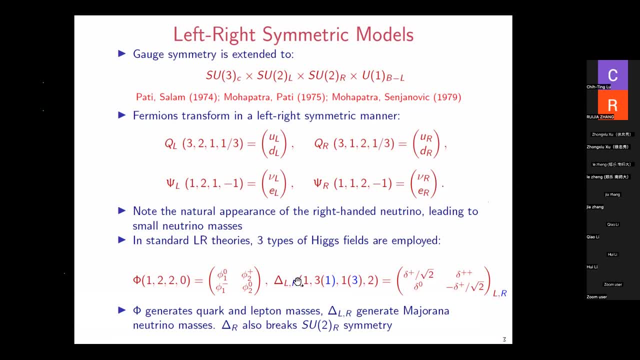 because parity symmetry requires the right-handed triplet should be accompanied by a left-handed triplet, And I will show that the parity transformation will take delta left to delta right. Okay, It will take phi to phi dagger, as I already pointed out. Okay. 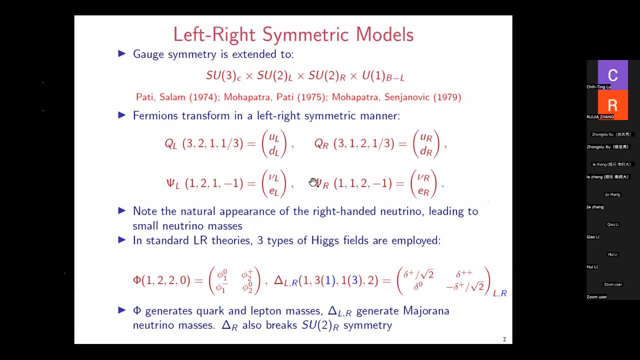 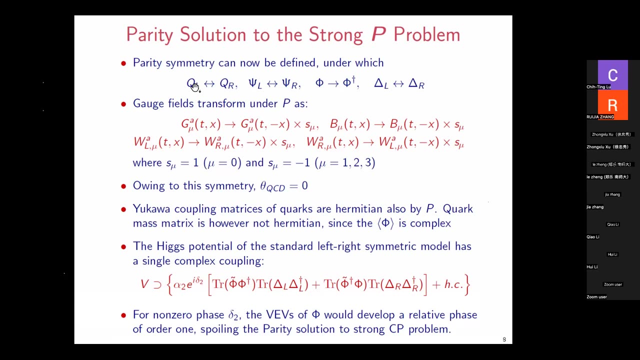 That's what makes the Yukawa coupling of this quads, as well as the leptons, to be Hermitian. Okay, Very good. So here is the in more detail: the parity transformation. under parity symmetry, left-handed quads goes to right-handed quads. 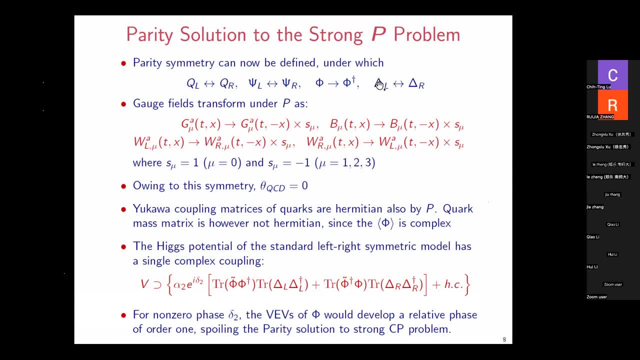 left-handed leptons goes to right-handed leptons, phi goes to phi dagger delta, the left-handed triplet goes to right-handed triplet And the gauge fields are given in more detail here. More interestingly, the left-handed W is transformed into right-handed W under parity. 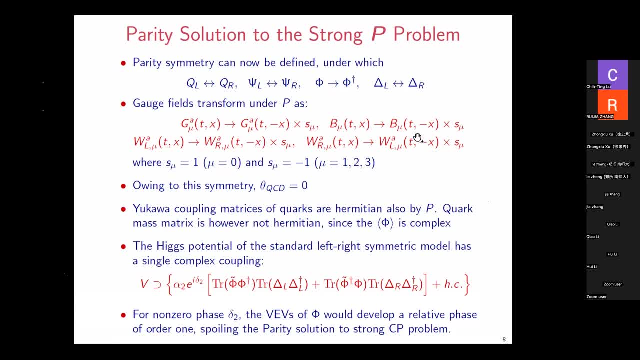 and right-handed W is transformed into left-handed W, And the sign factors are: well, this is S, mu is plus one, then the spacetime index is zero. It is minus one if it is spatial length accordingly. So it is true that the right-handed W will acquire a mass much higher. 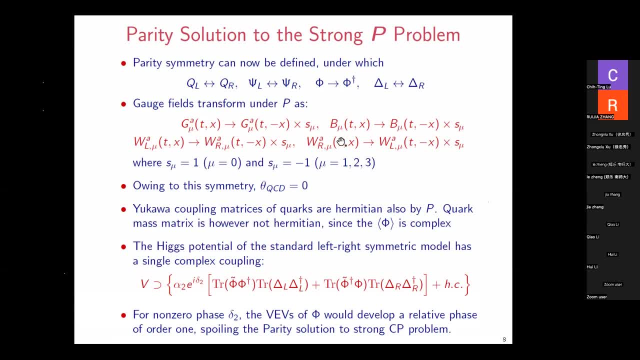 much heavier compared to the left-handed W, but this symmetry still is there And because of this symmetry, theta QCD can be set to zero. It is zero. I mean, if you have this symmetry, theta QCD has to be there. 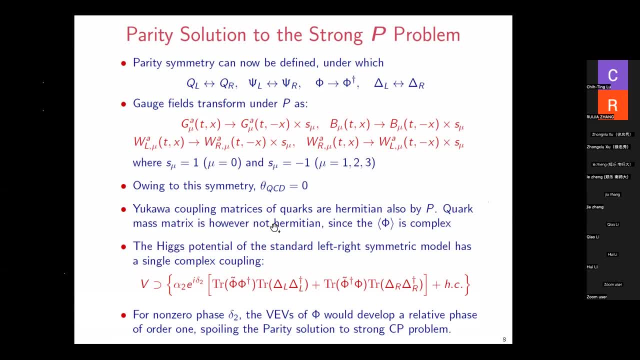 And, in addition, because of the same parity symmetry, we have a Hermitian Yukawa matrix. However, the vacuum expectation value of this phi field, which generates a the quark masses, it, cannot be made real. It turns out that many people have studied this. 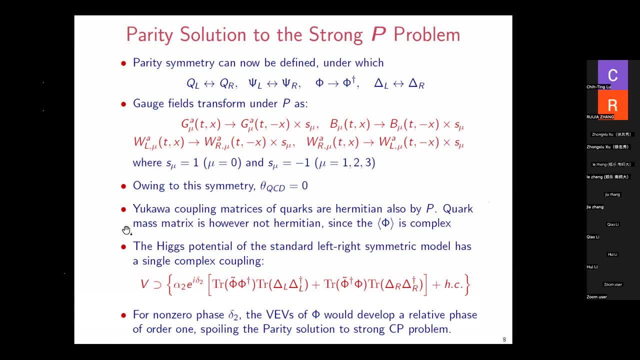 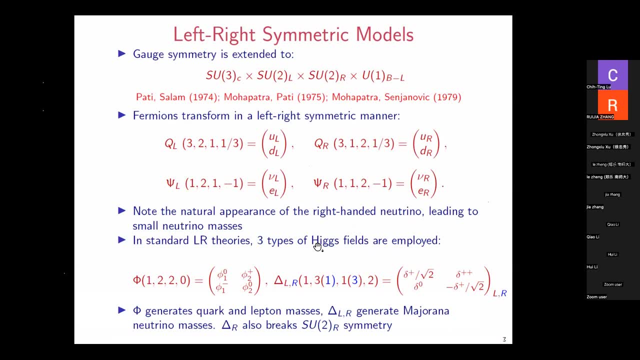 maybe some in the audience have studied it. It turns out that the Higgs potential with these fields is rather rich. There are like 20 terms. Every term is real because of parity, except one term, And that one term is listed here. 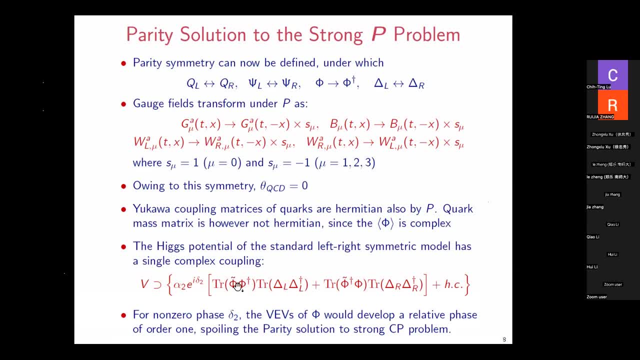 It's a kind of a mixed scalar field: phi tilde, phi dagger, delta, L, delta dagger- This is the parity invariant term And the coefficient is in general complex. So because of this, once they minimize the potential, the vacuum expectation value of the phi will be complex. 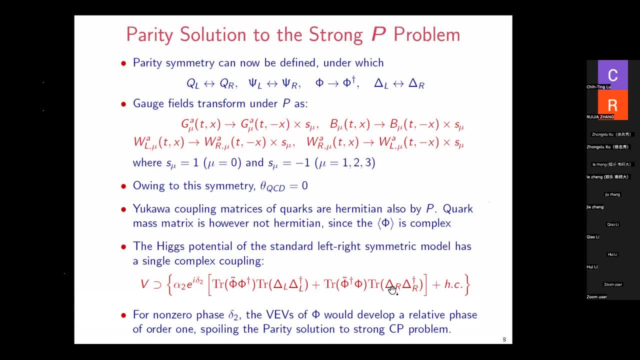 So this spoils the simple parity solution. In this version of left-right symmetry, the parity solution is not quite enough to solve the strong CP value. Okay, well, there's a good try, but we almost got there, but it was not quite sufficient. 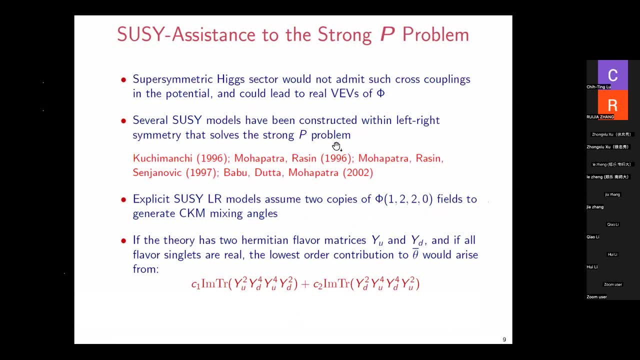 Okay, so what do we do? This is also there has been some effort to try to recover the solution in the standard left-right symmetric model. One idea is that if you have left-right symmetry and combine it with supersymmetry in the this term here, 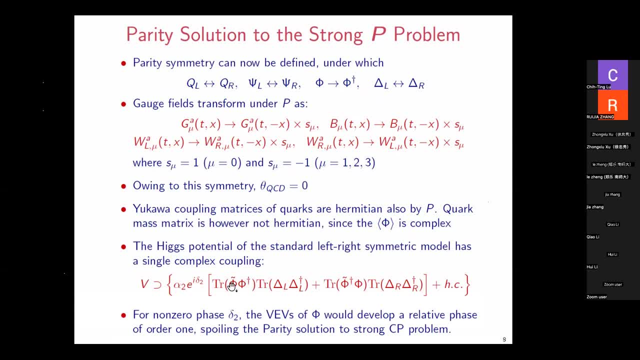 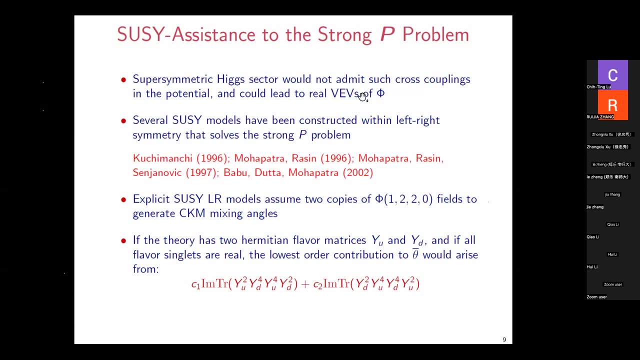 with the different fields involved, with some fields and some conjugate fields. this such a term is not easily generated in supersymmetry, So supersymmetry would have this term automatically resolved, So that feature has been used. What happens in supersymmetry is that you need two of these. 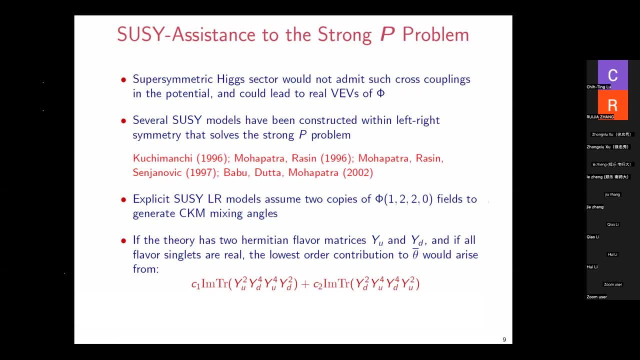 these phi fields in order to because the only well, you need to have two Yukawa couplings to generate the CK mixing elements. In non-supersymmetry, you can choose phi and a summation conjugate. that is enough. 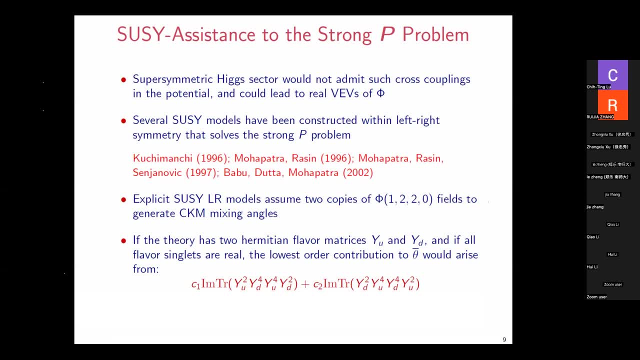 but in supersymmetry that is not possible because the superpotential has to be holomorphic. So people have studied multiple two Higgs fields and it turns out that the superpotential, all the parameters are real in many instances. I list here many of the studies. 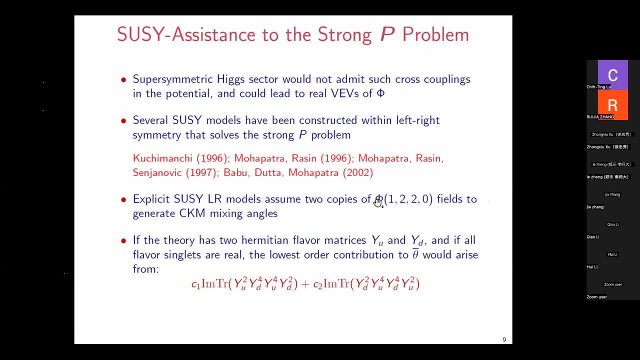 and I will kind of very quickly summarize the results here. And so this is something some, I think, very, very general, I think Given two Hermitian-Yukawa matrices, I mentioned that there are two phi's and so there are two Yukawa coupling matrices. 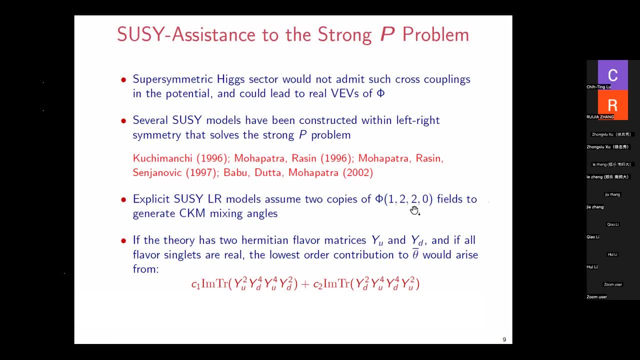 I can call them YU and YT. Now, given two Yukawa coupling matrices, we can try to make a flavor invariant, which is a singlet under the flavor symmetry. These are three by three matrices, right You? so you have to take trace of these products. 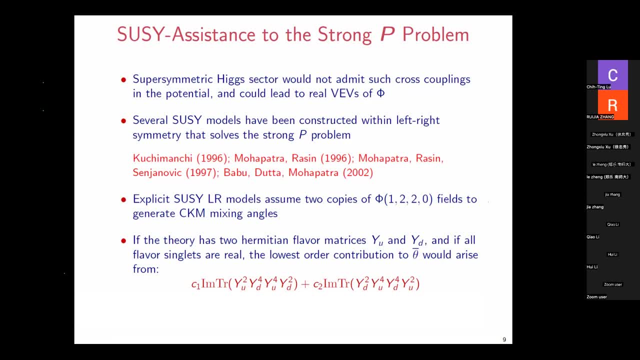 of this matrix in order to make a flavor singlet. You can one can see, after a little bit of playing around, you will see that the combination, that is complex, will have the 12 such coupling: YU squared, YD for YU for YD squared. 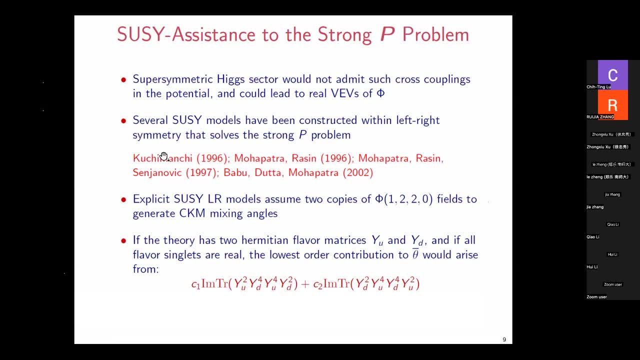 This is the lowest order term that is allowed to be complex. So that's actually interesting, because this means that in these supersymmetric models, only source of complex parameters are these Hermitian matrices YU and YD. It is very likely that the theta bar parameter 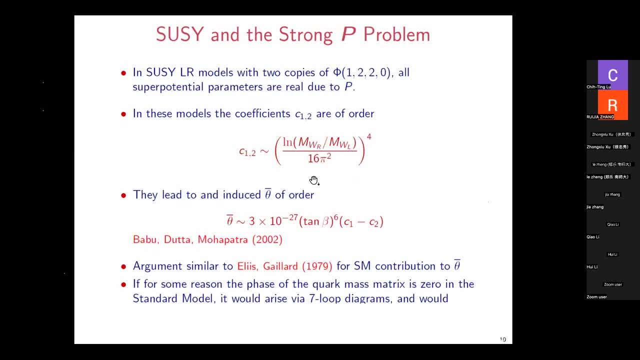 will be very, very tiny And indeed this has been checked in this, I think, in the model that we studied. This is again supersymmetric model. This coefficient C12, it arises at some four-loop level and the theta bar estimate is something of order. 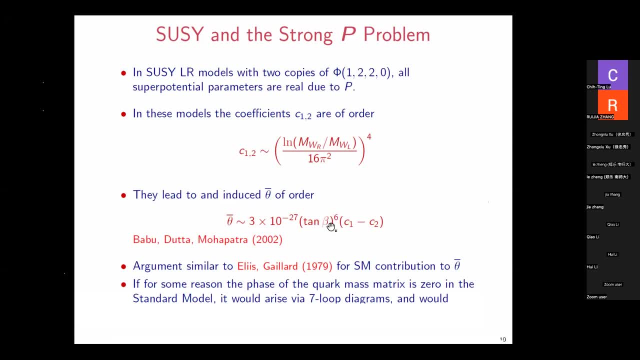 10 to the minus 27.. In supersymmetry there is tangent beta. it could be big like 10,, but still it is well below the experimentally required value. 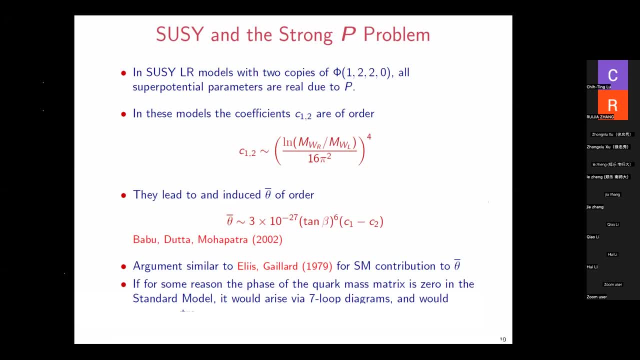 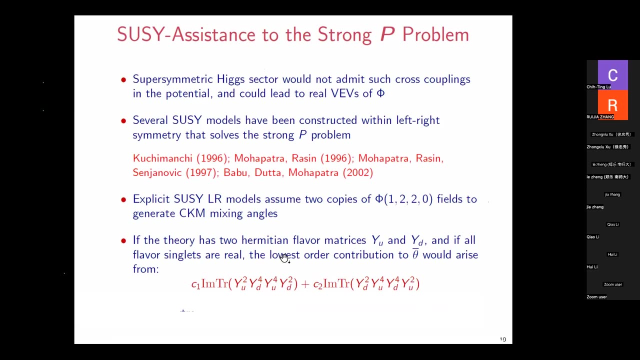 This is. this argument is very similar to an argument Ellis is wrong- Sorry, Ellison Gaillard- who studied the induced value of theta bar in the standard model. They found that of course, in the standard model Yukawa couplings are not permissive. 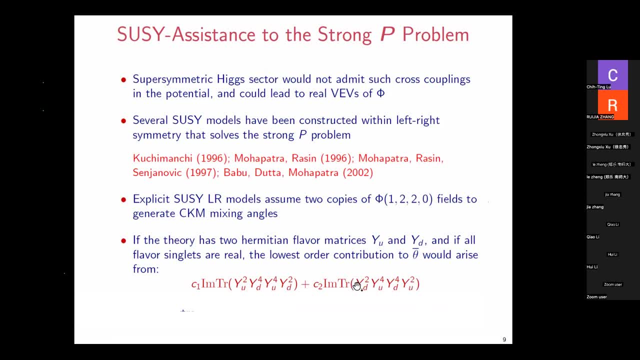 but they found that the lowest order where theta bar is induced is something like this: That's the 12 powers of your power coupling, But instead of YU or YD, you do YU, dagger YU, and YD, dagger YD. 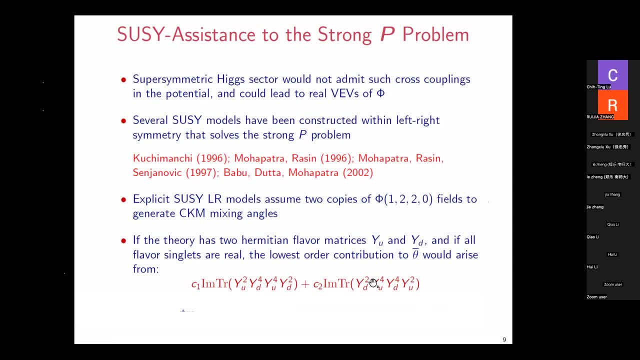 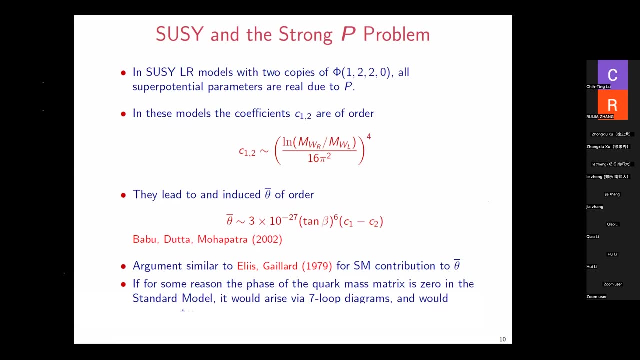 Then you replace this here. That is the lowest order where one would generate CP theta bar in the standard model. Hello, Yeah, Hello. I have one question. So because you introduced the supersymmetry, does the Sussi breaking will destroy this solution. 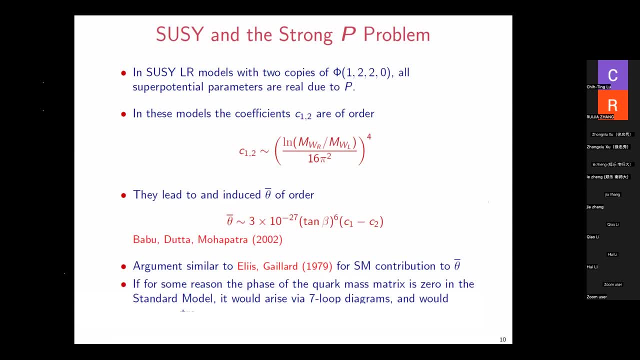 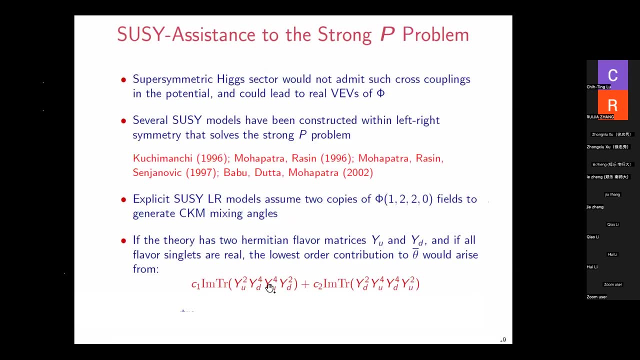 If we have a general Sussi breaking, we have the complex phase in the green. Yeah, you're right. So you're saying that that's a very good point. So in the supersymmetric models with these two Yukawa couplings of the phi field, the statement. 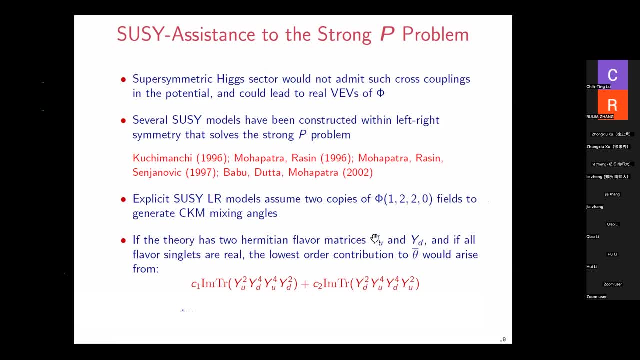 is that if there are only two, Two Hermitian-Yukawa matrices, and all others are real scalars, real scalar singlet, then this is the lowest order theta bar you can generate. But you're right that in supersymmetry 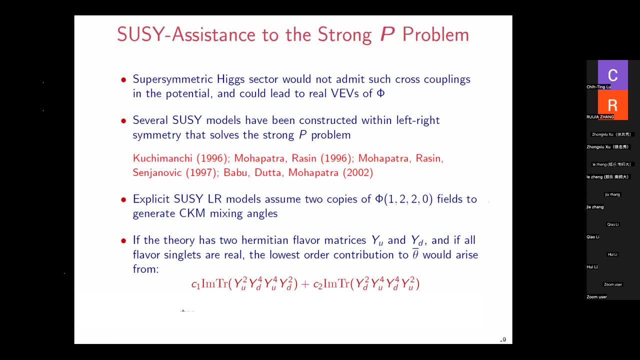 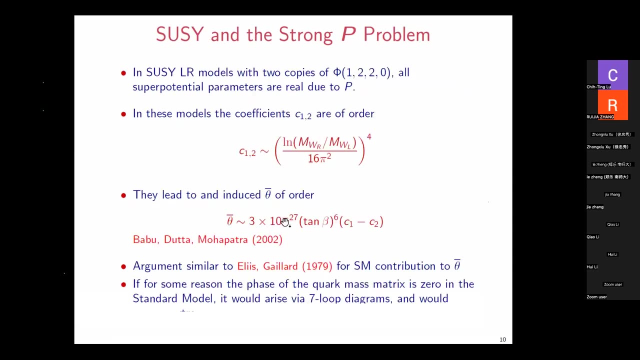 if you have a general supersymmetry breaking then there could be a flavor structure associated, And if those flavor structure deviate from the flavor structure in the Yukawa couplings, then there could be additional contributions. So this estimate is no longer true. 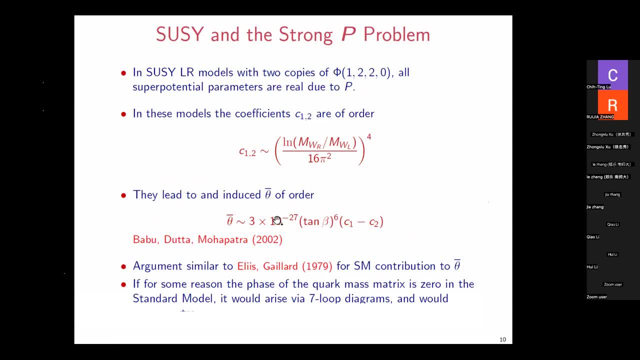 In fact, in this paper we had done that estimate. It's actually become much bigger. It could be of order 10 to the minus 10.. But it's still suppressed. It is suppressed. This estimate, I would say, is the supersymmetry. 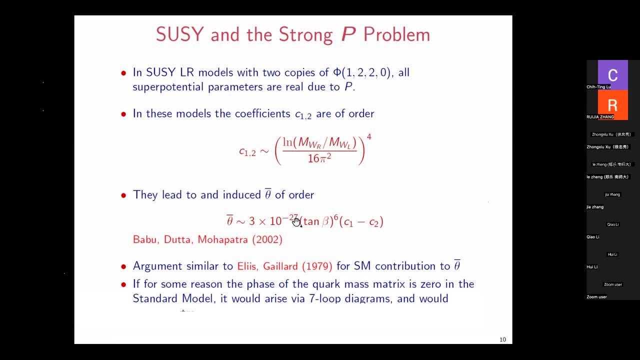 with some universal supergravity-like type boundary condition. This will be true in supergravity-based supersymmetry breaking, But for general supersymmetry breaking this could be much bigger. I agree. OK, thank you. So this is also true for the standard model. 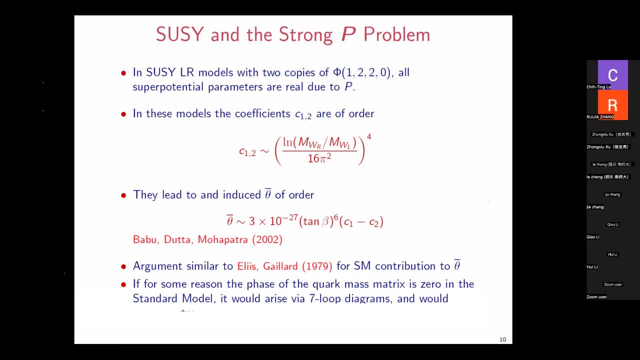 If, for some reason, if the phase of the quark mass matrix was very small- 0,, for whatever reason which we don't know- then the induced value would be quite small. It has to arise at some 7-loop diagram, But of course it doesn't solve the strong safety problem. 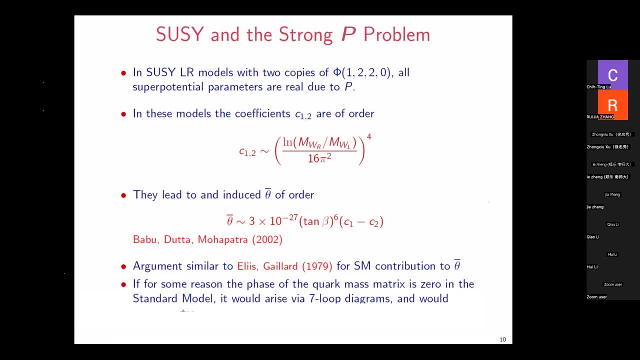 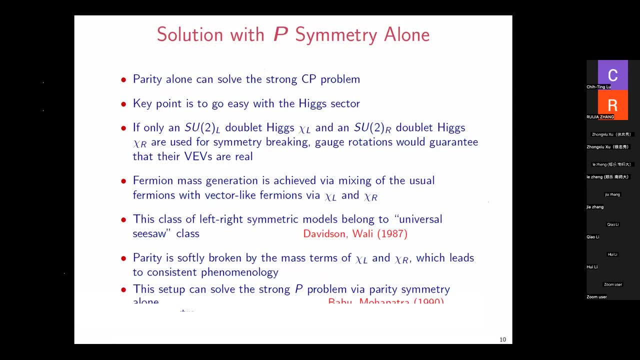 Standard model. the statement is that if, for some reason, theta bar was 0 to begin with, it will stay that way. OK, so in the remainder of most of the talk I will show that parity symmetry alone, without relying on discrete symmetries or supersymmetry. 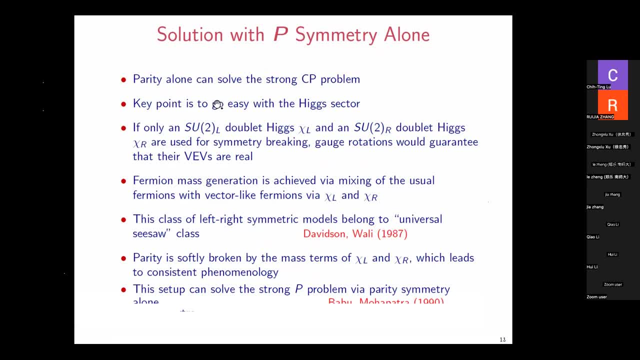 it can solve the strong safety problem. The key point of this idea is that we go easy on the Higgs sector. Remember, in the standard left-right symmetry there were several Higgs fields that made the vacuum expectation value complex. OK, But if you can construct a class of left-right symmetric models, 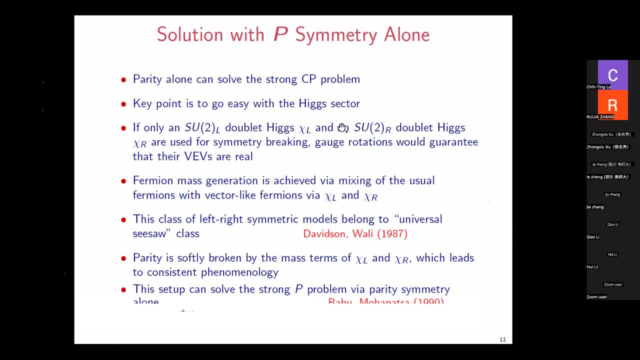 where you have only a doublet Higgs field, one for SU to left, one for SU to right- then by gauge rotation the vacuum expectation value can be made real. OK, In that case, without any loss of generality, the vacuum expectation value are all real. 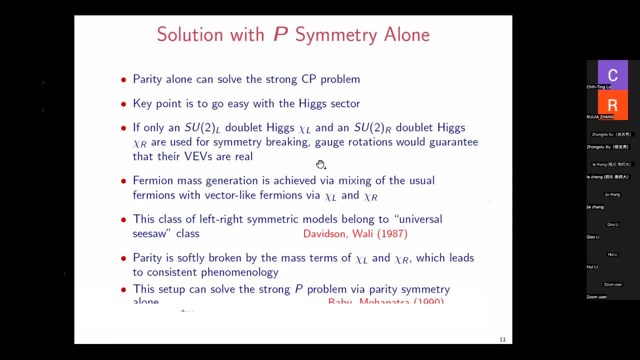 However, this causes a little bit of a difficulty because this left-handed doublet and right-handed doublet cannot generate the quark mass. That is achieved by introducing a vector-like fermion. So standard model fermions can mix with this vector-like fermions through this left-handed 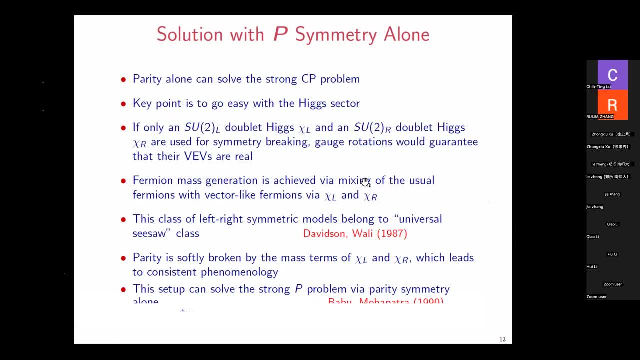 doublet and right-handed doublet. And so what happens in this class of models is that all the fermions like quarks charged leptons. they will acquire mass through a seesaw-like mechanism. This has been studied by Davidson and Wally in 1987.. 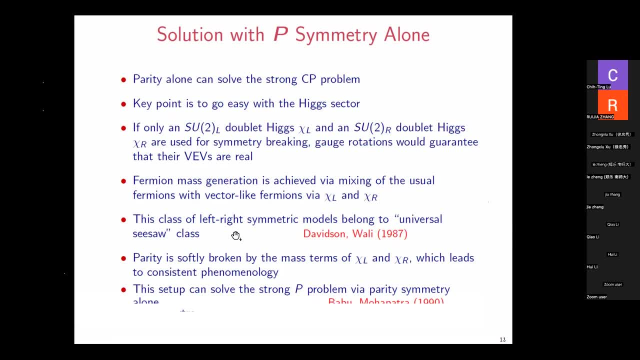 They call it universal seesaw, That is, every particle is getting its mass through a seesaw mechanism. Now we have to still have: the vacuum expectation value of the left-handed doublet should be much smaller compared to the vacuum expectation value of the right-handed doublet, so that the WR is much heavier. 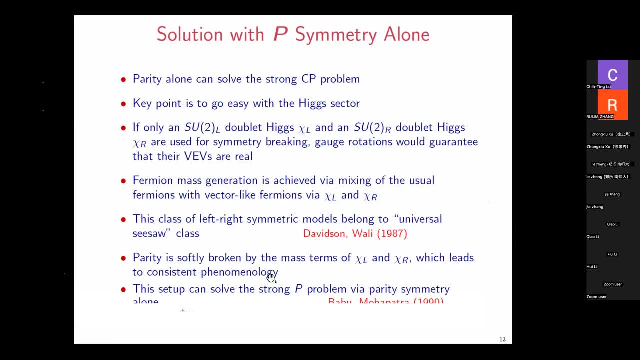 than WL. That is needed for consistent phenomenology And this can be achieved by in the Higgs potential we can softly break this parity symmetry in the mass term for chi-L and chi-R. Then that doesn't introduce any divergence anywhere in the theta bar. 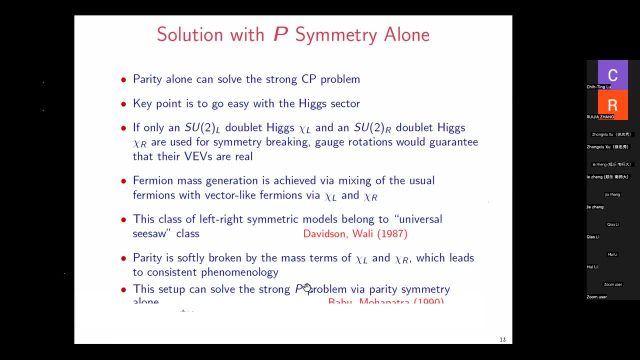 So this provides a good setup where strong parity problem can be solved. This was initially suggested by Mahapatra and me in this context some years ago, But recently there have been a lot of activity on this idea And I want to kind of summarize that. 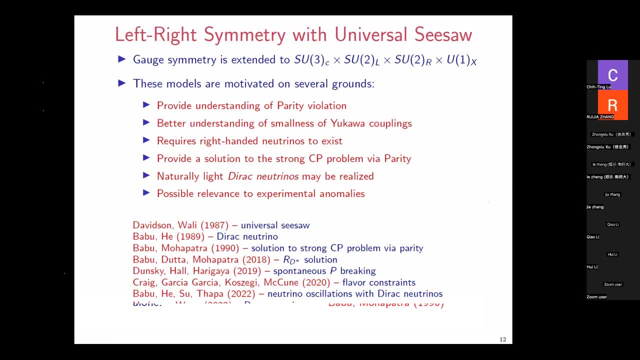 So this is not the traditional left-right symmetric model. It is a left-right symmetric model with this universal seesaw. The gauge symmetry is, as in this left-right model, You have SU left cross, SU right cross, U1.. And these are motivated on several grounds. 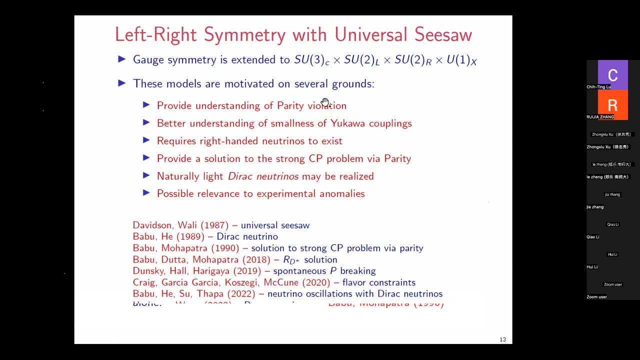 First of all, parity violation is explained as a spontaneous origin Because it's going to give us a seesaw mechanism for quarks that you call a quark, And these quark couplings are not as widespread In the standard model. the quark couplings. 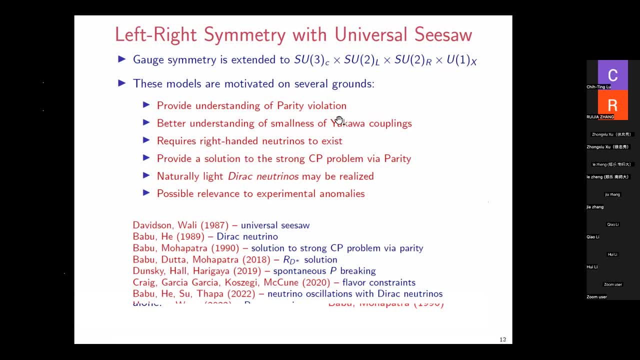 range from 1 to 10 to the minus 6.. But if you know the seesaw formula, you know the quark couplings in a seesaw mechanism. it can go from 1 to 10 to the minus 3.. So there is a little bit of the spread, is not that so much? 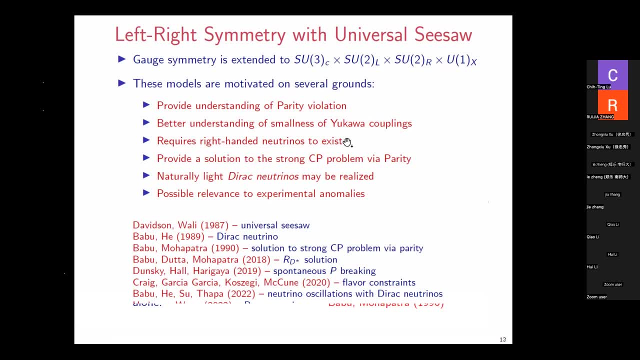 And, as in the standard left-right, it requires the existence of right-handed neutrino and therefore neutrino mass And, as I will show, it has a solution to parity, which is a problem, And it turns out that it can provide naturally. 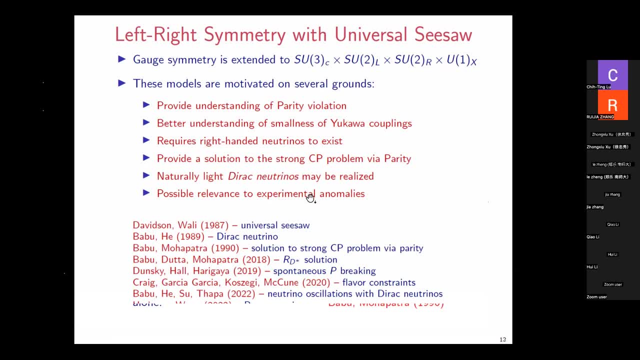 light derogating treatment. I will say a little bit more about it And there may be some possible relevance to experimental anomalies. I will talk a little bit more. So I already gave some references. The universal seesaw is 87. He Xiaogang and I actually pointed out soon. 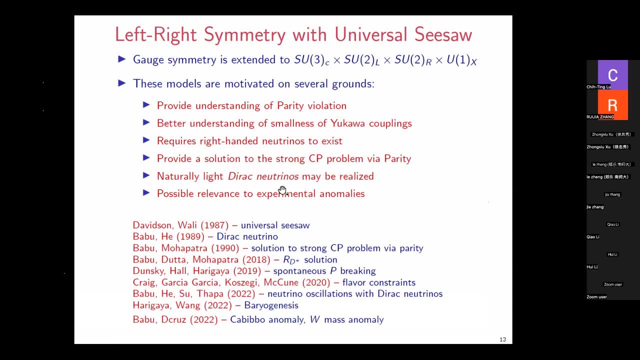 after this idea was proposed that neutrinos may be derog particles And this was kind of forgotten until recently. So Xiaogang and my previous student Mingxian Su and Anil Tapai we looked at it in this neutrino oscillations. 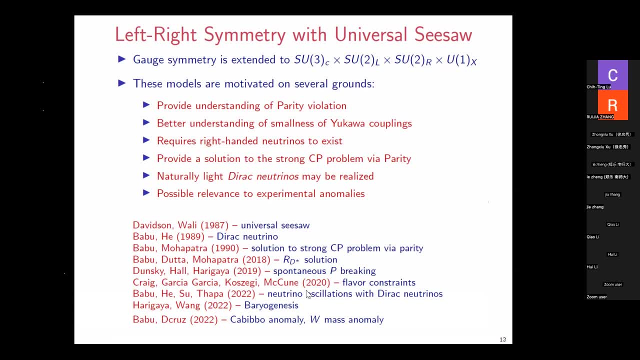 And we showed that the derog neutrinos that arise from here actually fit the neutrino oscillation data. well, I'll summarize that result, And I already talked about the strong CP solution. Some of the anomalies were suggested to be explained in this setup. 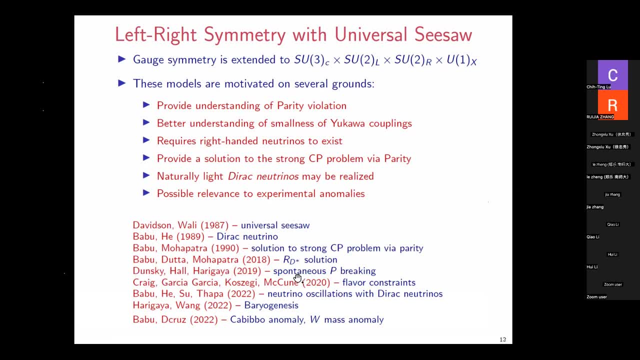 This group, the Berkeley group, had studied this with the purely spontaneous parity breaking, without even having the soft breaking of parity This requires. I will not talk much about it, but it's exactly the same setup, except that the right-handed breaking scale has to be rather heavy. 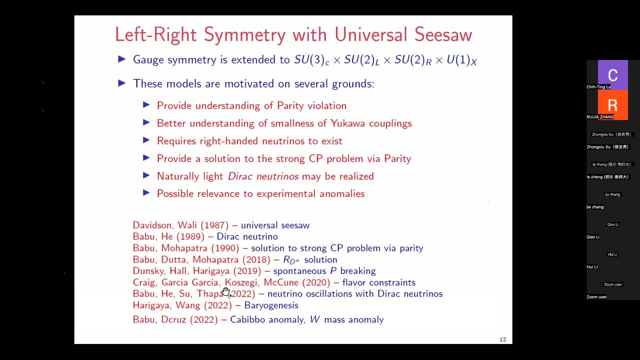 Flavor constraints have been studied by the Santa Barbara group And more recently, there has been a study by Hari Gaya and Wang on bariogenesis in these models. And I will finally talk about the anomalies with my student, DeCruz and I are coming out with a paper. 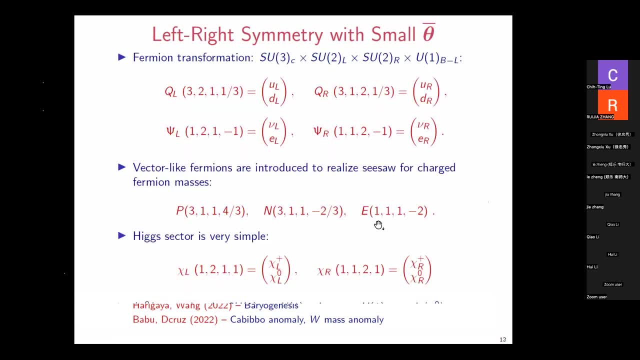 soon. So this is a general setup. So the setup is something like this: The gauge group is the standard left-right, All the fermions are, as I already discussed, But then we introduce this model, introduces this vector-like fermion. 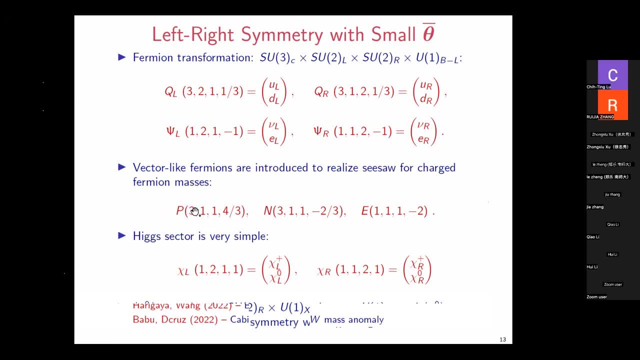 This is P corresponds to up-type fermion. So the up-quart mixes with this P, down-quart mixes with N and charge-laptron mixes with E And this mixing occurs through this. the Higgs vector is very simple. 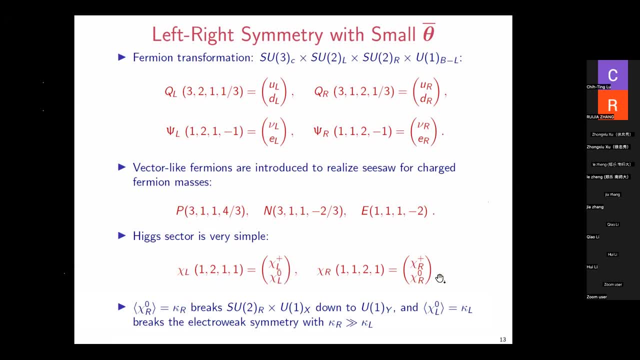 There is a left-handed doublet and right-handed doublet And their vacuum expectation values are real. So this mixing occurs, say QL bar. let's say take NR QL bar, NR chi-L. That is one of the allowed interactions. 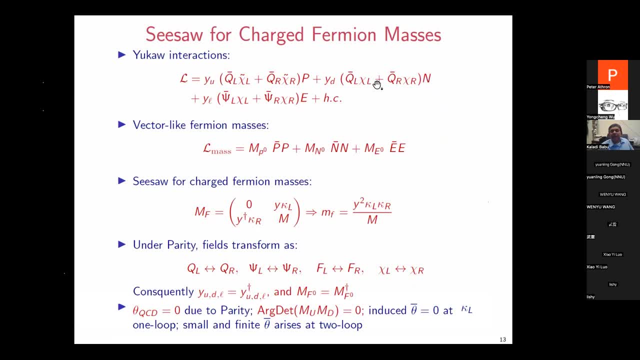 And I have written down here: QL bar- chi-L N, QR bar- chi-R N. And these coefficients are exactly the same because of parity symmetry, Because under parity, QL goes to QR, chi-L goes to chi-R. 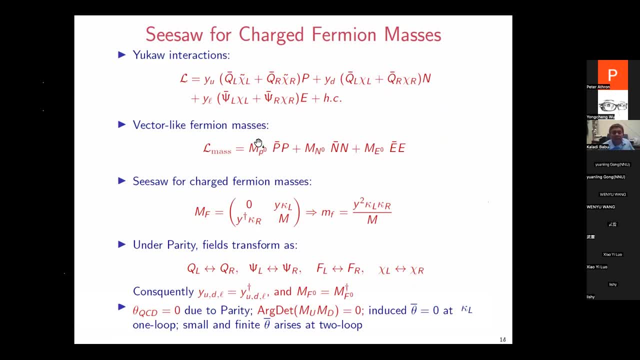 Therefore the coefficients have to be exactly the same And then these vector-like fermions can have bare masses that are given here, And these bare masses have to be Hermitian matrices because under parity symmetry the left-handed fermion goes to right-handed fermion. 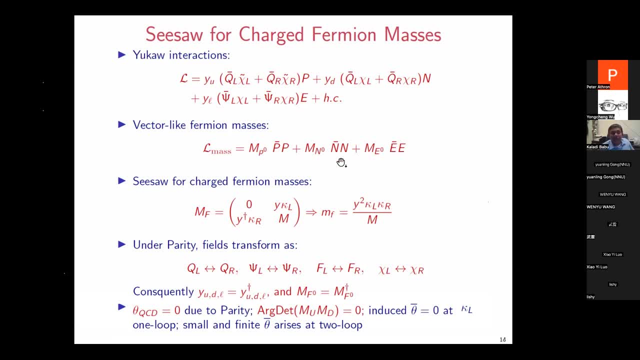 That makes it bare mass matrix. It has to be Hermitian. So the full mass matrix for any say up-quad sector is given by this kind of a seesaw matrix And by the diagonalization of that the ordinary fermions will get some mass. 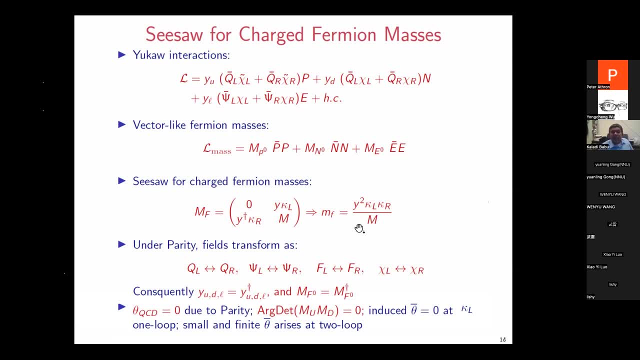 given by the seesaw formula And, more importantly, because it is y here and y dagger there, and the vacuum expectation values are real. if you look at the determinant of this mass matrix, it is real. That means that at tree level, theta bar has to be 0. 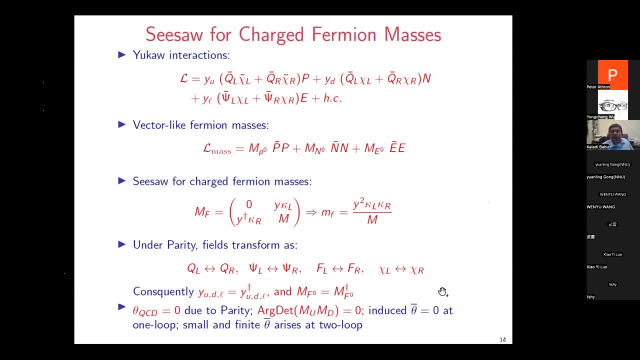 Argument: determinant of mu m t is 0. Therefore theta bar is 0 at tree level. Now theta bar will be induced at loop level. So we have to, because the experimental constraint is quite severe. we have to make sure that the induced theta bar 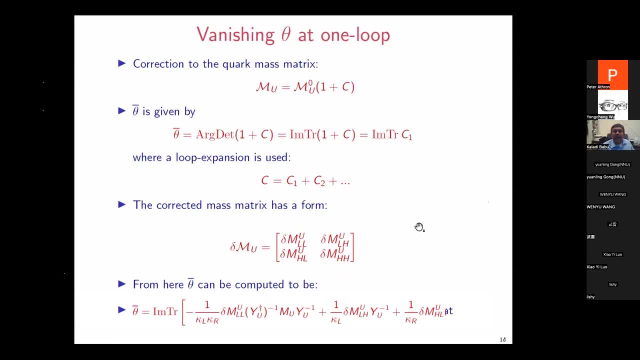 is sufficiently small And that has been studied. vanishing of theta bar. It turns out that in this setup, theta bar is actually going to be 0.. The one-loop correction to Theta bar is exactly the same And this is the calculation that is shown. 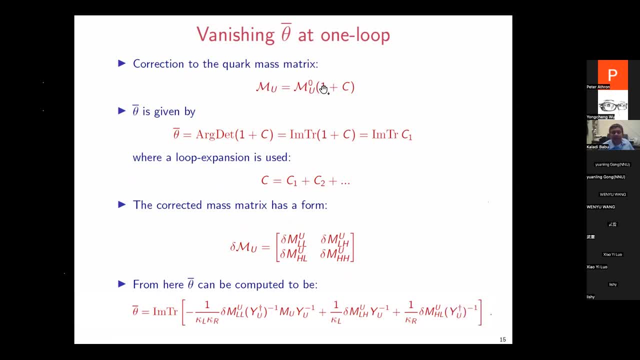 I can write the up-cork mass matrix as the tree-level matrix times 1 plus some correction matrix And this correction matrix, every entry, every block is corrected. That is shown here And one can go ahead and compute the induced value of Theta bar. 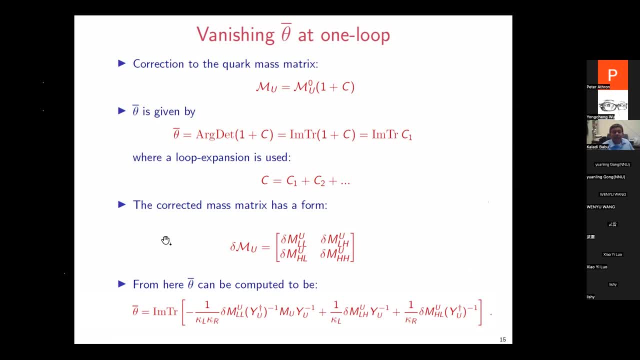 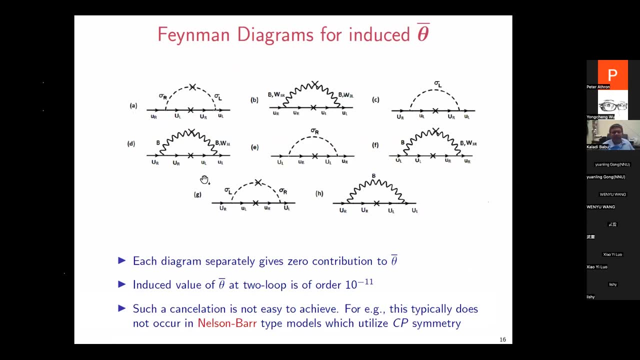 The formula is given at the bottom of this slide And these are the one-loop diagrams. There are gauge boson exchanges involving the left-handed W- right-handed W. There are Higgs boson exchanges. This is the B-minus-L gauge boson. 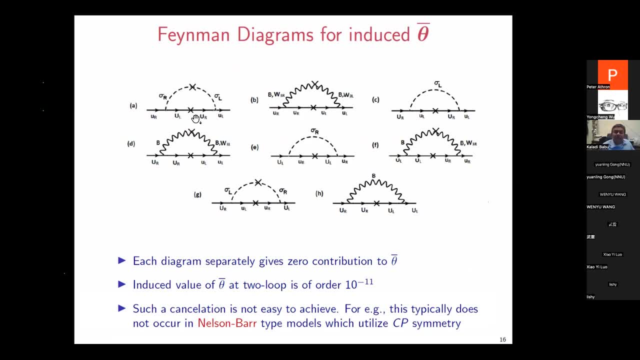 Actually, it turns out that every diagram separately gives zero contribution to Theta bar at one-loop level. This is very interesting because Theta bar is then going to be really supported by some two-loop factor. And this is the one-loop diagram. And this is the one-loop diagram. 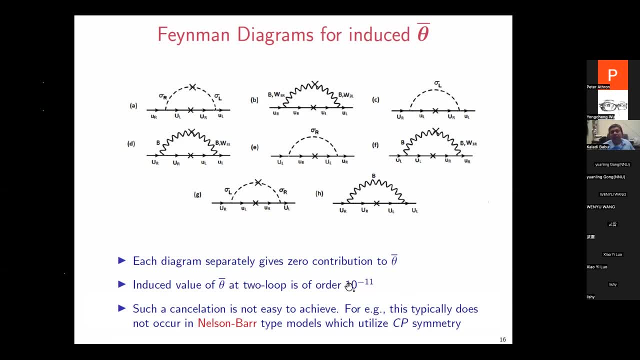 And we estimated the two-loop induced Theta bar, It comes out of order 10 to the minus 11.. This is, I think, a very nice solution to the strong CP problem. I should point out that this cancellation of Theta bar at one-loop, or the vanishing of Theta bar at one-loop, 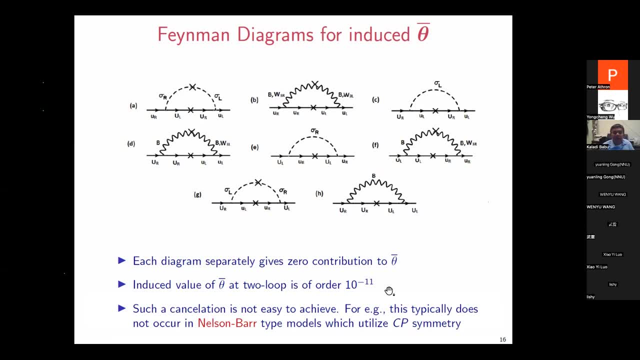 it is not shared by another class of models called the Nelson-Barr model, which is a similar idea, except that instead of parity, they use CP symmetry, If you look at the two-loop induced Theta bar. it is not shared by another class of models called the Nelson-Barr model. which is a similar idea, except that instead of parity, they use CP symmetry. If you look at the two-loop induced Theta bar, it is not shared by another class of models called the Nelson-Barr model, which is a similar idea, except that instead of parity, they use CP symmetry. 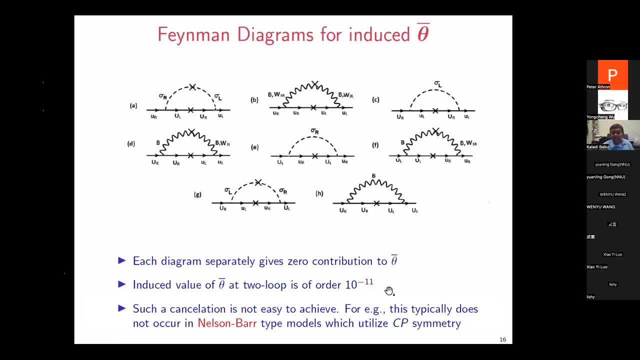 If you have spontaneously broken CP symmetry one can suppress Theta bar. but typically one would get Theta bar induced at one-loop level And unless you tune parameters appropriately, the Theta bar less than 10 to the minus 10 is relatively hard to achieve there. 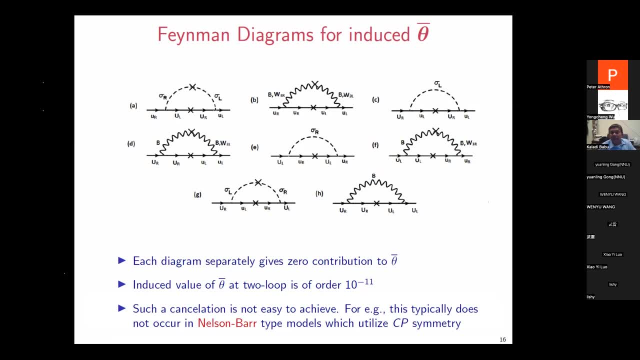 But in the model I presented it is pretty easy to get it because all the one-loop diagrams are. it's the power of parity, Parity breaking. is this diagram? remember that it originated from parity invariant theory? Okay, this is a side comment. 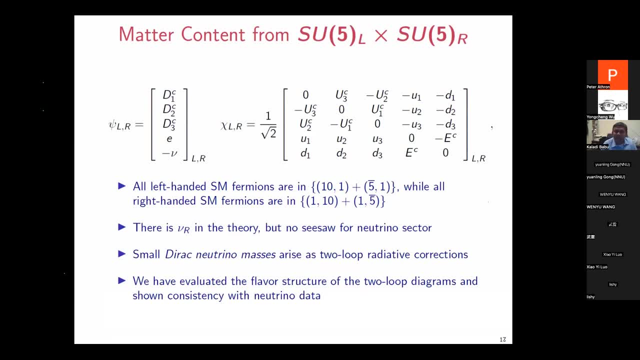 The particle content that is used in this universal seesaw mechanism. that actually can be embedded into a unified theory based on SU5 left cross SU5 right. The idea here is that all the left-handed fermions are multiplex of SU5 left. 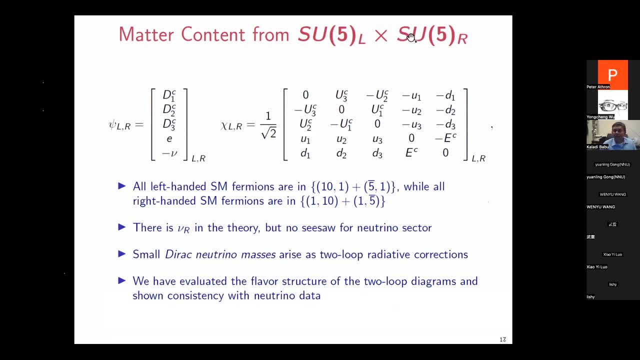 and all the right-handed fermions are multiplex of an SU5 right. In this setup, the number of particles is exactly fitting to SU5 left cross SU5 right. You see that, yeah, there is a new right. You see, the SU5 right contains a multiplex which has a right-handed neutrino. 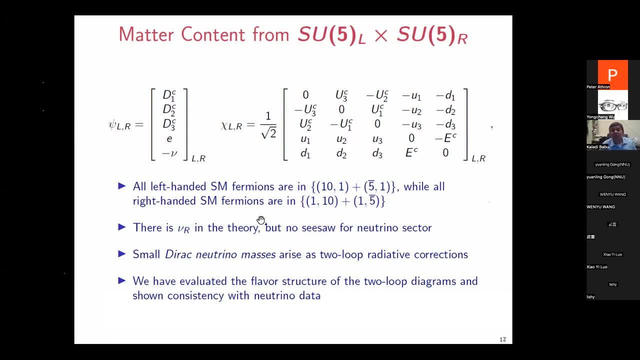 Even so, there need not be a seesaw mechanism. The neutrino could remain at the right part of this And the masses will arise only at some two-loop level, as I will show. So this is an interesting scenario, where the neutrino masses are of the Dirac type. 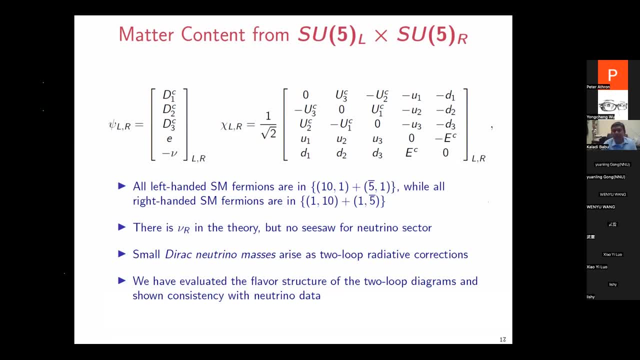 but also still very suppressed, And this just comes out from the gauge structure. It was not something required, but the theory was motivated by introducing parity symmetry and also to solve the Schanzky-P problem. But as an outcome, it provides us for free, very tiny Dirac neutrinos. 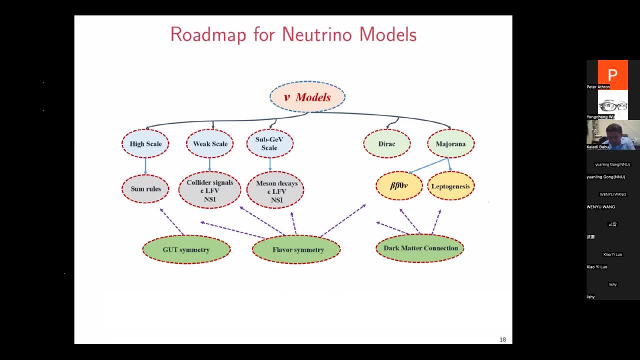 So I may have to hurry up a little bit, but this is a very general overview of neutrinos are very important. There are major experimental efforts going on to study the properties of neutrinos as a roadmap. We know a lot about neutrinos, about their masses, oscillations. 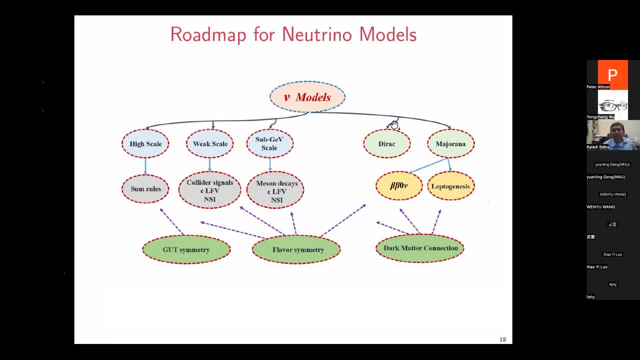 but we have many. There are many things that we don't know. For example, whether they are Dirac or Maserana is unknown. If it is Maserana, that would lead to neutrinos of double beta decay connected to leptogenesis. 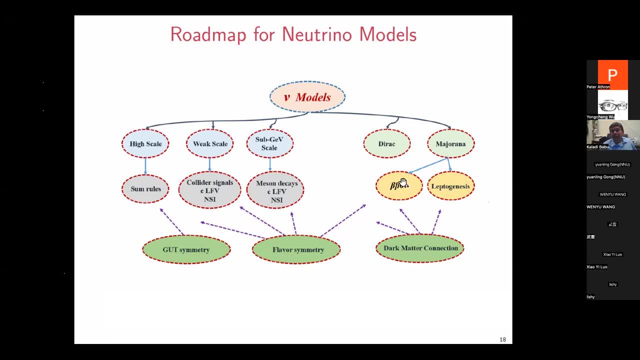 We don't know. Dirac neutrinos don't lead directly to neutrinos of double beta decay. That's one way to distinguish. We don't know the scale at which neutrino masses are generated. It could be a very high scale, could be a very weak scale, could be electron volt scale. 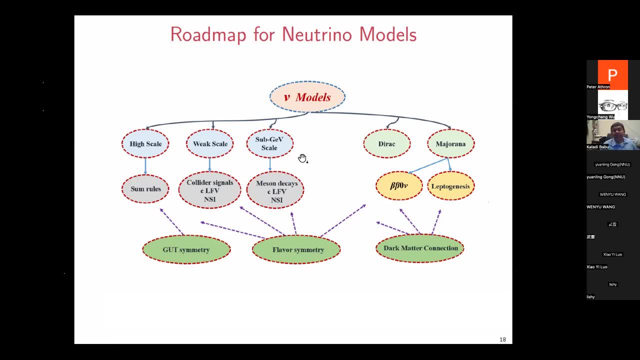 We have no idea These are. These experiments will currently going. ongoing experiment and also lighter experiments could provide us more deeper understanding of this. At the moment, we don't know the origin of neutrino mass or also the nature of the particle itself. 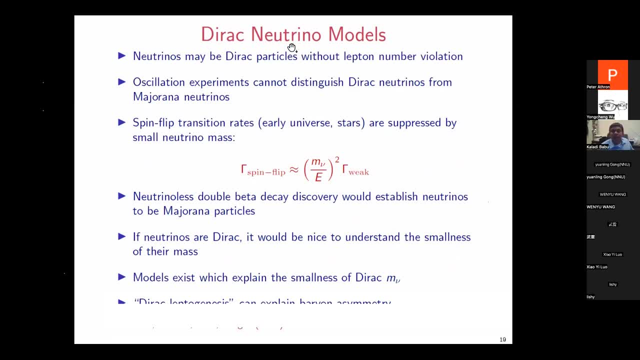 So this is somewhat unconventional. Dirac neutrino models are OK. from phenomenology, You might say. the neutrino oscillation cannot distinguish a Dirac neutrino from Maserana neutrino. You might think that Whatever spin-flip transitions in early universe cosmology et cetera, wouldn't that disfavor a Dirac neutrino because it has a sterile component? 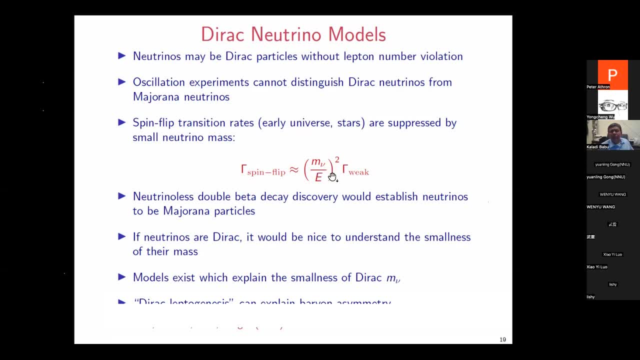 But that is not true, because the spin-flip transitions will go like the rate, will go like mass of the neutrino over the energy squared. So this is highly suppressed. If it is a Dirac particle, it would be nice to understand why the mass is small. 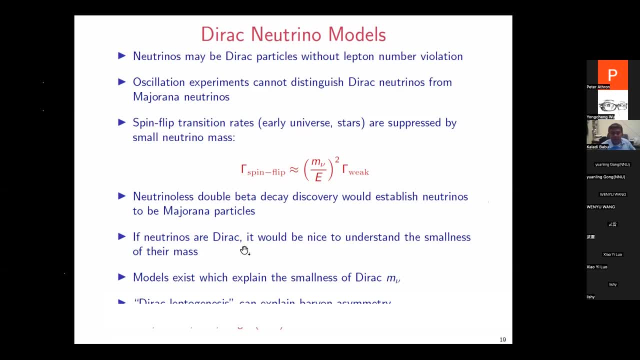 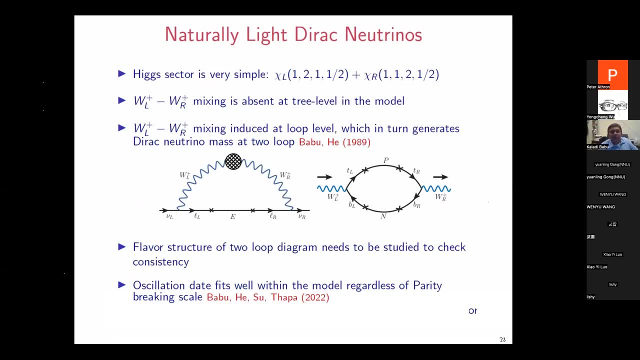 And there exists Dirac neutrino mass models And I will jump right into- Let me skip this, Yeah, right into- this model that we are discussing. So this left-right symmetric model has a simple Higgs sector, Left-handed doublet and right-handed doublet. 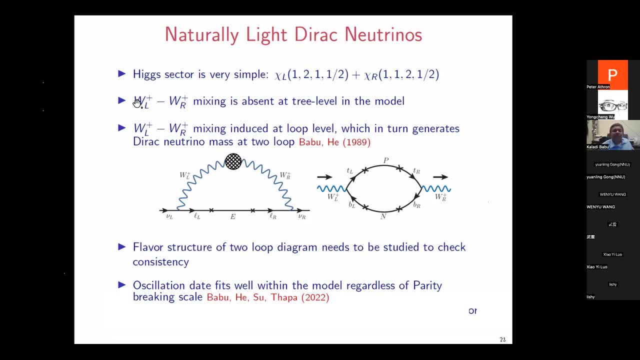 With such a simple Higgs sector, it turns out that the masses- there is no mixed mass term between WL and WL. There is no mixing between WL plus and WL at tree level. However, through Loop level, left-handed W will mix with right-handed W. 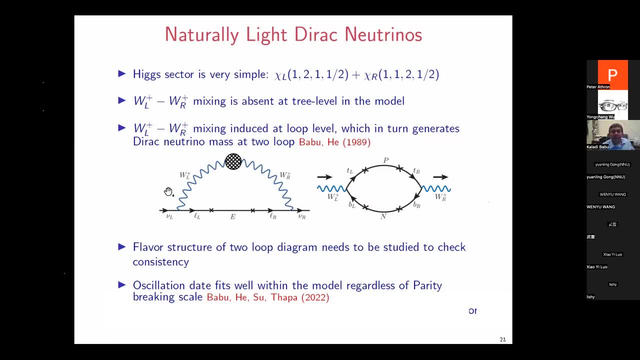 And the diagram is shown here. And if we insert it into this diagram on the left, one would generate a two-loop level, a Dirac neutrino. Because it is a two-loop diagram, magnitude is highly suppressed And, as I already said, there is no seesaw for the Dirac neutrino with the spectrum that is suggested by this theory. 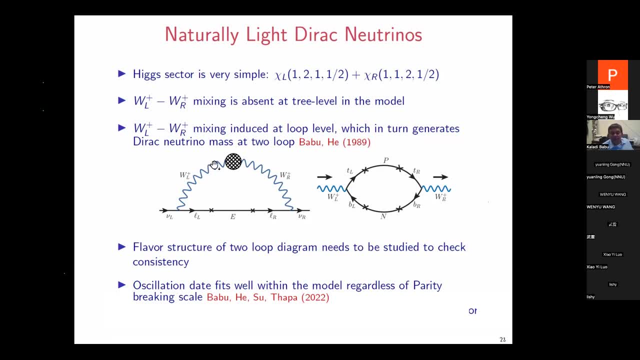 Now, recently We looked at the flavor structure of this and to see whether it is consistent with neutrino oscillation data, And this is the work with the Shaogang, Mingfian and Anil that we wrote recently, And so the challenge there was to evaluate this two-loop diagram. 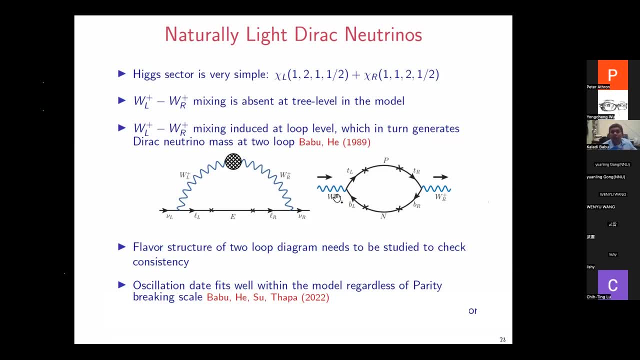 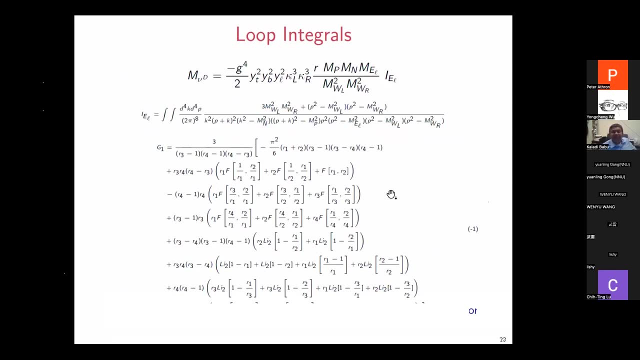 For evaluating the two-loop diagram. we had to put this W to be off-shell And that is actually. we were able to do it, and this is the details of the two-loop evaluation And the summary is that this is our best fit to the neutrino oscillation data in the two-loop Dirac-Math model. 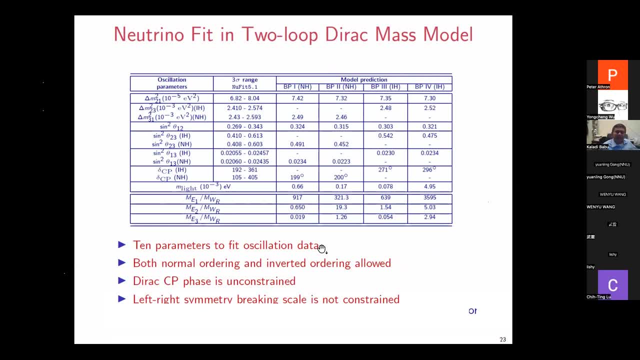 There are about 10 parameters to fit oscillation data and the charged lepton masses, And so there is enough freedom. It admits both normal ordering and inverted ordering of neutrino masses. The CP phase, the Dirac CP phase, is unconstrained. 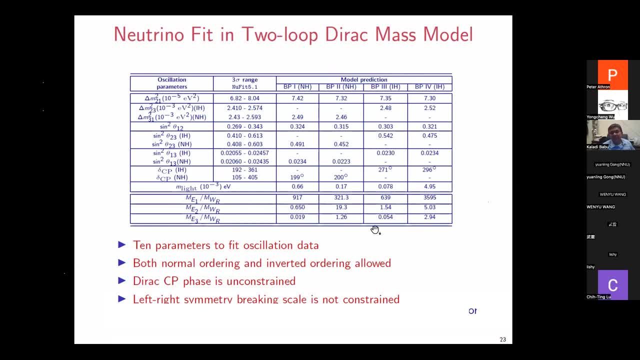 The scale of left-right symmetry also is not really constrained. It is really the Dirac-Math is a, it's a coefficient of a dimension four operator, So it does not decouple. if you made the mass of right-handed W very heavy. 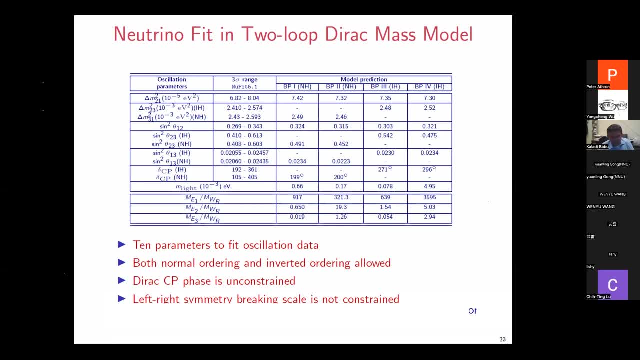 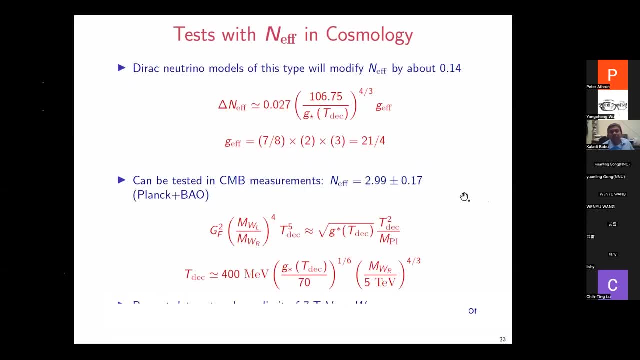 So unfortunately we cannot pinpoint what the mass of right-handed W should be from neutrino oscillation data. But otherwise it is all it's all good. Now, one way to test the idea that neutrino arising from this kind of theory is a Dirac particle is through the cosmological parameter and effective. 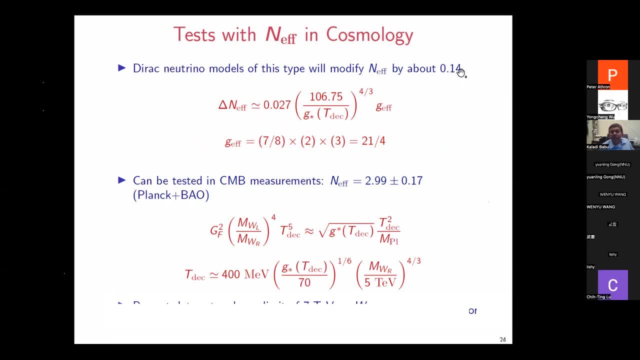 It turns out that Dirac neutrinos will shift and effective by this number, 0.14.. This 0.14 comes from- this is the expression. There is a g effective, the number of light degrees of freedom in thermal equilibrium. 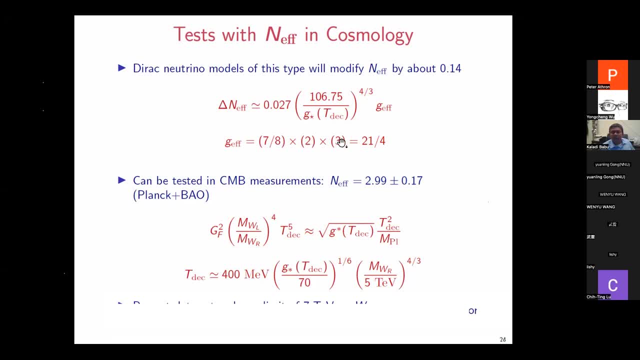 Seven-eighth is due to fermion. The two is for spin. There are three right-handed neutrinos. that comes out to this much: Currently, Planck satellite data puts a limit of an effective. it cannot be modulated, but it puts a limit of an effective. it cannot be modulated. but it puts a limit of an effective. it cannot be modulated. 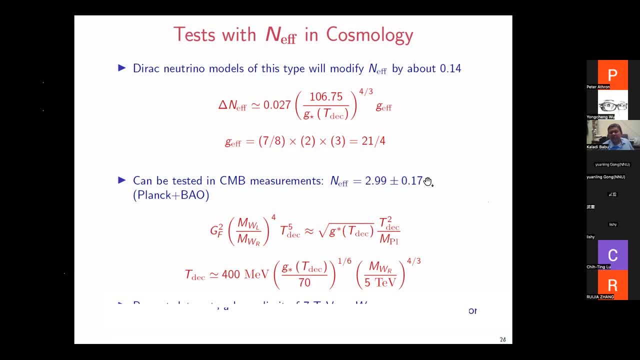 it cannot be modulated, but it puts a limit of an effective. it cannot be modulated, but it puts a limit of an effective. it cannot be more than at one sigma. It cannot be more than 3.2 or so. 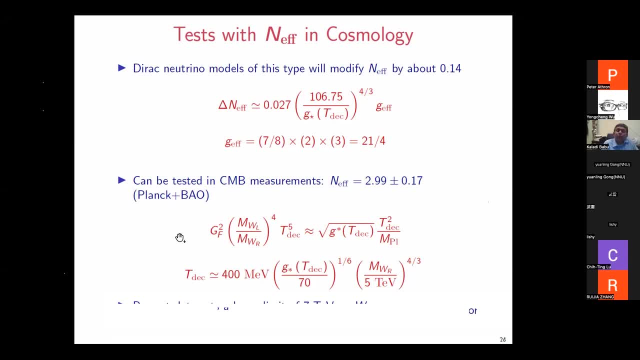 And these right-handed neutrinos were in thermal equilibrium through the right-handed gauge, both on interactions And they decouple. the right-handed neutrino will decouple from the thermal plasma around 400 MeV or so for low right-handed W mass And using this one can determine that delta and effective predicted by this theory. 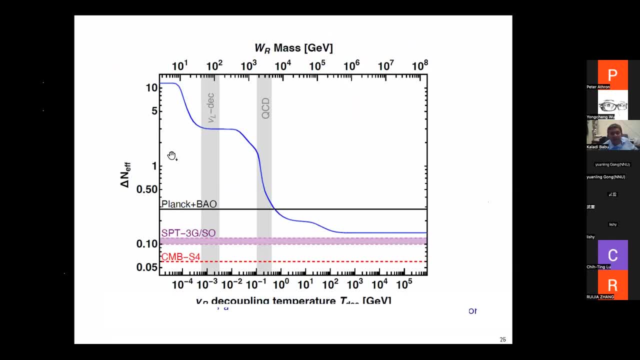 And that is shown here. So this is the decoupling new R decoupling temperature And on the top there is a WR mass. This is the new R decoupling temperature from the formula I just showed you And already we see that the Planck data puts a lower limit of about 7 TeV on the right-handed W. 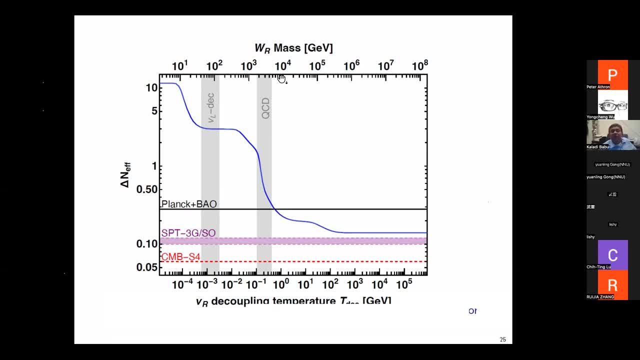 mass which is a little bit stronger than the LSC limit of 4 TeV on the WR mass But, more interestingly, in the second bone it is an effective gain and less effective gain. the near future. there are two experiments: the Southpaw telescope and the CMB stage four. 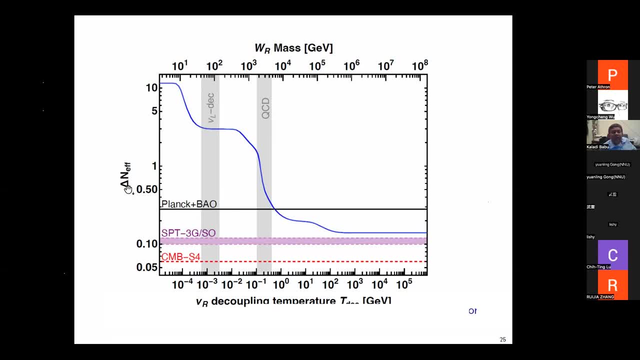 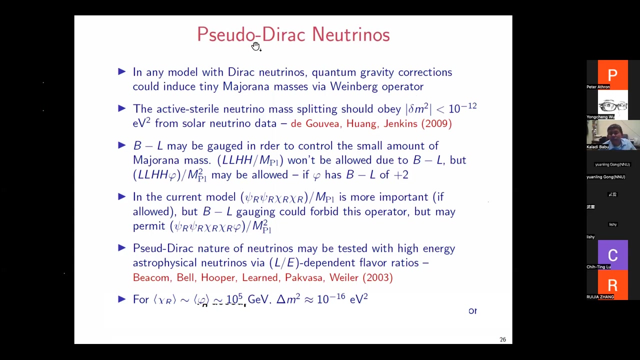 experiments are supposed to pinpoint an effective to a few percent level, And since the deviation is predicted to be 0.14, there is a good chance that this could either confirm the idea that neutrinos are Dirac particles or exclude this idea. Let me, maybe because of short of time, The idea that this neutrinos could also be pseudo. 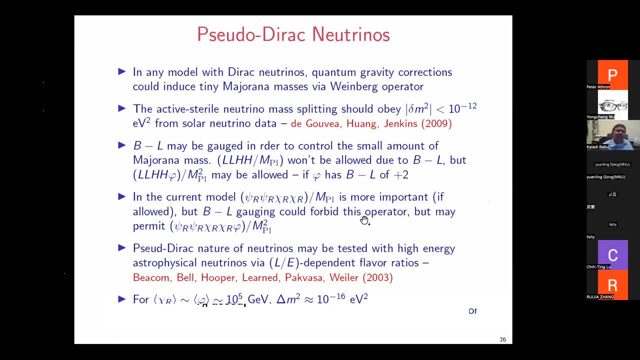 Dirac particles. I will. it is the pseudo Dirac particles are like Dirac particles, but fundamentally they are Majorana particles. The off-diagonal entries dominate over the diagonal entries in the seesaw matrix, So this has been studied by various groups and 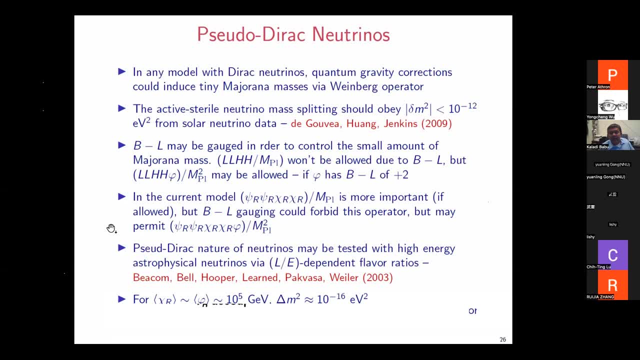 there are also experimental constraints from solar neutrinos. For example, the mass splitting between the active species and sterile species should be less than 10 to the minus 12 electron volts squared from solar data, And this whenever you have a Dirac neutrino there, once you include plant suppressed. 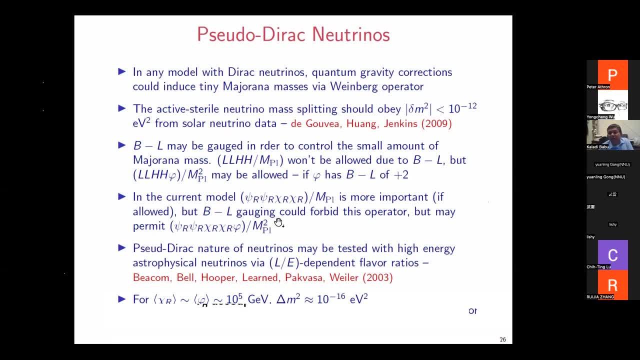 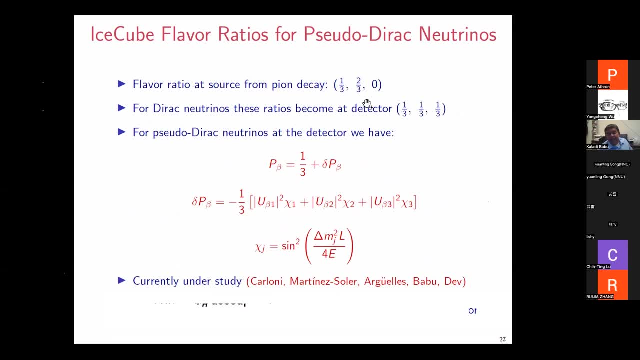 operator such as this. there is a good chance that it could be a pseudo Dirac for me, And this idea could be tested in very high energy neutrinos. In fact, we have an ongoing analysis with the Harvard group where we are studying this. 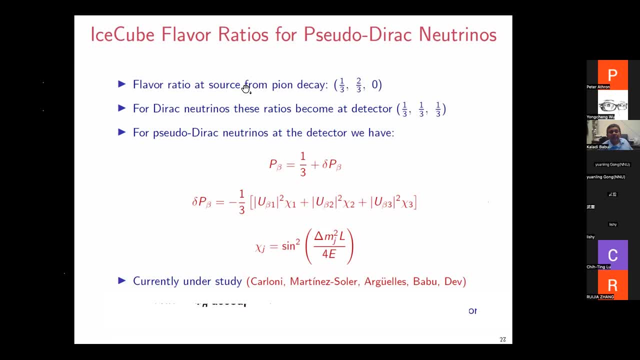 in more detail Here. what is shown here is that the traditional 1,, 2, 0 composition that is a pion decay produced of neutrino. it will have two neon neutrinos for every electron nutrient. That is just the flavor composition In the standard Dirac neutrino hypothesis. 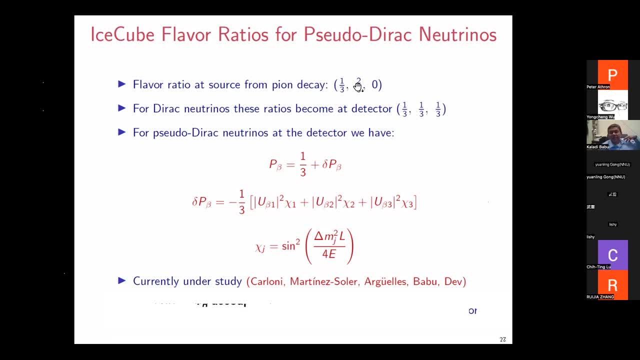 after oscillation. if they travel mega parsec of distances after the neutrino oscillation that takes place, they will become equal mixtures. However, if they are pseudo Dirac, for some range of this mass, splitting this one-third, one-third, one-third will deviate by some factor given by this expression. So 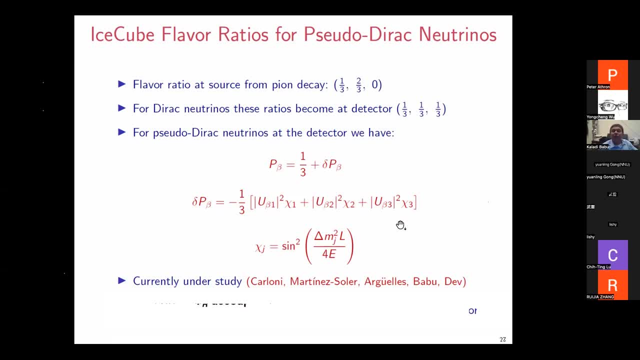 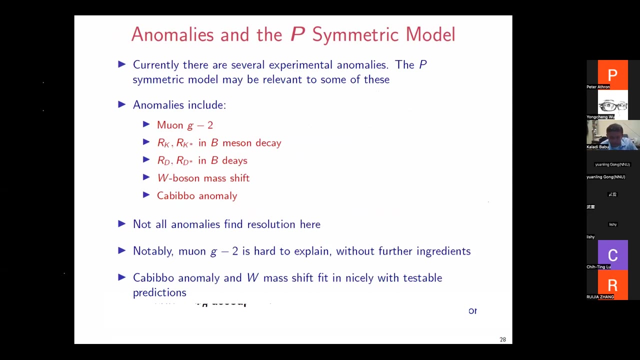 that is being currently under study And if you know the source of the ultra high energy neutrino, we can actually test the hypothesis that the neutrinos could be pseudo Dirac neutrinos. Okay, The last point. do I get another five minutes or so? 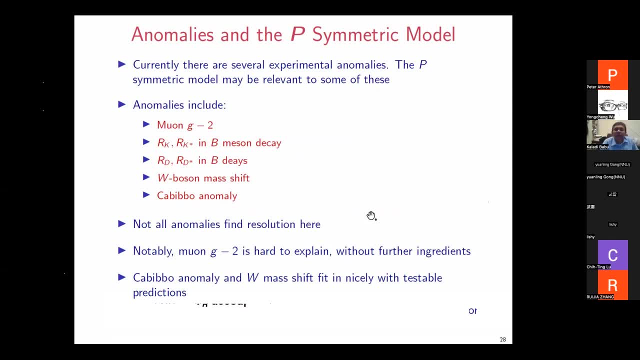 Yeah, Yeah, Please go ahead, No problem. Okay, Yeah, I wanted to say some relevant talk a little bit about the relevance to the experimental anomalies. As we all know, there are many anomalies. Some of them could be addressed in this context. There is the Mion G minus two. there are BDK. 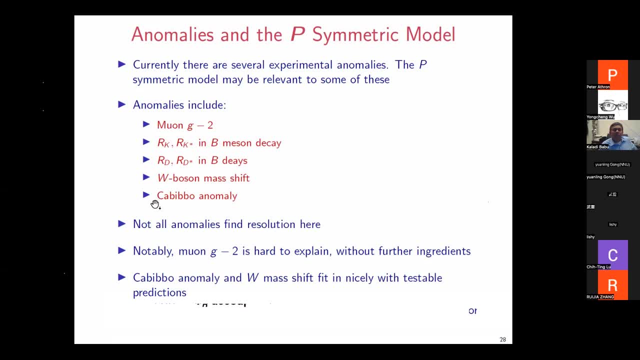 anomalies: RK, RD. there is a W, both on March shift. there's something called Khabibov anomaly. But okay, we have a setup. We cannot change the setup very, very much because the setup is constructed to solve the strong CP problem. If we add more, many more particles, the solution 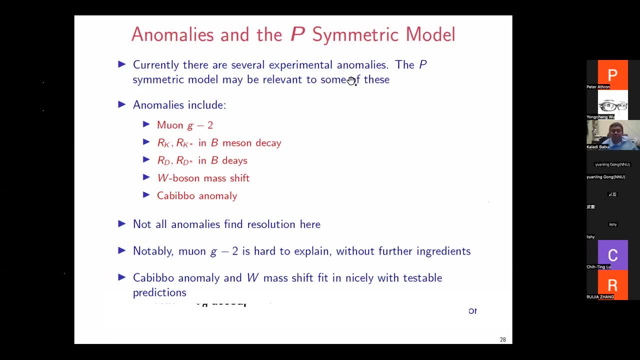 may be lost. So not all anomalies can be explained in this context, But there are some anomalies that we can try to solve. For example, we tried to explain the Mion G minus two anomalies. It is very hard to explain within this context. So what we found was that, similarly RK and RK star. 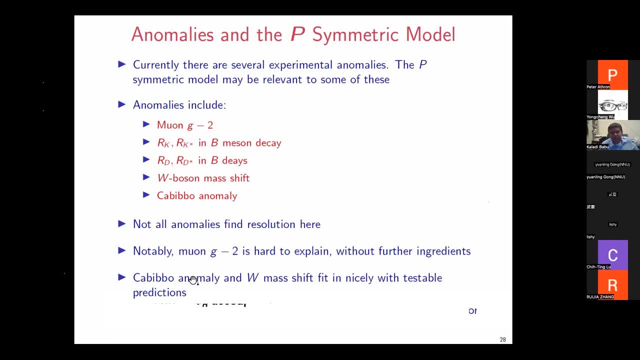 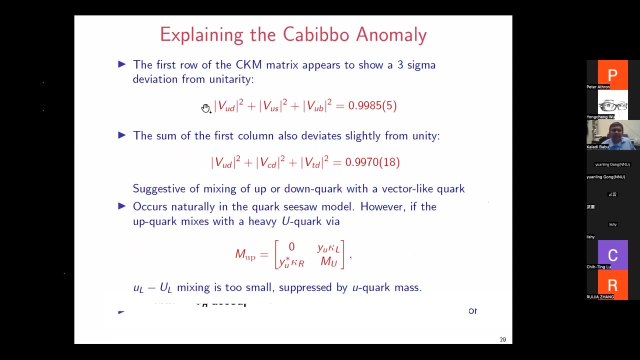 is very difficult to explain within this context. We found that the last two listed here- the shift in the W both on March and the so-called Khabibov anomaly- actually fit rather well within this model. And let me explain that. the Khabibov anomaly is the statement that, if you 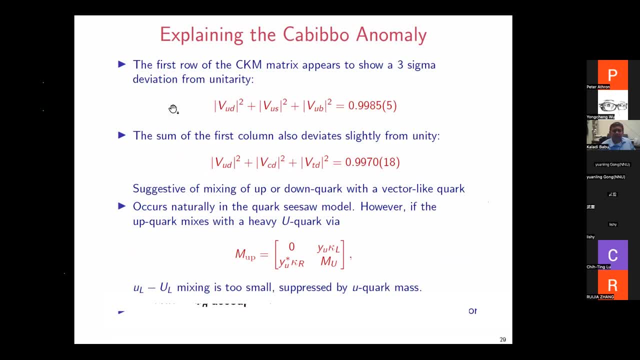 take the length of the first row of the CKM matrix, it doesn't quite add up to one. There is a three sigma discrepancy from one. So this could be an indication that there is some additional fermion which mixes with the up quark or the down quark And in fact 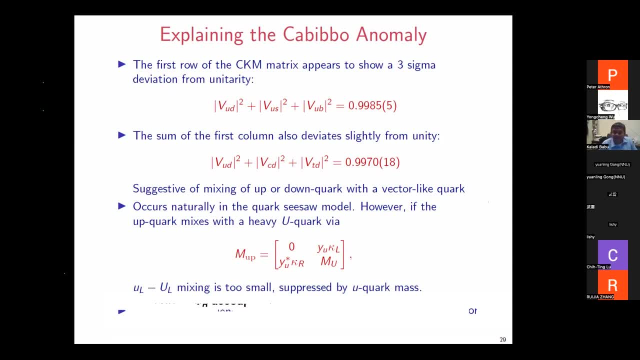 it happens naturally within the context that I was describing, because we needed the extra vector-like quark. It is also true for the first column. It doesn't quite add up to one, So together this is called the Khabibov anomaly. 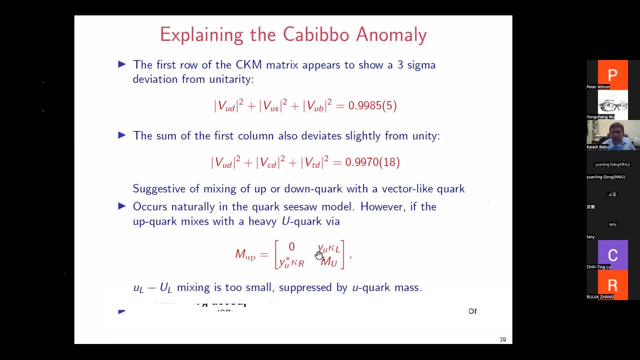 So if I take, for example, the up quark, the ordinary up quark mixed with some vector-like quark, actually we cannot explain that In the standard model. if you had the motivation for that, this could explain the anomaly. But because of parity, this coupling YU and this YU star are 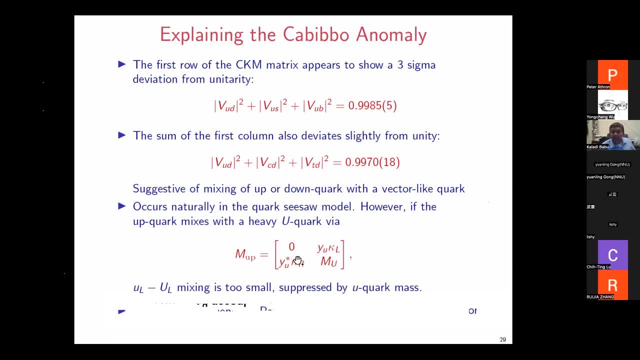 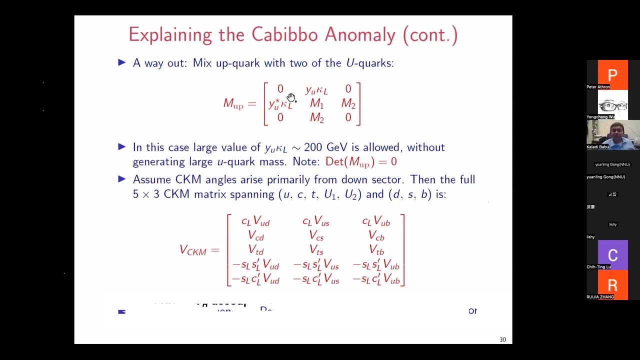 exactly the same because of parity. And then this mixing has to be extremely tiny to be proportional to the up quark. So this cannot explain, in a parity symmetric theory, the Khabibov anomaly. However, we have three flavors of this heavy quark, so I can mix up quark with two vector-like. 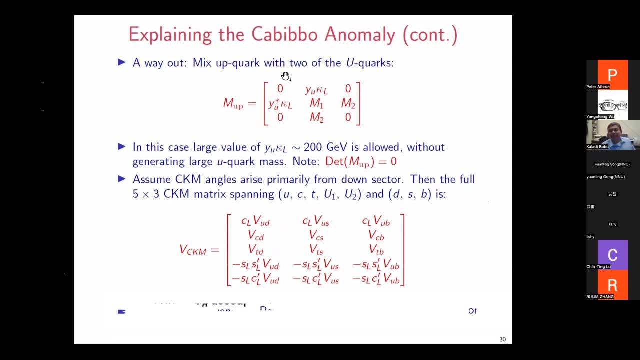 up quarks. That can be shown. It is a flavor structure where one up quark mixes with two heavy quarks And if I choose this kind of a pattern the determinant is zero, So it doesn't lead to any up quark mass. So I can get the up quark mass, But it can also be. 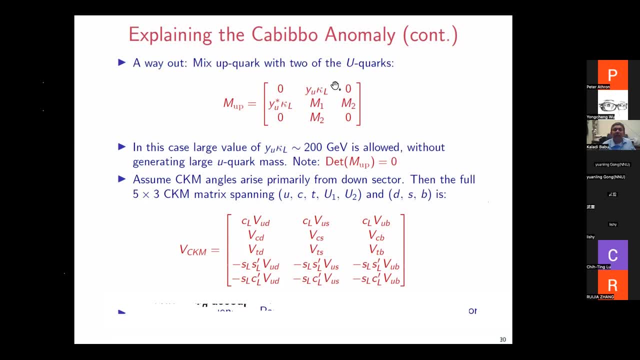 the mixing between the ordinary up quark and the vector-like quark is given by this ratio: yu kappa l over one of the heavy masses, And so that is actually a consistent way of explaining it. So for simplicity here I assume that the CKM mixing comes entirely from down quark. Then you go through this: 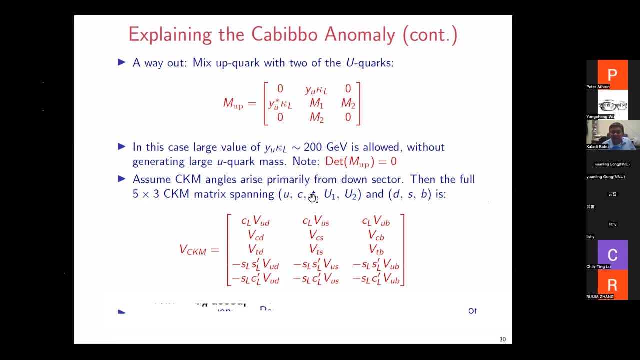 diagonalization and you will see that I have up charm and top and these two heavy quarks and ds and b and together they form a five by three CKM matrix and the first row and first column are modified and you don't. if you sum up the, this cl stands for the cosine of the mixing. 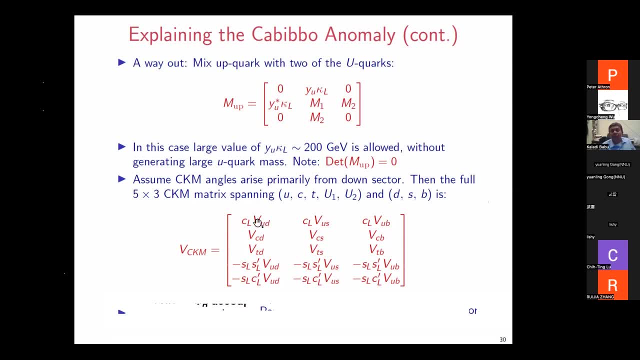 angle of the up quark with one of the vector-like points and you see that the sum of the the length of the first row is not long, no longer one. it is a sine squared of the mixing angle, and when the sine squared is about four per second. 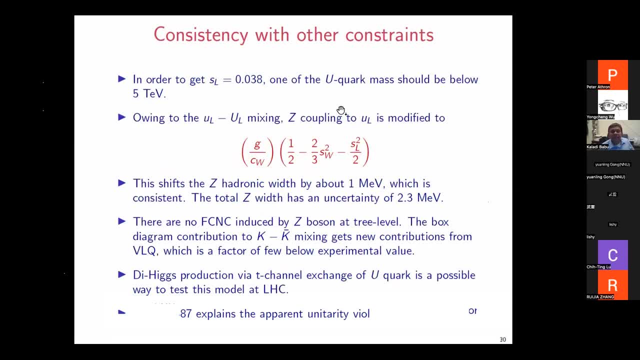 It can explain the Khabibov anomaly and this is consistent. yeah, when sine is 0.038, then anomaly can be explained and in order to get that to be four percent or so, the vector, like one of the vector-like quarks, have to have mass below 5t. So that's a prediction if Khabibov anomaly 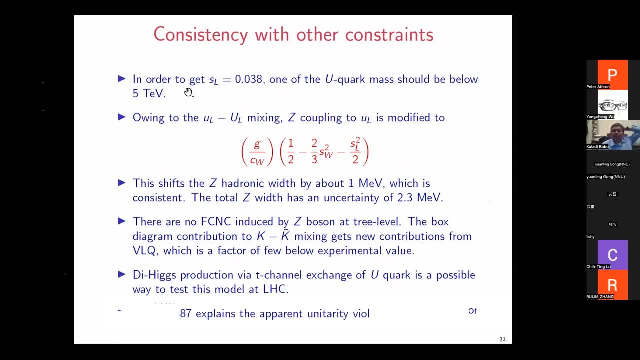 stays. within the context of this, one of the vector-like quarks have to be below 5t. and here I've shown that. uh you know, once uh quark mixes with vector-like up quark, it can change uh the z decay decay width into up quark. 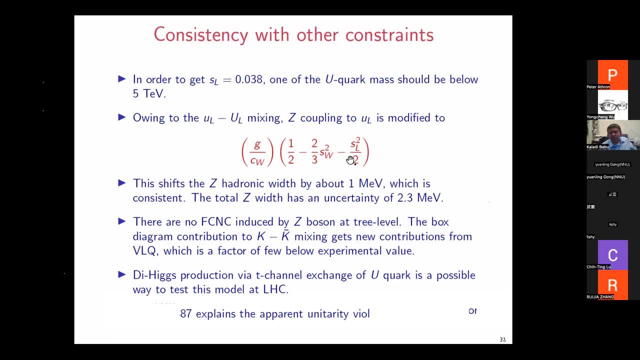 the hedronic z decay width. it will actually. the coupling is modified by this extra term. uh, but we check that the z width is. it shifts by one mev. current experimental limit on hedronic z width is about 2.3 mev, so it is consistent and there are no flavor changing. 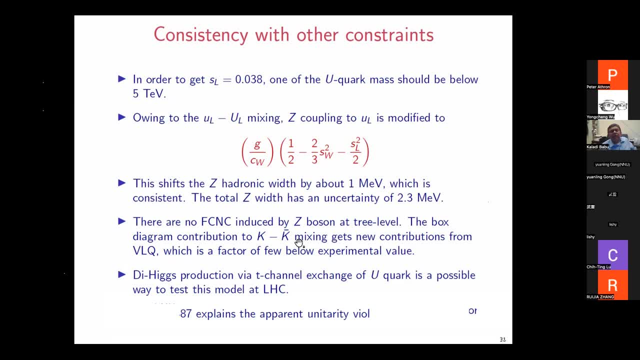 uh in flavor change induced by the zebos on a tree level and kk bar mixing. there are some contribution from loop level box diagrams but they are at order of magnitude below uh experimental limit. it's an interesting possibility that one can have dihix production through t-channel exchange of this vector-like point. this is 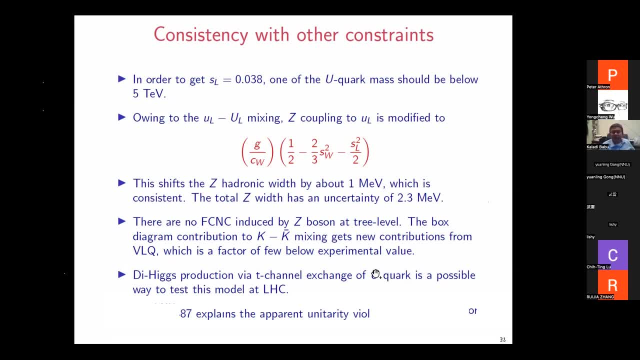 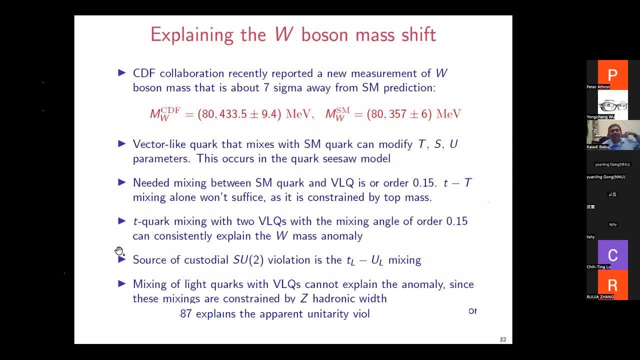 something. there have been some studies, but it is something that will be quite interesting to check in connection with the Khabibov anomaly. it has not been done, but we are thinking about it. and the last point is that we can also explain the w boson mass shift. as you all have heard, cdf recently reported: 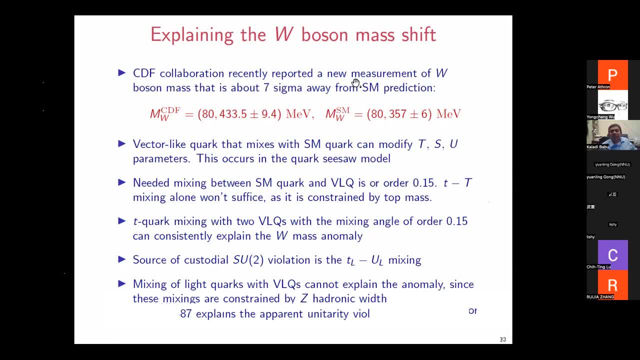 new measurement of w boson mass, which is seven sigma away from standard model prediction. if you have vector-like quarks it can modify the oblique electroweak precision parameter t, s and u. this occurs in the in this model, that's quark seesaw model. 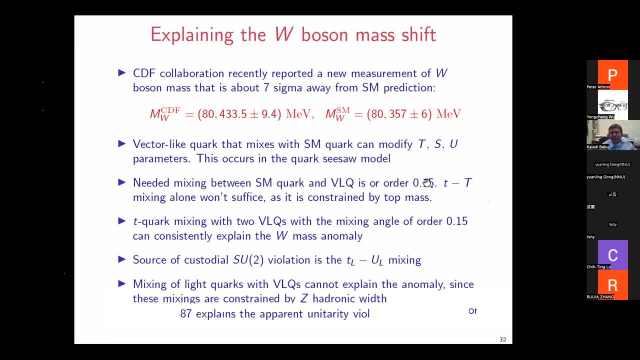 one might think that the top mixes with that top partner with them. if the mixing angle is a 0.15, that would be okay to explain the w mass shift. however, that is not consistent because then that would lead to very heavy top month because because of parity symmetry the top mass actually requires the mixing angle to 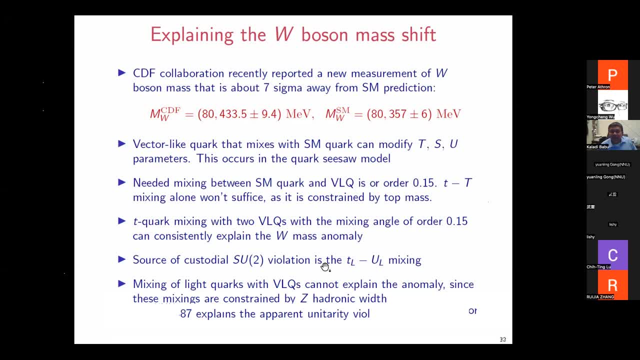 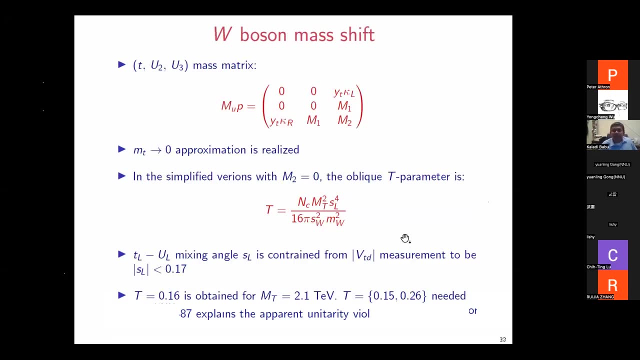 be much smaller than 0.15. uh, the source of the custodial su2 violation is a mixing of top left with this vector-like up quark. uh, this is su to double it. this is it to singlet. so this. this breaks, as you do, custodial symmetry. 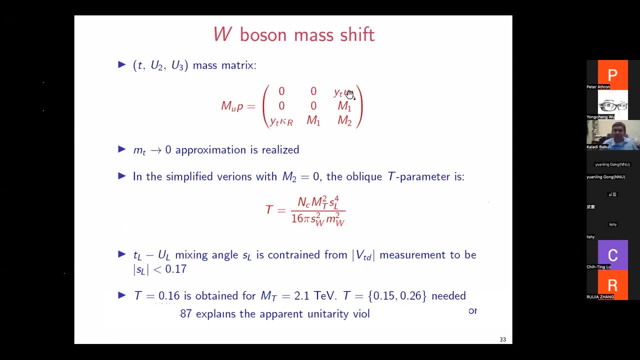 And so the trick is again: we have three different heavy quarks. If top mixes with two of these guys, then top mass is not a constraint And the t parameter is approximately given in some limit. It's a lengthier expression, but we have done it numerically. 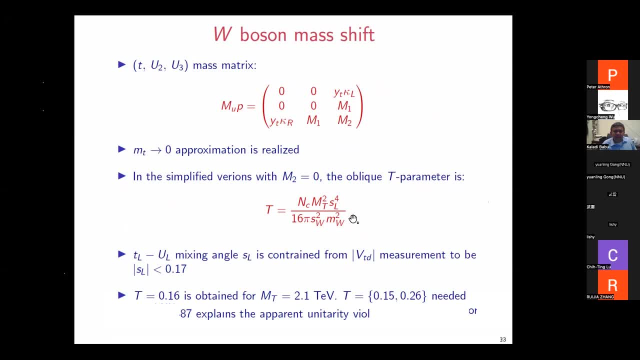 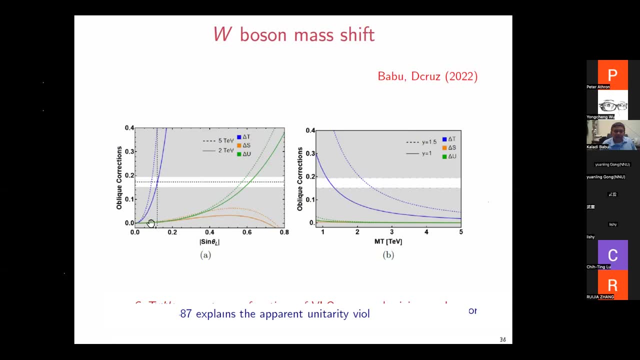 But in a simplified version. t parameter is given by this And this can explain the w boson mass shift. So in this plot the mixing angle of the top with the heavy top is plotted as a function of the oblique parameter t, s and u. 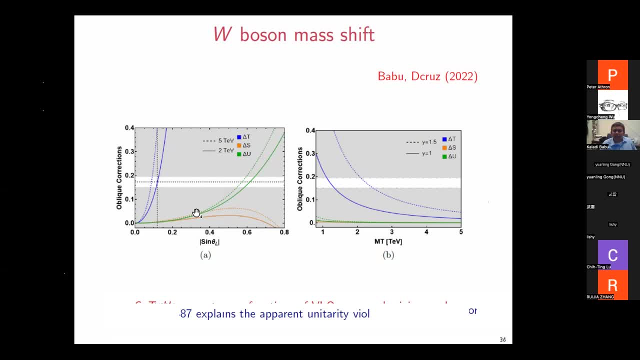 It turns out that the t parameter is a bigger contribution to the w mass, And here the mass of the vector-like top is plotted. And if you go below about 3 or 40, t v, the shift becomes too small. 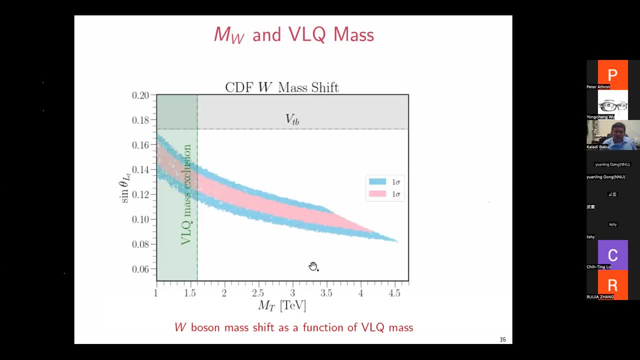 And that is shown here. The w boson mass shift has a function of the vector-like top and the mixing angle. The vector-like top is excluded below about 1.6, t v or so from direct searching. But you see that there is an allowed region when the mass is. 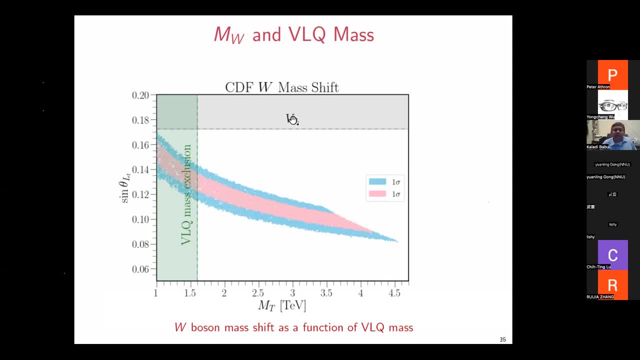 below, about 4, t v And then v t v. measurement determines that this mixing cannot be more than about 70, 0.17 or so. So there is an allowed region. There is an allowed region which is consistent with the Khabibov anomaly as well as the w. 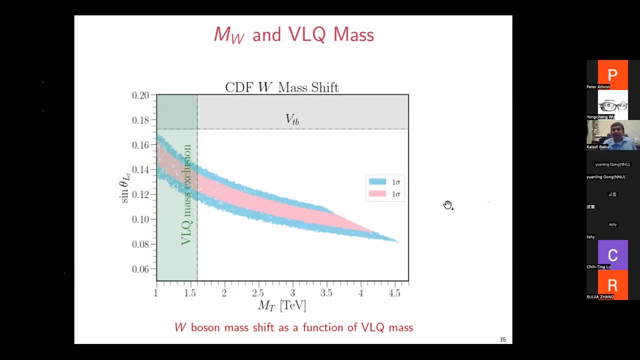 boson mass shift. So these are the strong CP solution itself doesn't tell us what the right-handed w scale is or the vector-like fermion scale, But if one of the anomalies is true and if it stays, then we can say that the right-handed w has. 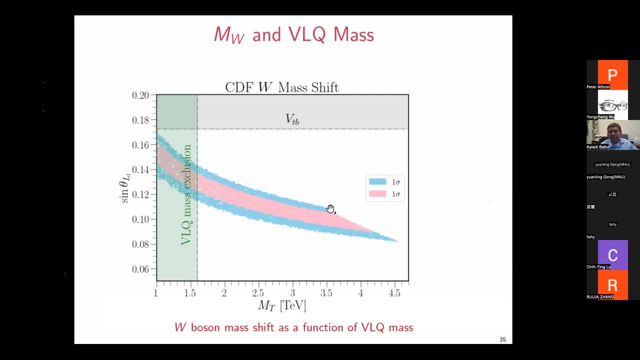 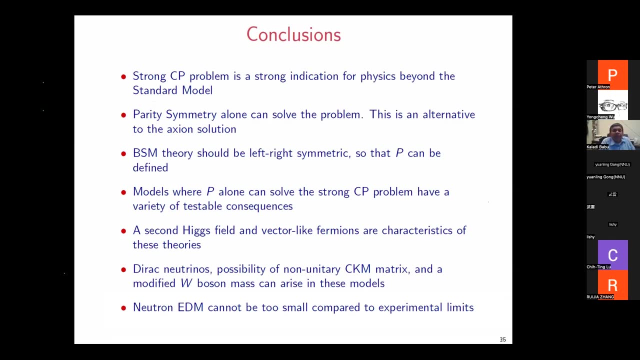 to be below about 10, t v And the masses of the vector-like fermion should be below 5, t v or so. So that brings to my conclusion. Strong CP problem is a strong indication of physics beyond the standard model. 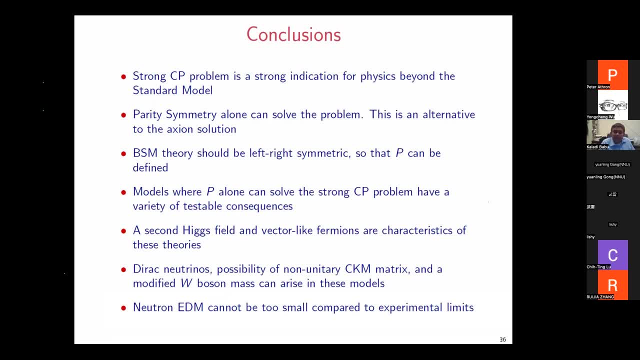 Parity, symmetric, alone, can solve the problem. This is an alternative to the axion solution. BSM theory should be left-right, symmetric so that parity can be defined. Models where parity alone can solve the strong CP problem have a variety of testable consequences. 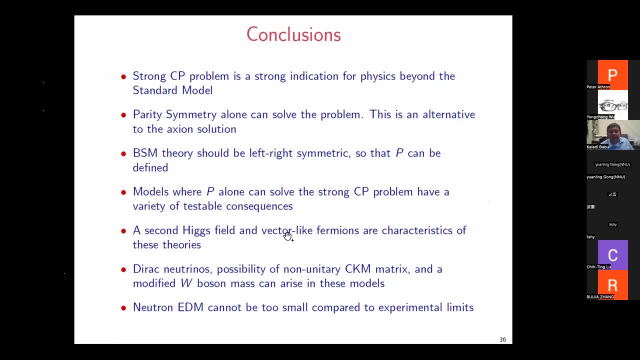 Generally speaking, a second Higgs field and vector-like fermions are characteristic. So we can say that the second Higgs field is a characteristic of this theorem. It allows for Dirac neutrinos, possibility of non-unitarity of CK matrix. modification of w boson mass. 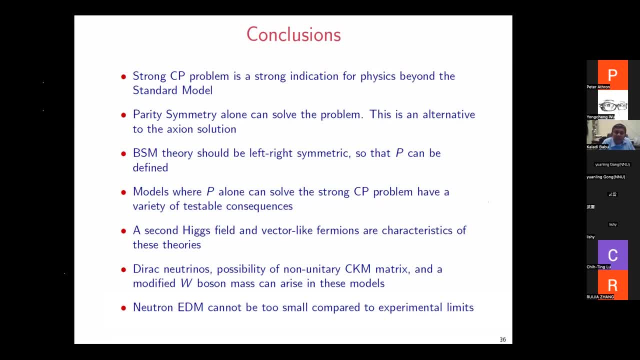 And finally, because this solution does not set theta bar to 0, like in the Pichet-Quinn solution, there is an induced value of theta bar that could contribute to measurable value of the neutron lactotipone. So future experiments can possibly tell us. 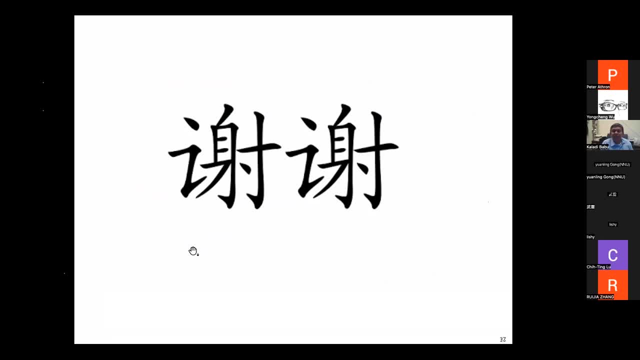 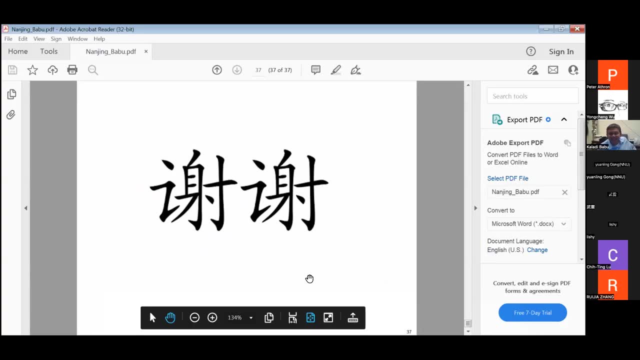 that there is an induced value of theta bar that could contribute to the non-unitarity of the neutron lactotipone. Thank you all very much for your attention. Yeah, thank you. Thank you for this nice talk. So we can have several questions. 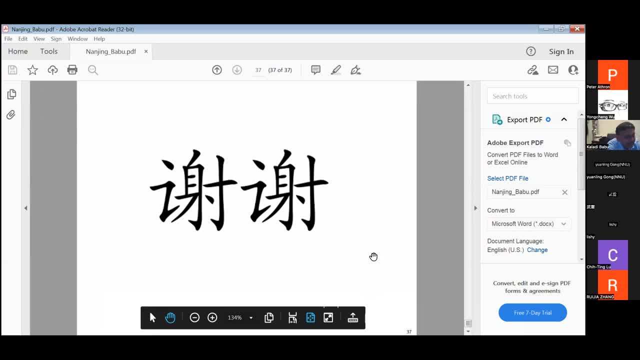 So if you have questions, you can unmute yourself to ask directly, or you can send a message in the chat box. So I see that there are some chat boxes, Oh, OK. yeah, That is about the slides. Yeah, I'll be sending Yangcheng the slides, not the talk. 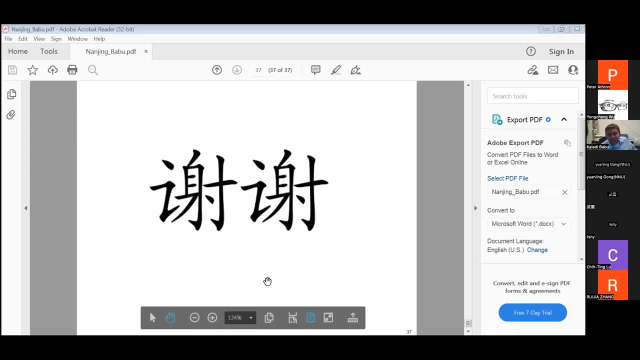 Yeah, thank you. Yeah, So I have a question about Dirac. You mentioned that it's hard to explain the muon g minus 2 in this model, So can you explain a little bit more like what's the difficulty there? 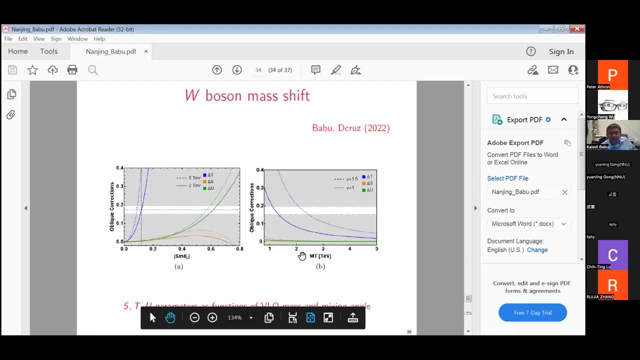 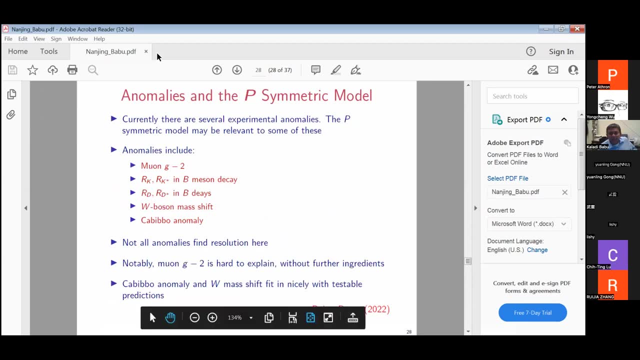 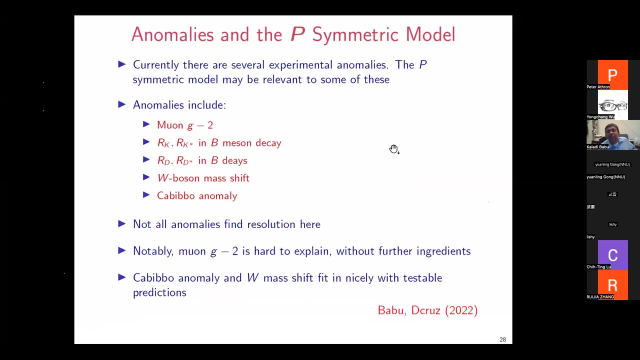 Yeah, sure, Yeah, among these anomalies, the muon g minus 2,. what happens is that there are experimental limits on the masses of right-handed v and right-handed w. The right-handed v should be greater than about 5 Tv from direct LHC constraint and right-handed w should be 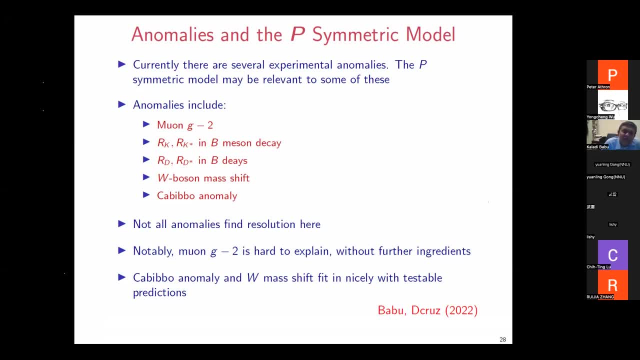 greater than about 14.. So if you have any loop correction which includes the right-handed w or right-handed z, it becomes too small. It is just a power suppressed by the experimental limit on right-handed w and right-handed z. So the best hope is to have a scalar interaction. 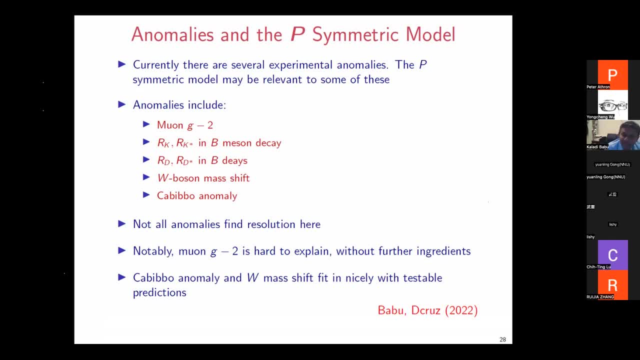 So, because the scalar factor is so simple, all we have is a standard model here. OK, So we have a single Higgs and a singlet scalar, which is the remnant of the SU2R break. So we looked at diagrams- one-loop diagrams. 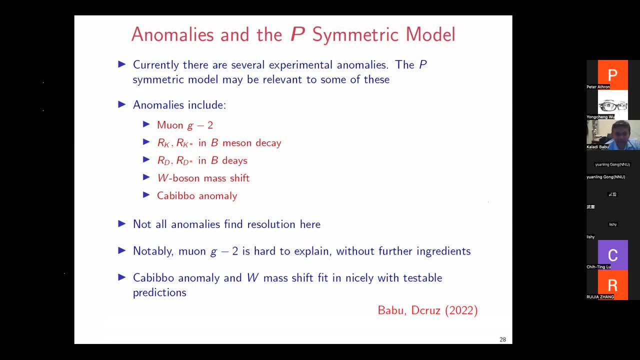 where the left-handed Higgs doublet mixes with the right-handed Higgs, the leftover Higgs field And the parity symmetry tells us that the relevant couplings are proportional to the muon mass. So even when the muon g minus 2 is greater than the muon g, 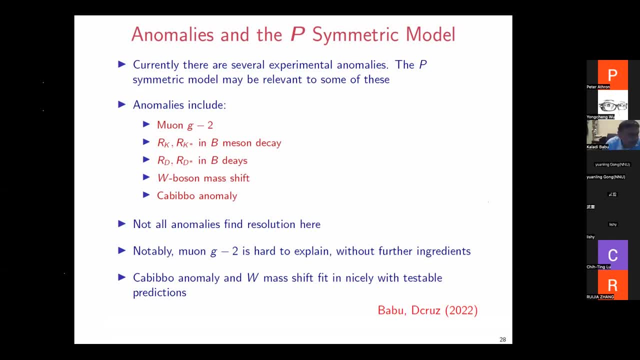 minus 2, there is a single Higgs field in the theory, Even when that single Higgs field is below 100 GV. even then the muon g minus 2 comes out to be one order magnitude below what is needed. So this is unlike the standard left-right symmetry. 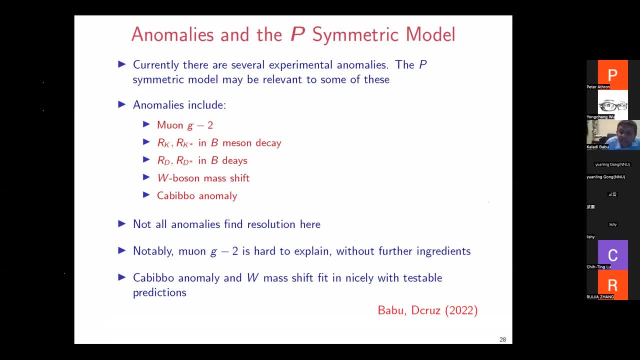 There are many new particles You can have, for example double char scalars coupling to muon. They can contribute to that. Here the minimality of the Higgs factor forces the muon g minus 2 to be rather suppressed. 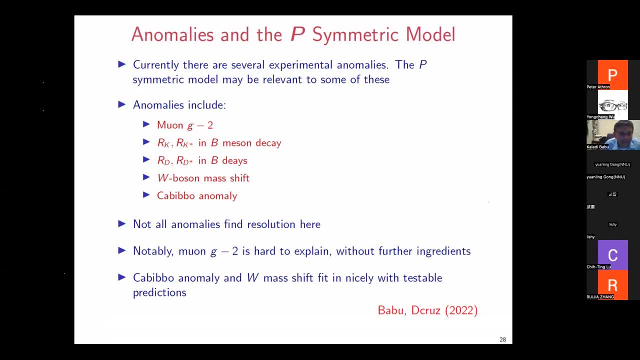 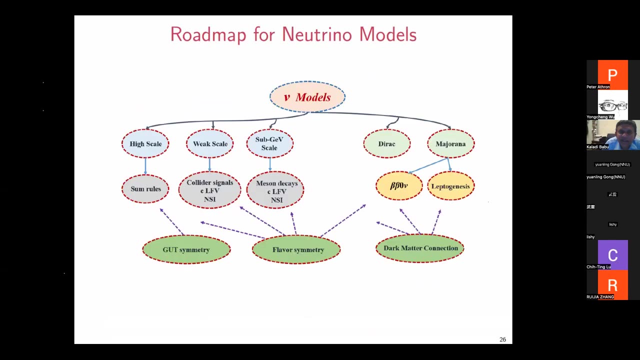 OK, OK, good. And I have another question about, like you mentioned, like in the model, you calculated the one-loop question to the theta parameter And at one-loop level, all this, each diagram itself, becomes 0.. 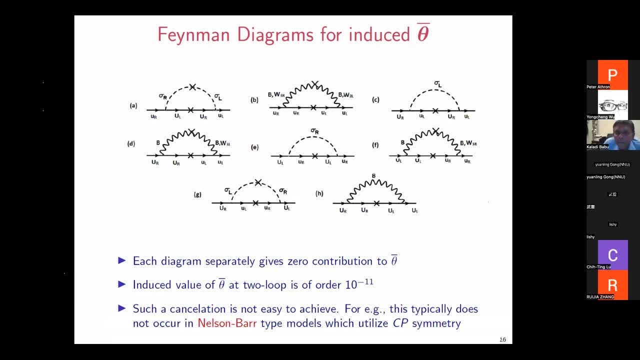 So is there like a, Is there like an explanation for that, like a symmetry or something like that for this? Yeah, so what happens is that I think the symmetry is parity symmetry, Since parity symmetry is there at the fundamental level. 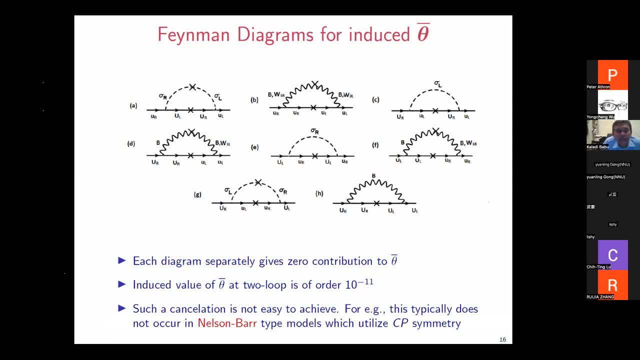 even when we evaluate these diagrams, we have to take any one of these diagrams right And we are interested in. you have to find the whole right quark mass matrix from this diagram and that is not enough. then i have to form a flavor invariant. 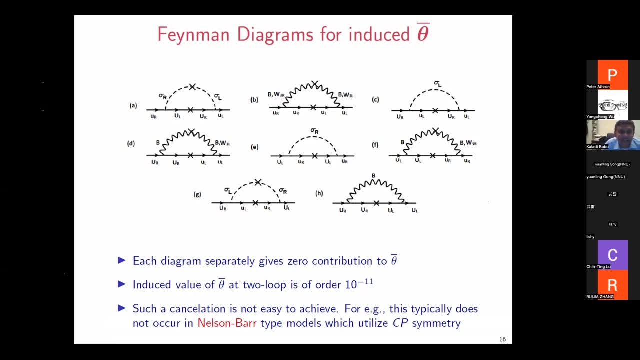 right, like because theta bar is a number, it's a flavor singlet, so i have to take, take a trace of some matrix. so what happens is that if i, if i have only trace of the up quark, you cover me, you cover coupling. then you can see that if i, on this one vertex i will put y, u and the other. 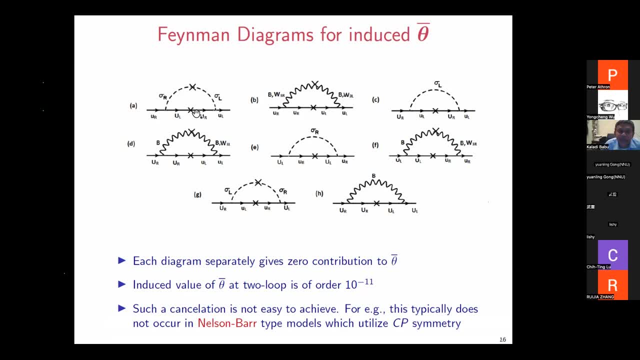 vertex, i will put y? u dagger and in between i will put the mass matrix for the heavy quark. but the heavy quark mass matrix is hermitian. why so? i have a trace of y? u dagger, m? u y u. okay, so that is real and because of that it is the the reason. reason for each of them separately: 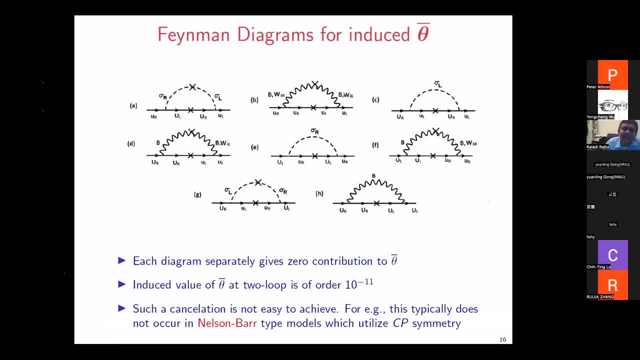 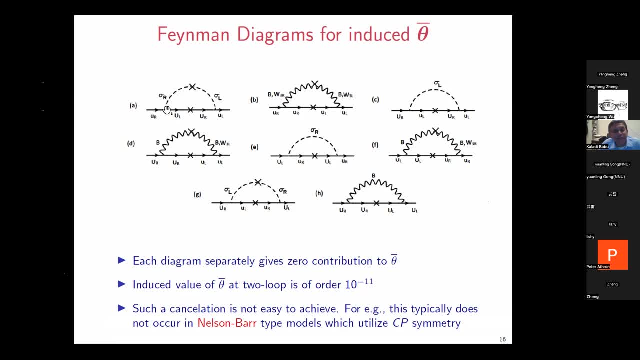 so if i compute the up quark mass matrix, i should bring in some down quark inside the loop and that's not there at the one. it does exist at a higher loop. okay, so that you will have some mismatch between different yukawa coupling, different yukawa coupling matrices. so yeah, 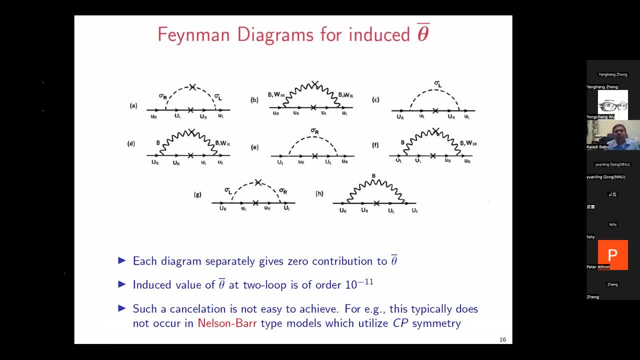 but the quick answer is that if you evaluate these diagrams and then take the trace the, the trace of the yukawa coupling matrix, and then take the trace of the yukawa coupling matrix, traces are all real, but one thing good, thank you. yeah, we have a question from audience, so 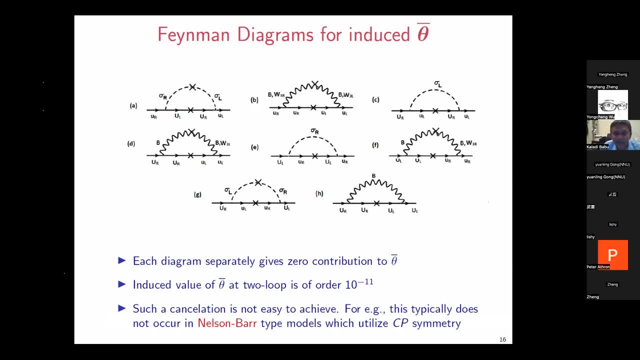 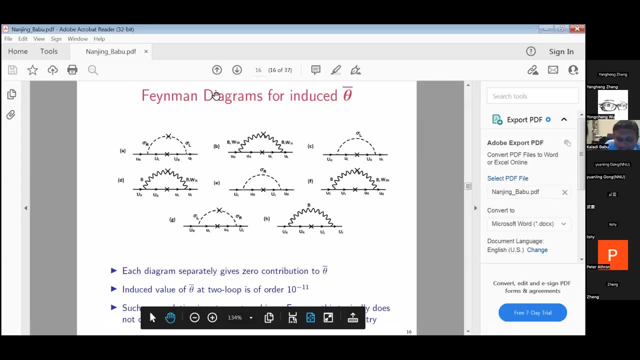 uh, yeah, please tell me to yourself. yeah, hi, hi, professor. uh, my nice and interesting talk, and i am a experimentalist so i'm not. i cannot follow all of those theoretical details, but uh, uh, it's interesting to know that your uh uh theory can explain this. 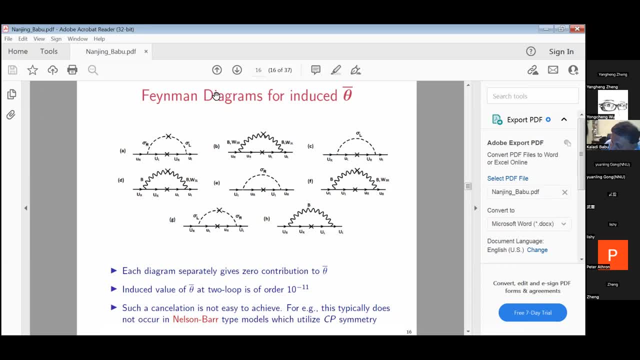 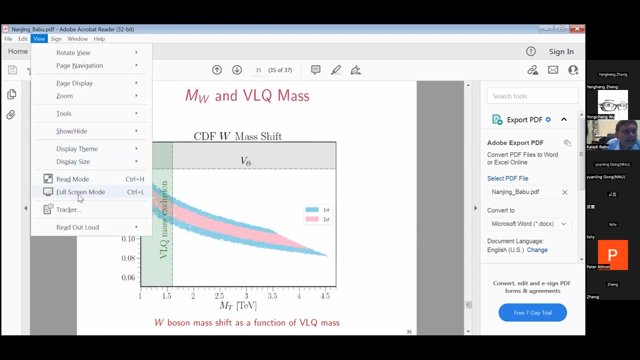 w mass and normal anomaly w mass and some other like the lactone flavor universality anomaly, essential. so my question is that: But can you use this measured WMAS from the CDF experiment to constrain your free parameters and give some kind of predictions on the other anomaly, like the hard D star or something? 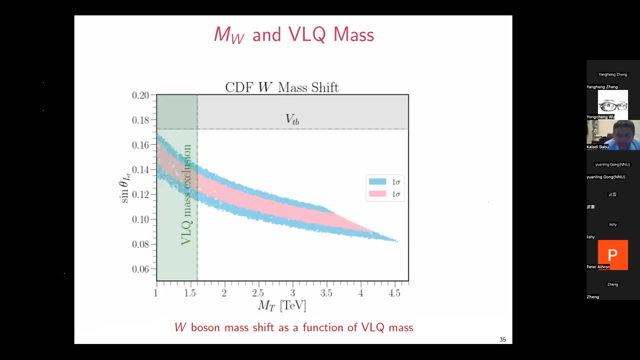 else? Yeah, thank you. Thank you, This is a very good question. Sorry that my talk was more theoretical, but I think it was still motivated by the experimental information that we have. So yeah, in answer to your question, this plot here: if you take the W boson mass measurement, 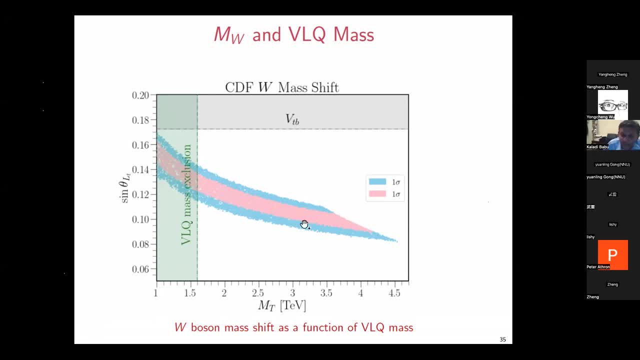 seriously and try to interpret it within this context. It requires the mixing to be. there is a mixing parameter, which is the top part, mixing with the vector-like particle that have to lie in this certain range between 0.16 and 0.1. 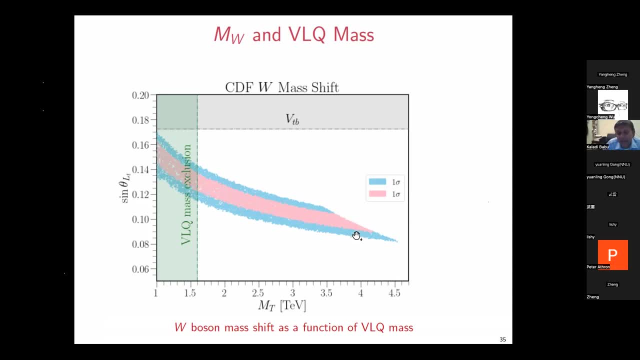 or so, And there is an upper limit on the mass of the vector-like part. It's about depending on whether you're allowing one sigma or two sigma. I think it can go up to about four TV So right, So the statement is that one sigma, two sigma. 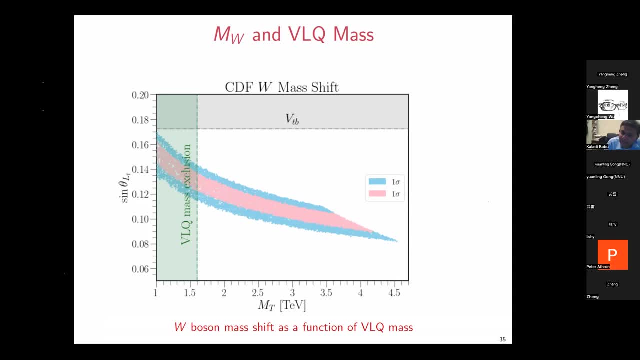 Right. So one of the vector-like quarks that mixes with top quark should have a mass below 14.. This is all we can say based on the W boson mass measurement. Now, if we combine it with the unitarity measurement of the first row of the CKM matrix, I think 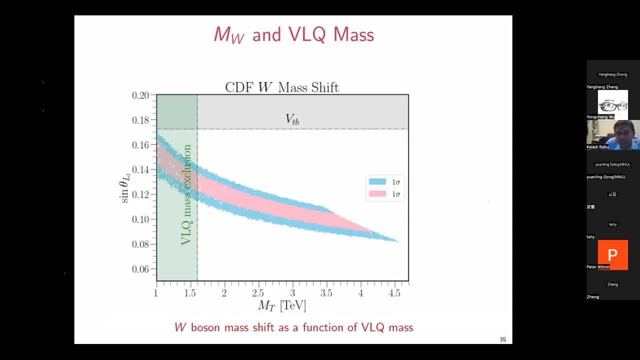 that also requires one of the vector-like quarks, A different vector-like quark which is something mixing with the down quark. It has to have a mass below about three TV And it's that mixing should be about 4%. The down quark mixing with with the vector-like down quark should be at the level of 4% in. 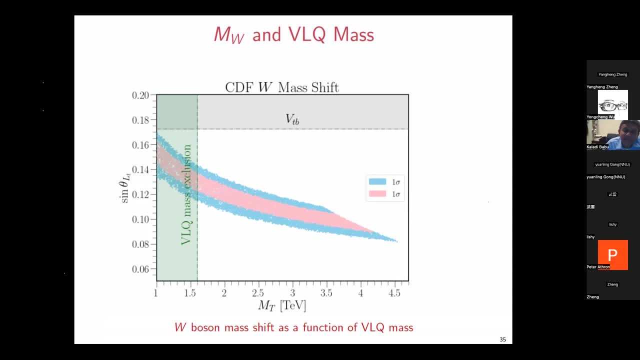 order to explain that anomaly Now. so we have these two pieces of pieces of information and we, unfortunately we are with this. Yeah, So the statement is that we cannot explain the BDK anomaly RK and RK star. There is just not enough enough room within the model to explain RK and RK star. 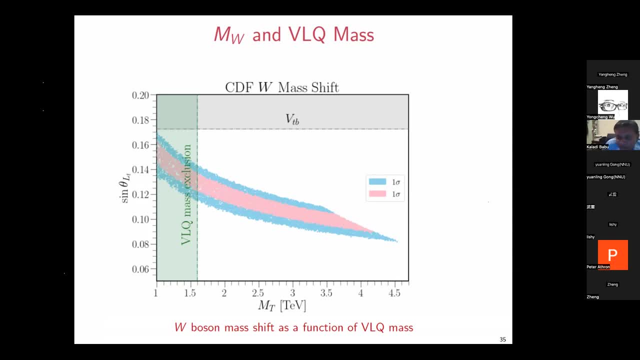 So, yeah, that is unfortunate, but maybe, you know, we can introduce new ingredient. but the philosophy was that we have a minimal model, We stick with it and and explore what it it predicts. So, according to this Theory, if this theory is right, the RK RK star anomaly should, should disappear. 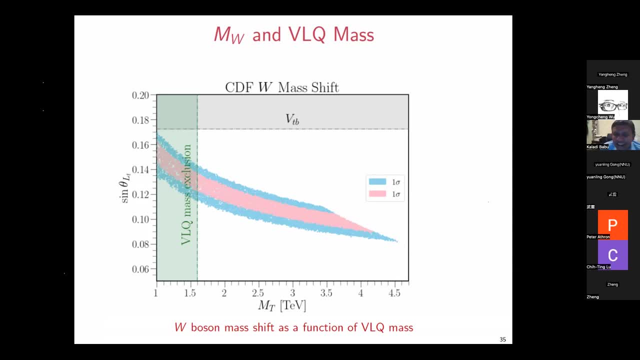 And similar to the muon g minus two anomaly should also disappear. Otherwise, if it is established with the, with the future experiment and also future lattice computation, then I think one has to go beyond the model that I presented here. Yeah, Okay. 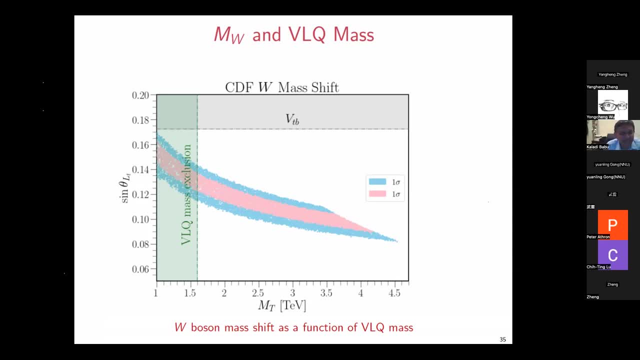 Thank you. Yes, Any other questions from all of you? No, Okay, Thank you. Thank you, I have a simple question. Go ahead. Yeah, Yes, Do you have a review paper, like a physical reports or something else? to summarize all, 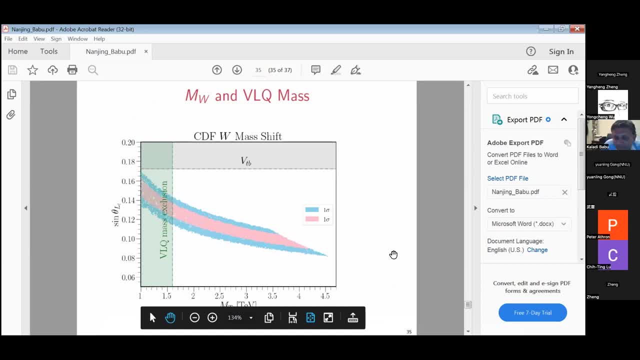 of these left right selection model? Okay, That's a very interesting question because you know, we have been thinking about it and we noticed that there are several review papers on on the axion solution to the strong CP, but very few actually, not at all, not, not at all. 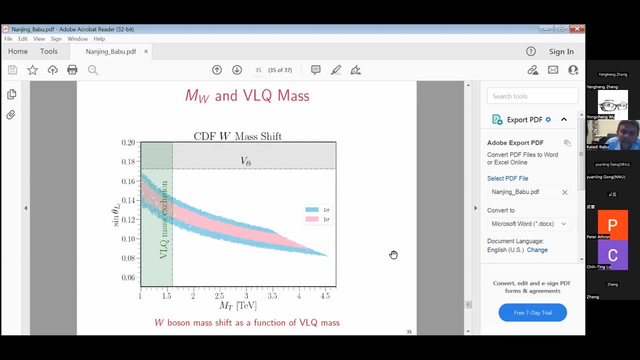 Any review paper for this parity solution or also CP, the CP solution to the strong CP problem. So in fact, yeah, unfortunately I'm not aware of any review paper, but I should say that in fact, I have a meeting with my collaborator. 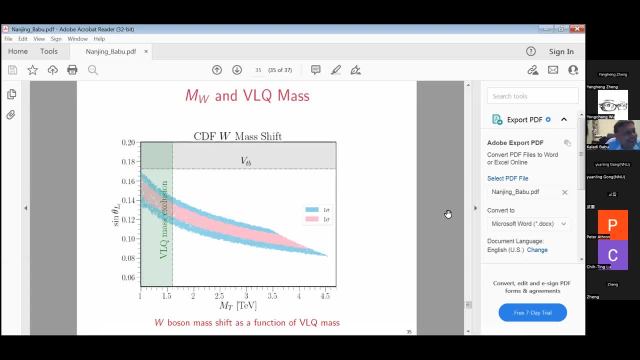 I'll be there, My collaborator, Ravi Mahapatra, tomorrow to be. I've been talking about writing a review paper, but it is in the works, Sorry. Another question: Does your vector-like quark contains the color degrees of freedom or? 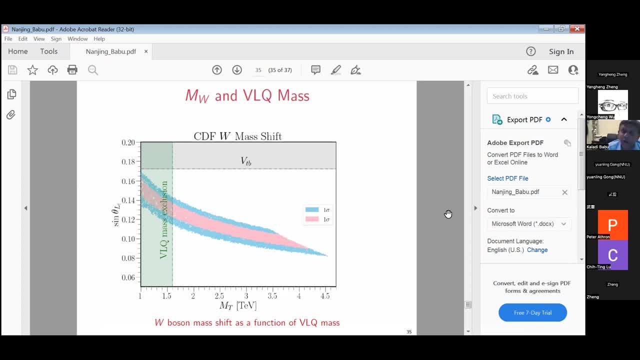 Yes, Yes, Yeah. So the vector-like quarks are exactly like ordinary quarks. They actually even mix with ordinary quarks. So they do have. they are exactly color triplet. It is vector-like in the following sense: They- I can write their masses- don't come from the Higgs interaction. 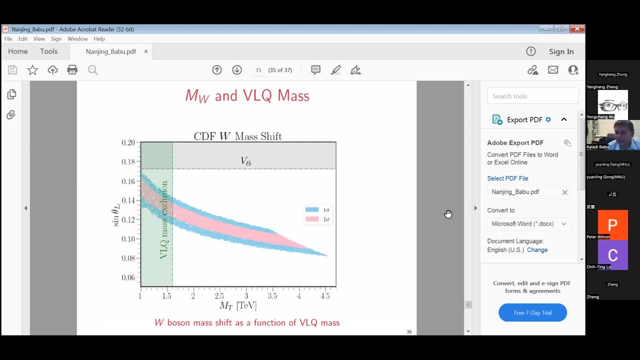 Their masses are you? just, you can write it down in the Lagrangian. So in principle, the mass could be much higher, much higher than the weak. weak interaction scale, like 100 GV. It can be 10 to the 10 GV if I want. 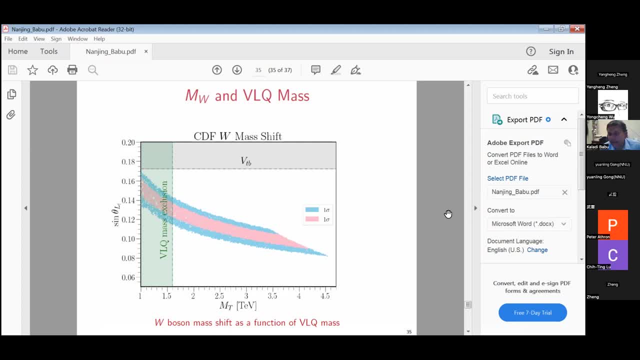 Because it's not Okay. Thank you. However, if you have something like this- a W mass is true, Then the experiment will tell us that at least some of the masses cannot be more than 4 GV or so. So in every respect, it is the color interactions- identical to the standard quarks. 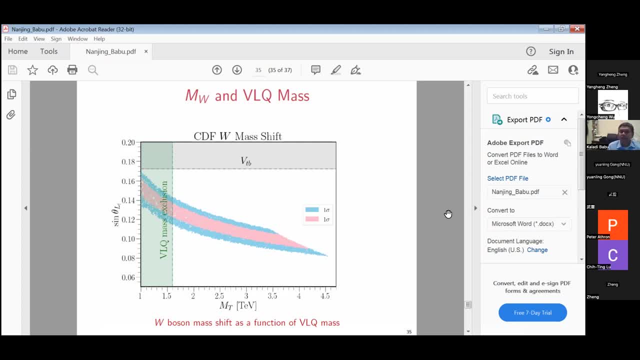 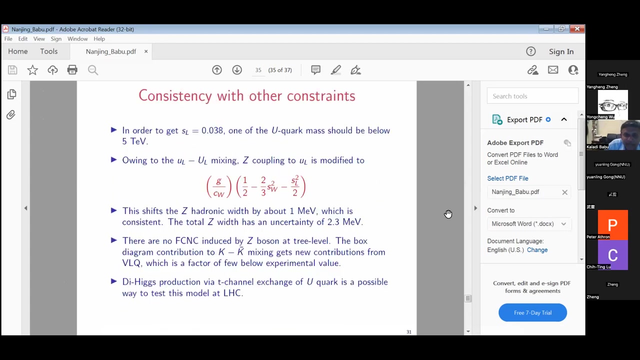 Their glue-on interactions are identical to ordinary quarks. Okay, The last stupid question: How do you wire break the parity spontaneously Just by the difference between Higgs, web or Right So the? I think I had it somewhere. Maybe I didn't export. 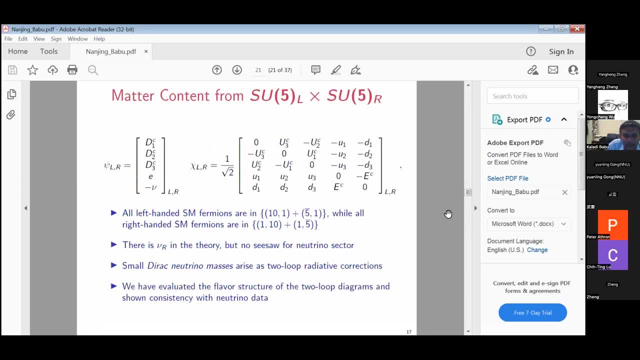 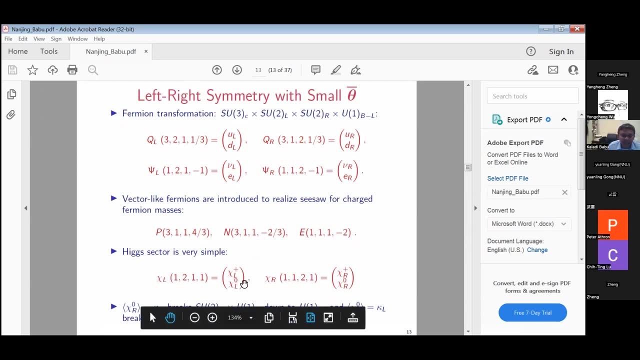 I did not write down the potential, but yeah, I can. I can expand on this for one minute, Yeah, So what happens? The? you have a. we have a left-handed Higgs field and a right-handed Higgs field. 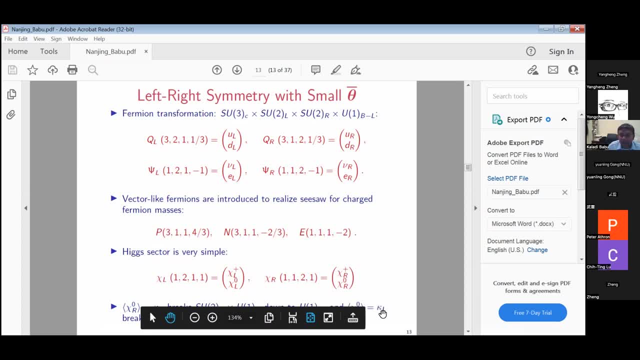 And the we have to somehow arrange for the vacuum expectation value of the left-handed Higgs field to be much smaller compared to the vacuum expectation value of the right-handed Higgs field. This can be done by writing a Higgs potential. If the Higgs potential is exactly parity- symmetric- 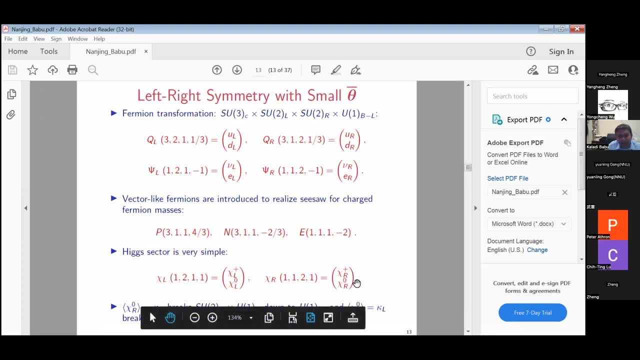 What happens is that the minimization will give right-handed Higgs getting a non-zero vacuum expectation value. The left-handed Higgs will get zero vacuum expectation value. This is acceptable. This is the idea that was developed by the Berkeley group. They say that if the left- right-handed symmetry breaking scale is around 10 to the 11 GV, 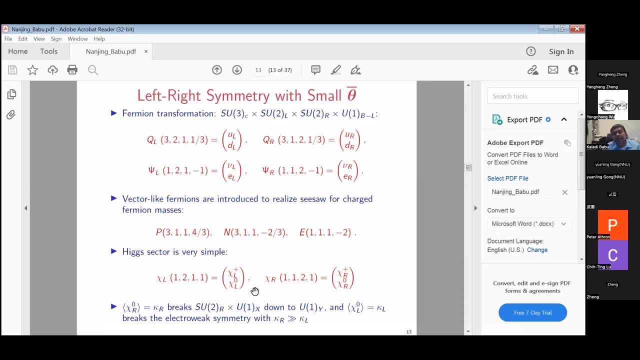 this is completely consistent with experimental data. The way we are adopting it is that we allow for a soft breaking of parity symmetry. That means that the mass term for the chi L and the mass term for the mass term for the chi L and chi R are slightly different. 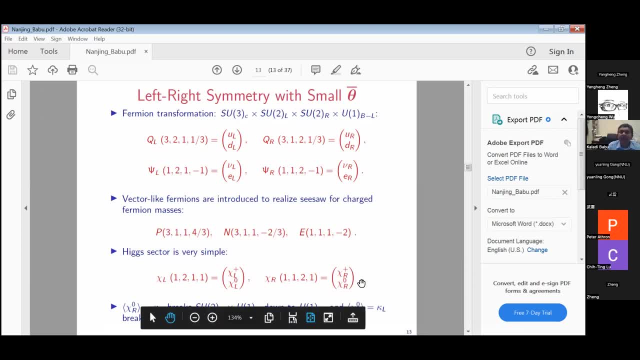 Then it will allow for the vacuum expectation values to be slightly different. Then it can be made completely consistent. We want to realize this hierarchy. This kappa R should be much higher compared to kappa L. Okay, But does this way of violating parity affect the Wafaa-Witten theorem? 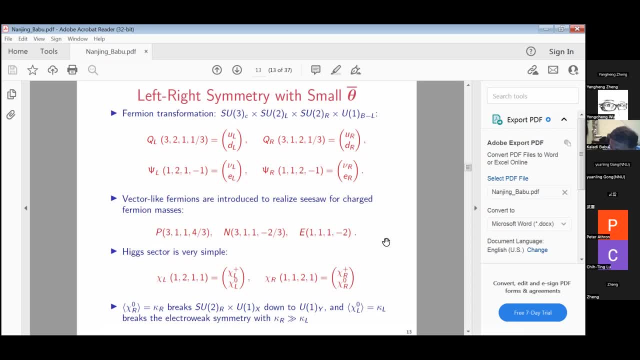 I mean the latter says this QCD, CP-conserving QCD- does not violate the ice beam symmetry. Will your parity violation influence the QCD sector, I'm wondering. Oh, I see That's an interesting question, Yeah. 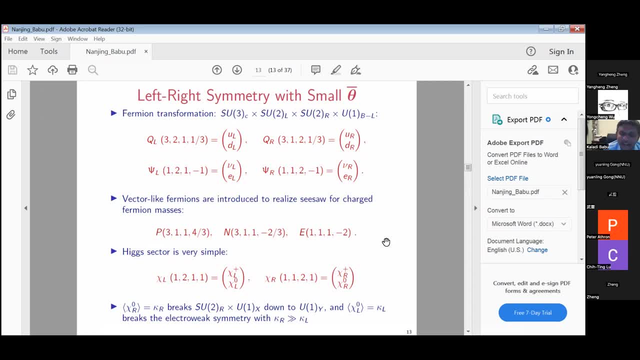 It's the Wafaa-Witten theorem that's applied to this case. It's an excellent question. I haven't thought about it, But I think a quick answer, which may not be exactly addressing your question, is that we have explicit. 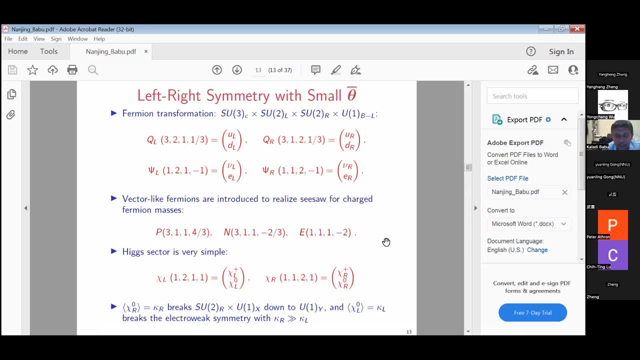 this will be the soft breaking is an explicit parity violation. So I'm not sure. in the presence of explicit parity violation, the Wafaa-Witten theorem is applicable. I have to look it up, I'm not sure. Okay, But this may not propagate into the strong interaction set. 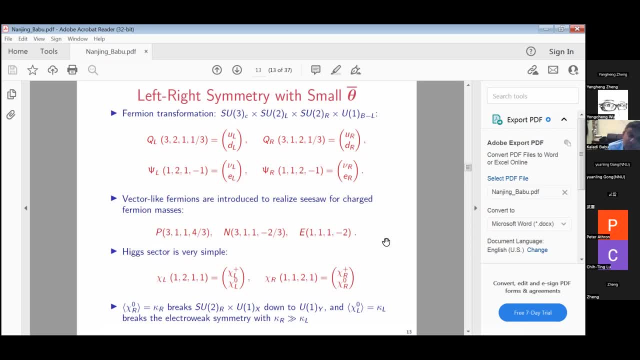 Yeah, except through the theta bar parameter. When this is affecting the parity invariant is affecting the theta bar parameter. So in that sense it is influencing the strong interaction sector, But it is I would say that it is affecting through perturbative method. 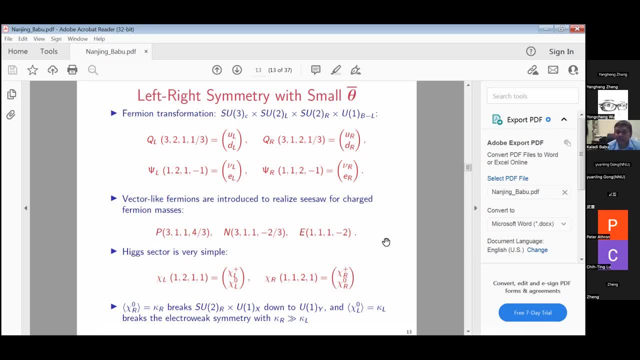 That is, we are inducing this theta bar perturbatively, not by non-perturbative interactions. Okay, Thank you very much. Thank you All right. Thank you, Yeah, So like it's already late there, So, 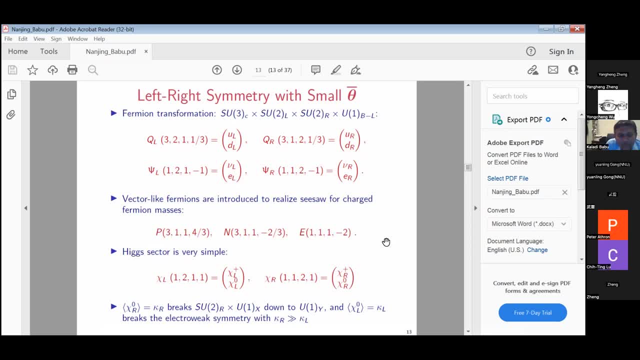 so I think it's yeah. let's thank the speaker again, So for this nice talk, and I hope we can have in-person meetings in the near future. Yeah, I hope so too. Thank you very much for thank you everyone for spending the early morning with me. 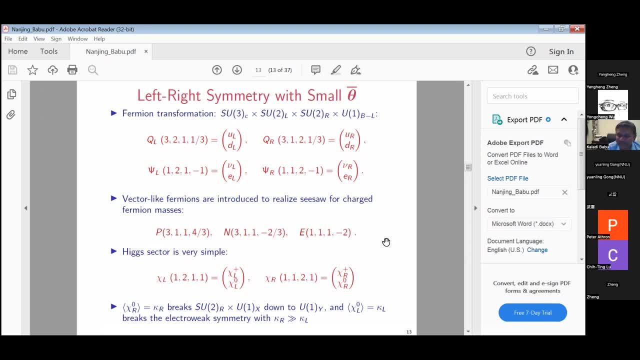 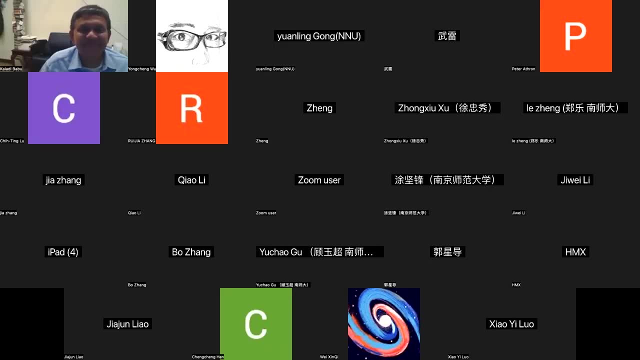